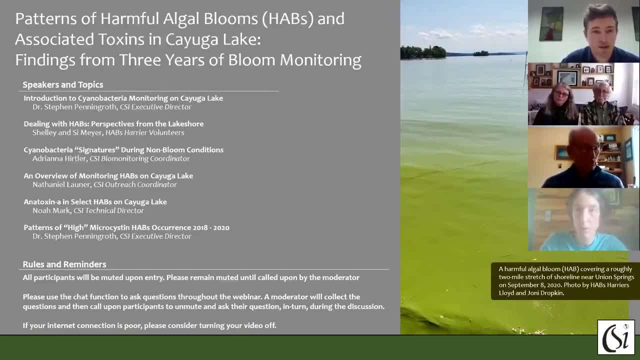 So just trying to keep it as organized as possible. We've got a lot of participants today, which is great. One final reminder is that if your internet connection is poor, please just consider turning your video off, and that should help tremendously. All right, and without further ado, I'll turn it over to Dr Steven Penningroth, Executive Director at the Community Science Institute, for the introduction to the webinar. 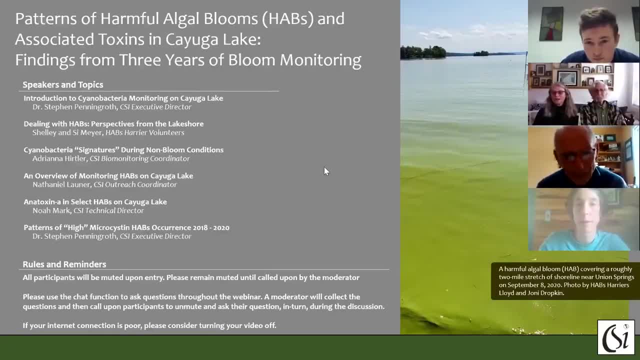 So I just pressed on share screen and it says this will stop now, And it says this will stop other screen sharing. Do you want to continue? So is that that's a yes? right, That's a yes? Yep, Okay, Thank you. 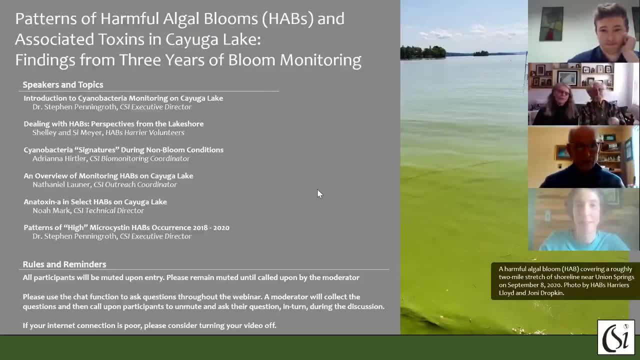 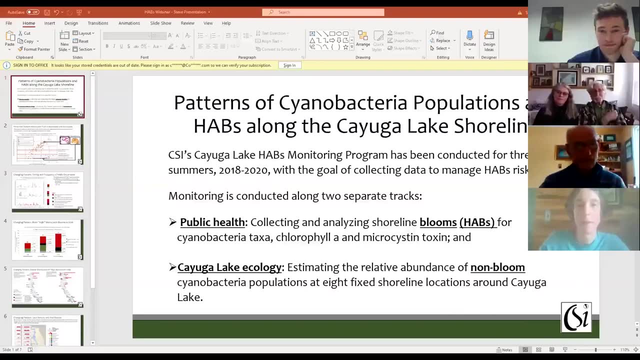 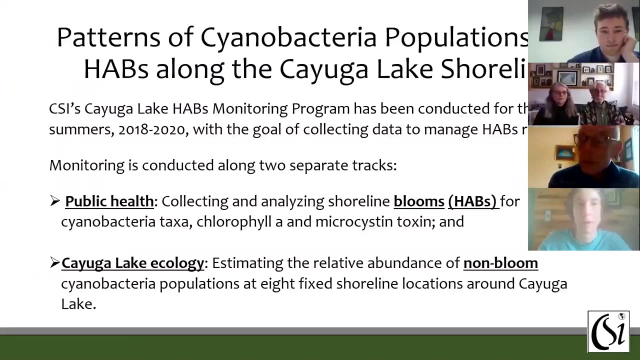 All right, And now? okay, here we go. Okay, here we go. So good afternoon everyone. My name is Steven Penningroth, I'm the Executive Director of the Community Science Institute And I'm really glad that you all can be here this afternoon. 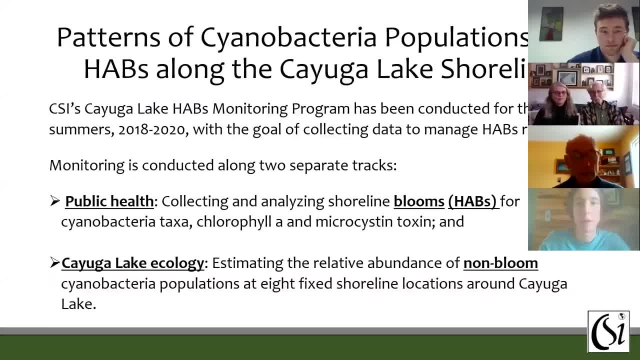 CSI, Community Science Institute, has been partnering with volunteers to monitor harmful algal blooms on Cayuga Lake for the past three years, And the goals of our monitoring program are twofold. One is to keep the public informed in near real time about where HABs are occurring on the Cayuga Lake shore. 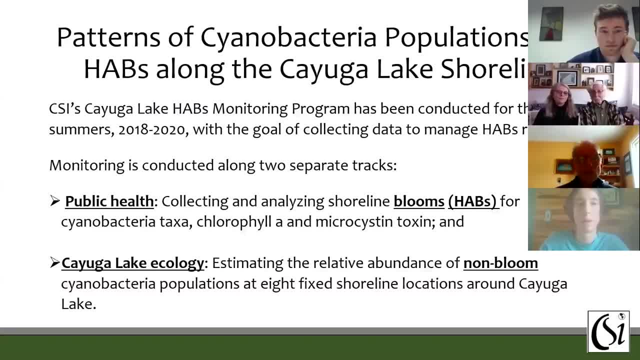 And the first one is to collect data about the property of HABs. The secondary goal is to track and monitor and document the activity of HABs in the area and their toxicity, And the second goal is to collect data that can reveal patterns. 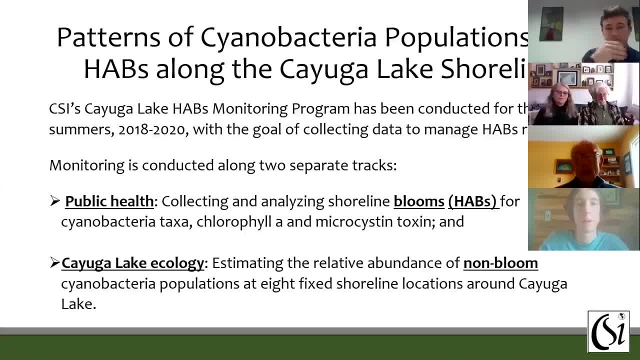 and help inform strategies for managing the risk from HABs over the long-term. So our HABs monitoring program operates along two separate tracks, And one track I'll call the public health track. Our 90-plus HABs Harrier volunteers patrol the shoreline and collect samples of blooms. 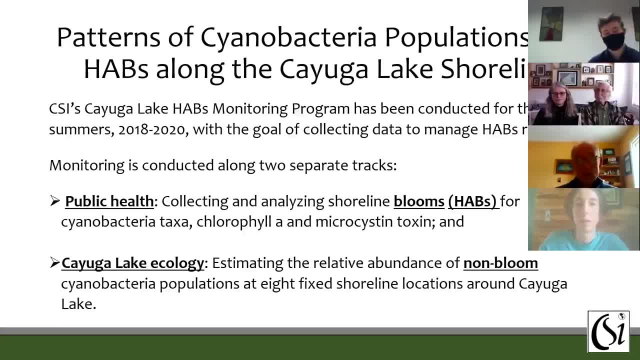 for analysis in the CSI lab. So that's our very large volunteer monitoring partnership with our Habs Harrier volunteers. And the second track is what I'll call the ecology track And that consists of CSI's biomonitoring coordinator conducting regular surveys of the populations. 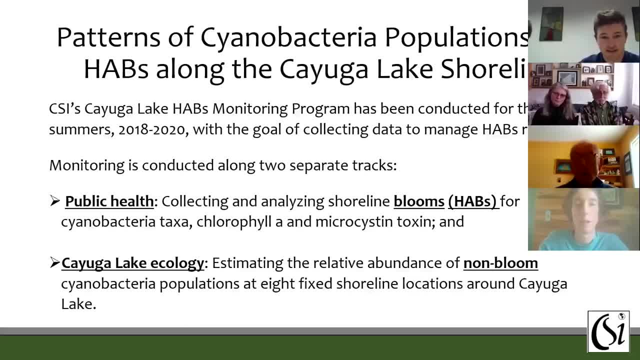 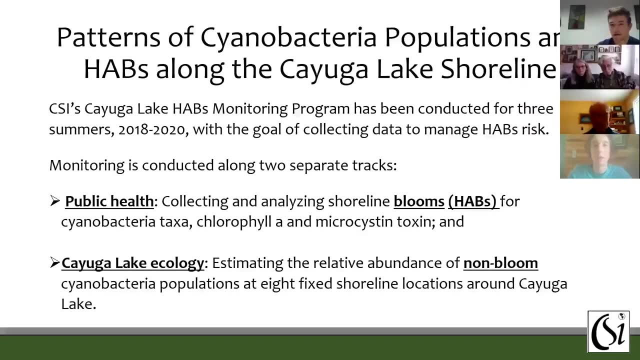 of several different types of cyanobacteria under non-bloom conditions at eight locations, eight fixed locations around Cayuga Lake. So our Habs monitoring program would not be possible without our many, many dedicated volunteers, And two of them will lead us off now. 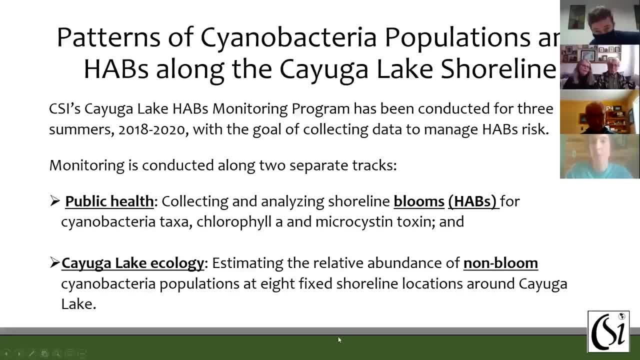 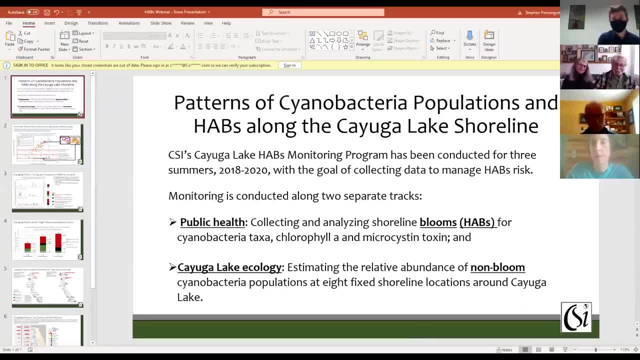 So I'll turn it over to you, Shelly and Sai. Well, we thank you. I'm Shelly And I'm Sai, And we do wanna thank CSI for including us in the presentation and, of course, for the important work that you're doing. 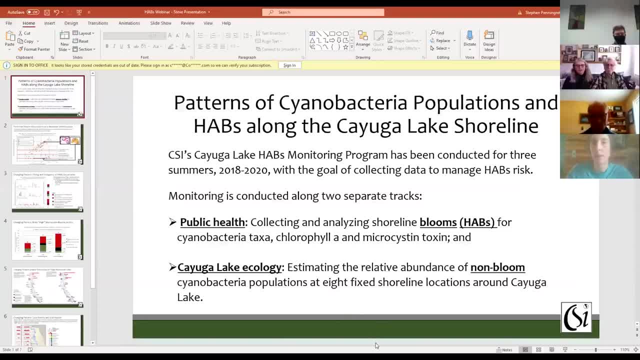 Our plan is that I'll talk a little bit about our location on the lake and then Shelly will walk you through a couple of the Habs we've been able to sample this year. So, if the gods are good, I can share a screen. 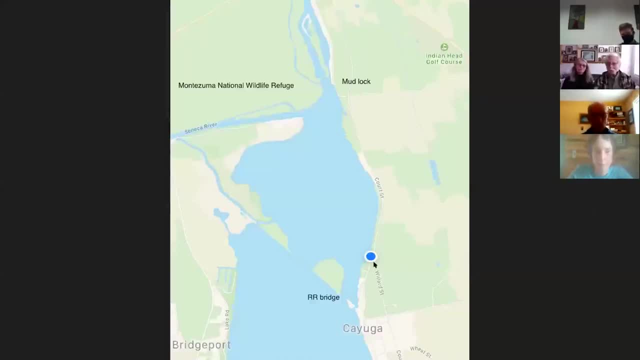 So this is where we're located on the water at the north end of the village. So this is where we're located on the water at the north end of the village of Cayuga. The zone that we monitor for CSI starts here at the railroad bridge. 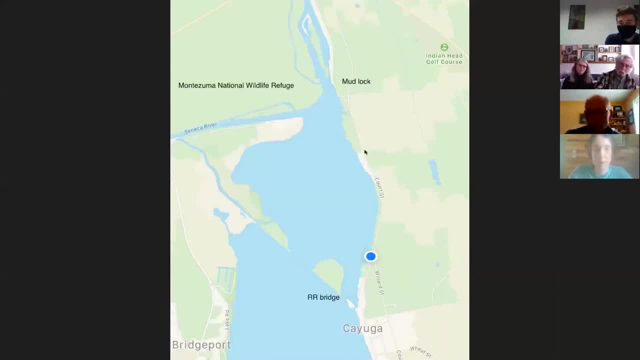 and goes up the eastern shore for a distance of about two miles up to Mudlock, where we connect to the canal system. You'll notice the proximity of Montezuma National Wildlife Refuge And you should also notice this chain of islands which makes this part of the lake really different. 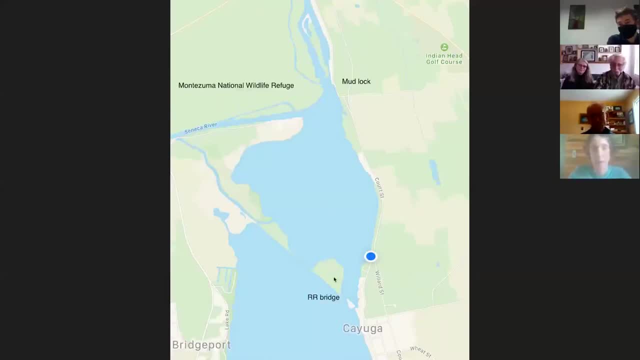 than the rest of the lake. It's quite sheltered And we'll also mention that it's quite shallow. I should say that this year we've also had another Hab Harrier who's been able to help us monitor the southern end of our zone. 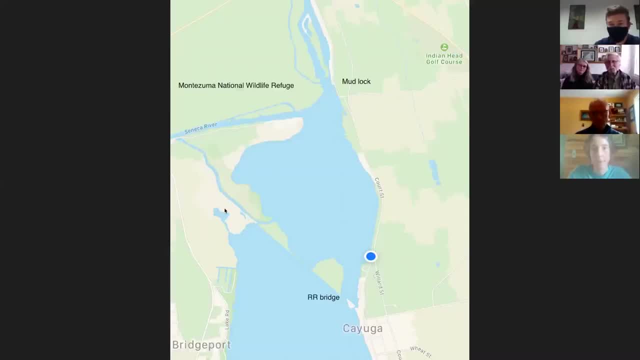 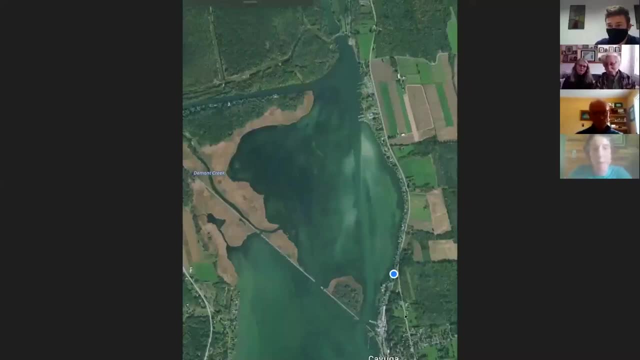 For reference. this is an Apple Maps satellite image. but what you can see along our zone there's a marina, a long string of private homes- The locals call them camps- A couple more marinas up to Mudlock. You can also see that, that part of the lake. 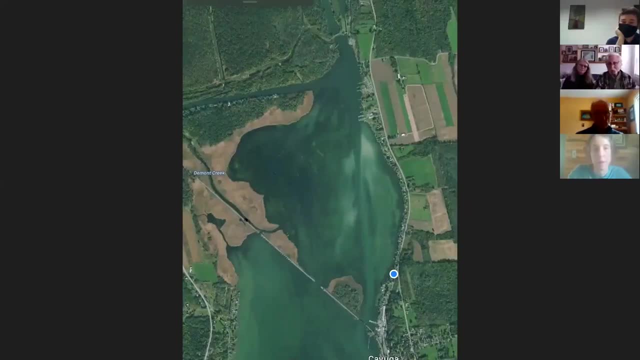 is entirely surrounded by marsh area. It really is quite pristine. The other thing I should mention about this image that I like is you can see the dramatic difference that that's the only part of this lake, or this part of the lake, has any depth at all. 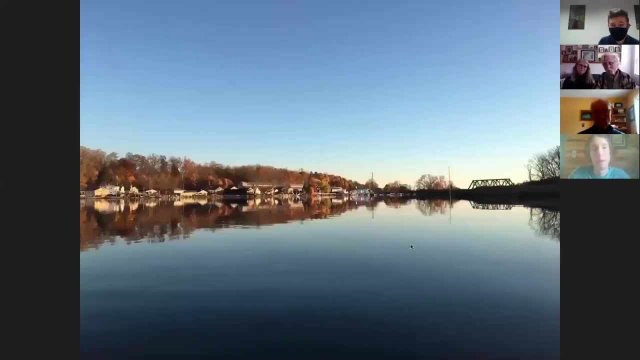 The rest of it is really quite shallow. Here's a water level image. You can see the railroad bridge, This one is Beacon Bay, Marina, and the beginning of this string of homes along the shoreline. I'll also point out that the water is remarkably calm. 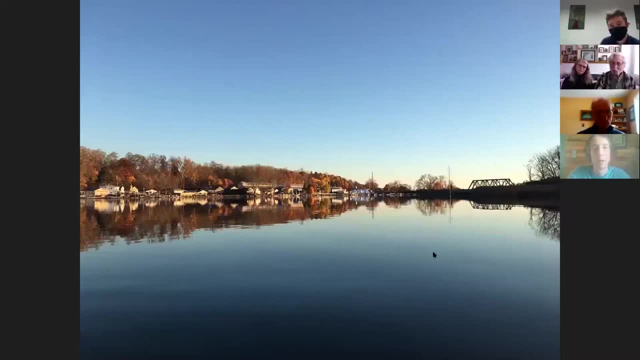 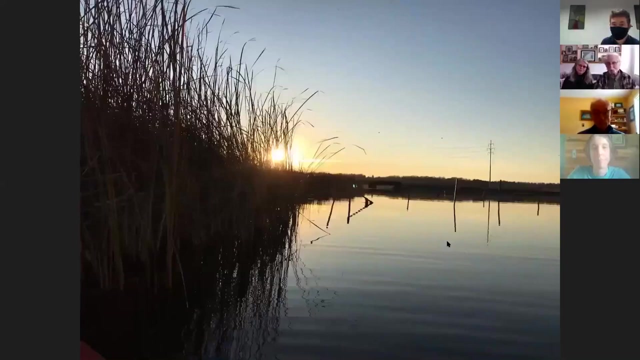 which is not so unusual. It's very nice for those of us who like to kayak. It's also very attractive to our algae blooms. Just for reference, the opposite shore. this is a piece of the island. You can see the marshland and further up. 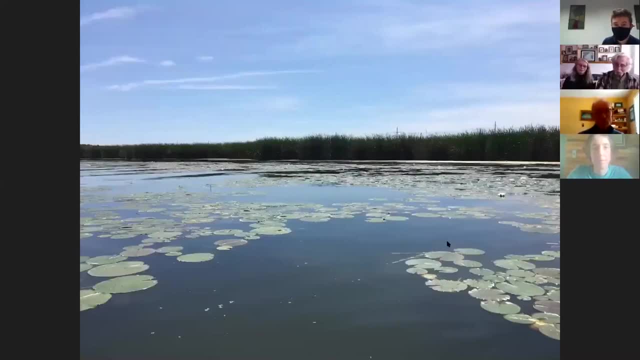 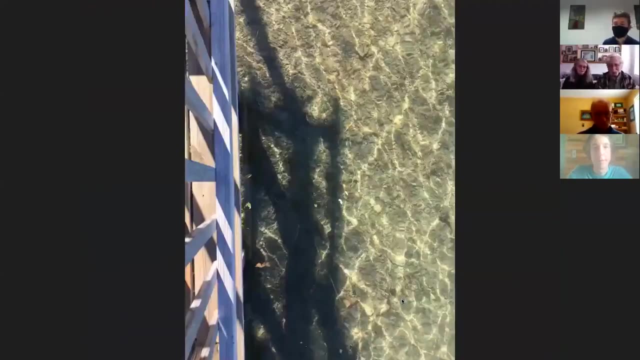 a very nice environment. This is Shelly's. gonna show you a lot of pictures of algae blooms, But this one we'll show you that it's not always the case that, viewed from our dock, on some days the water is crystal clear and you can see great detail. 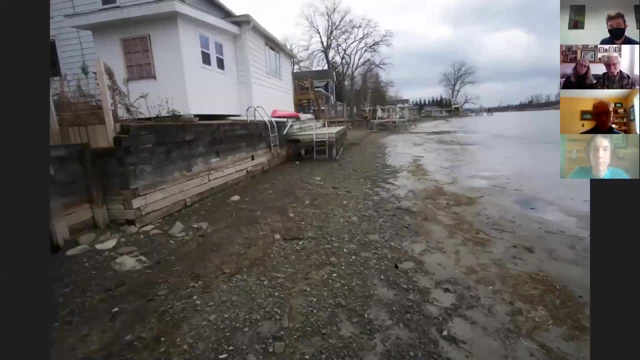 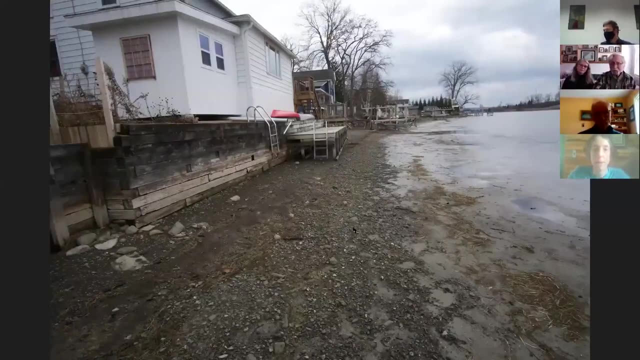 It's quite shallow here as well. This is a an image from mid January. At this point they've lowered the level of the lake a little more than three feet, And so much of our shoreline is exposed. You can get a sense of how gradual the slope of the bottom of the lake is. here We've only 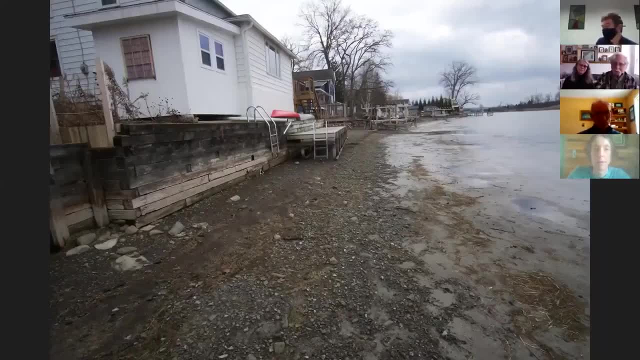 got about 18 inches of water here at our bulkhead and in fact we could walk all the way out to the channel if we were so inclined. The other thing I'll mention in this image is the sediment that begins out here, which we imagine is a nutrient-rich sediment that really covers the 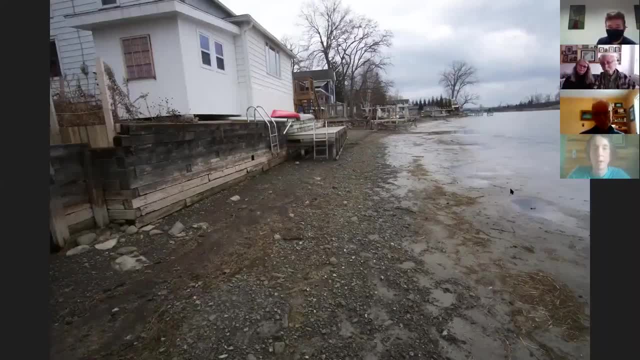 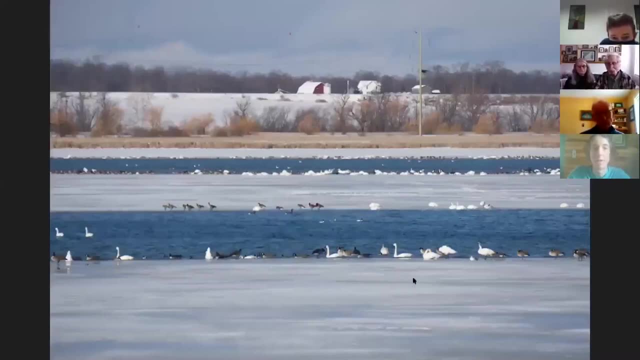 floor of the lake all the way out through this part of the lake For reference. a bit later in the season- this is about a month later- you can see the shallow water is iced over The channel. up here mostly stays open and we do have some of our favorite visitors. 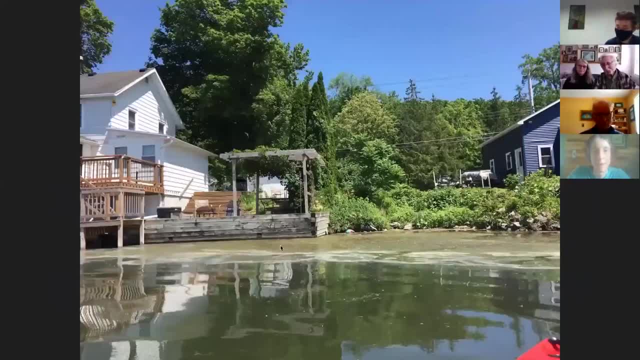 Here we're focusing again on our house, but what I want to point out in this image is that the bottom of the lake is a little bit deeper than the bottom of the lake. This is the amount of plant material that seems to be accumulating in our shoreline. It's a feature. 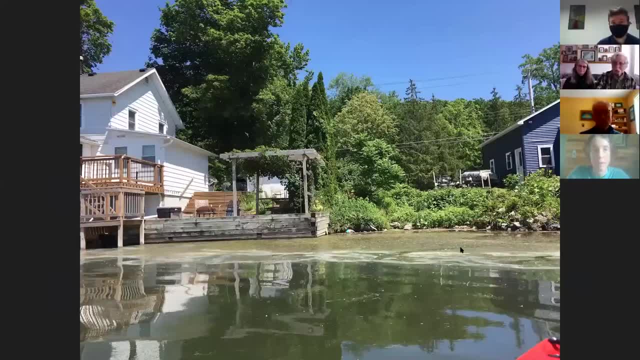 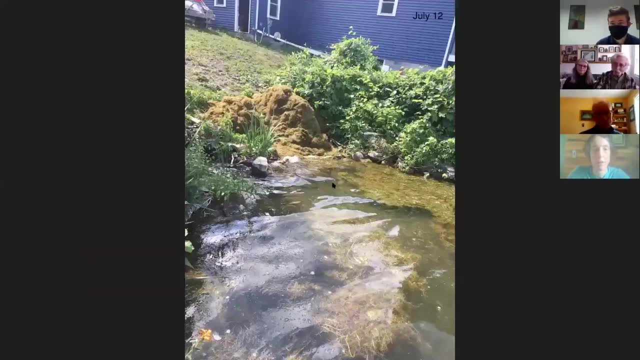 of where we live, that things accumulate here and to some extent, we've been able to make use of it. This is early in the season we've collected. This is sago pondweed, which we've got in great abundance. We've made use of it for compost and mulch, and it's a gift that keeps on giving Later. 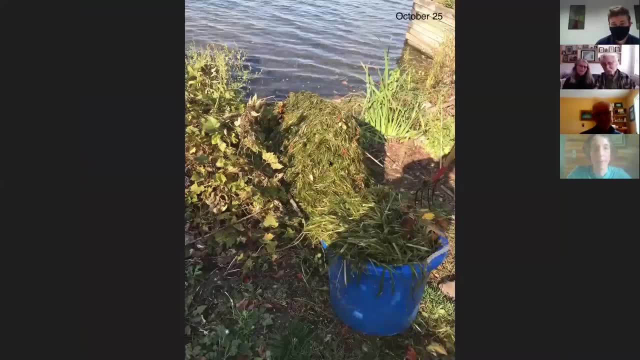 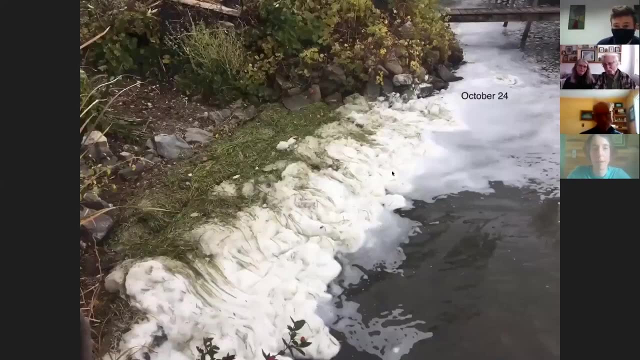 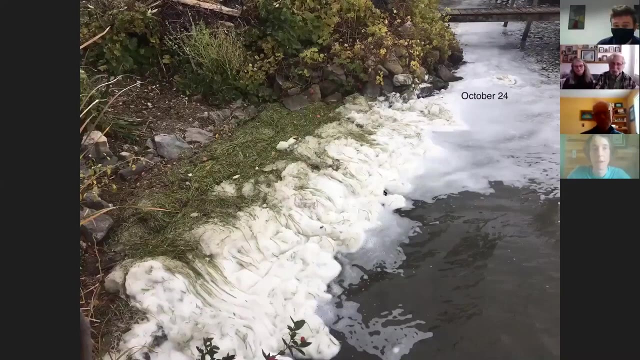 in the season, we've been able to continue to collect. This is an eelgrass, which dominates later. For reference, on windy days we don't see the algae blooms, but we do. Things still accumulate, and one of the things that some folks are interested in is this foam. 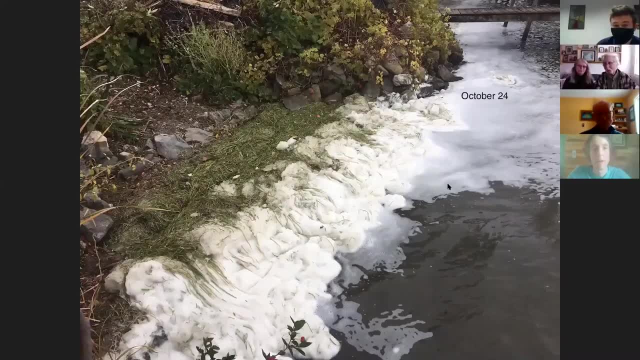 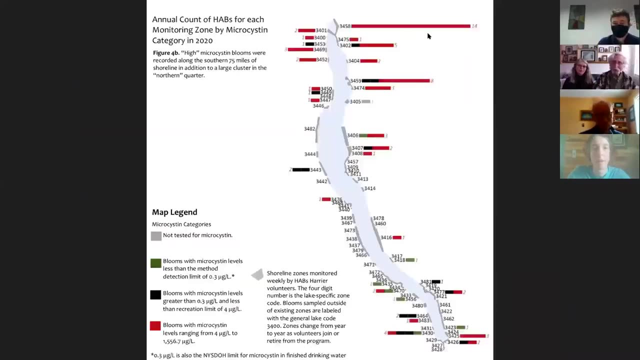 which we understand some people think may be related to the, to the blooms. So this is an image from a CSI report. This is our part of the lake way up here, and what you see is we have an embarrassing number of blooms that we were able to sample this year, and Shelly will talk. 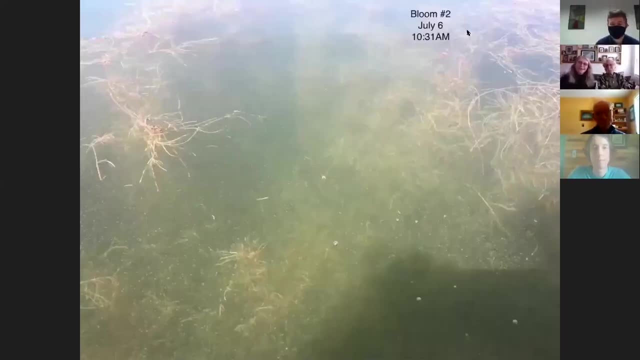 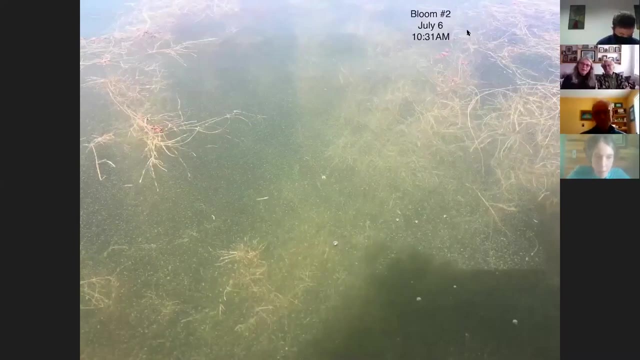 about some of those. The first bloom I wanted to call to your attention today is very early in the season, right pretty much at the beginning on July 6th, This was our bloom number two, and our habit when we monitor our zone is to paddle out into the middle of the lake and straight. 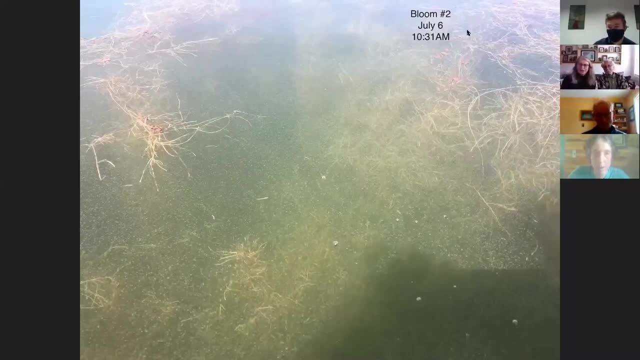 to the north end and then slowly come back down along the shoreline where we expect to see blooms starting. But before we got to the north end or toward the shoreline, we were already seeing a bloom beginning, and this was in the still water trapped among the plentiful sago pondweed. 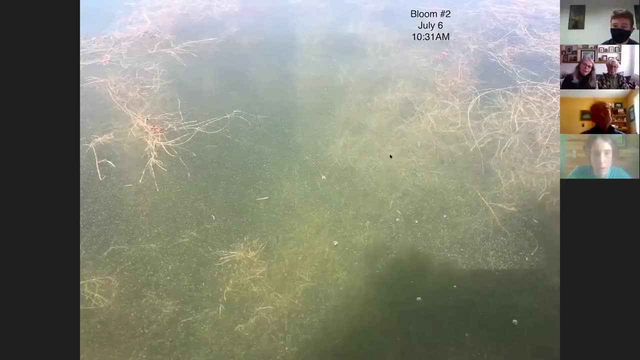 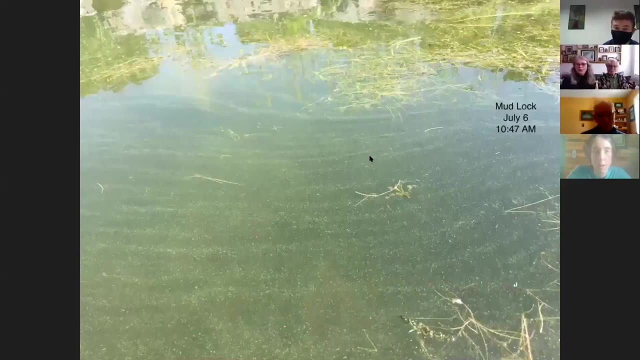 which is proliferating from year to year, and it was very hot. It was a sunny day and it was happening quickly. As we approached the shoreline, at Mudlock, we could see the the HAB was starting to make streaks along the shore. 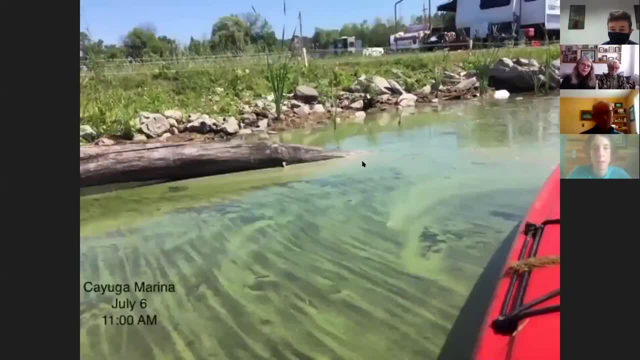 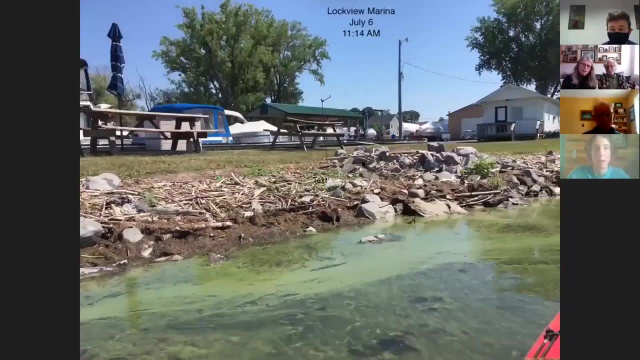 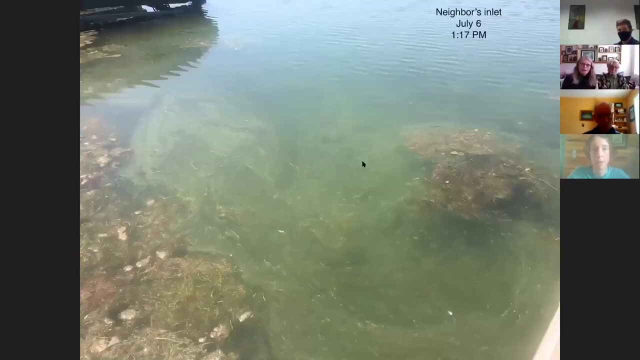 and continuing south. by the time we got to Cougum Arena it was quite intense and that's where we decided to sample. And further down the shoreline it was also bad at Lockview Marina and by the time we got back to our own shoreline around noon we could see it was beginning to. 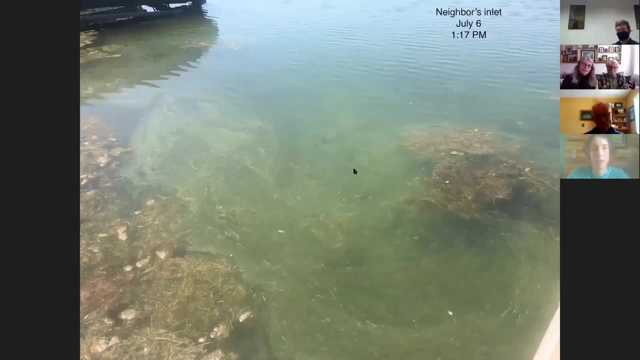 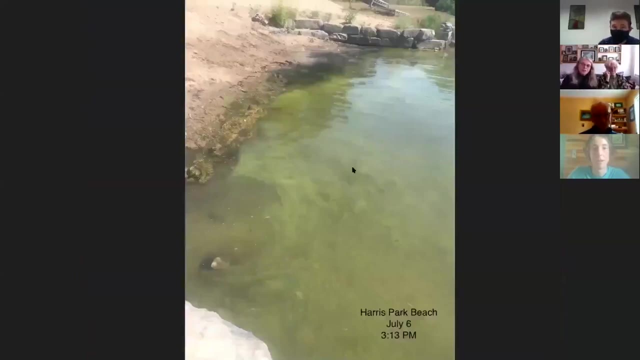 happen there also, By a little after one. this is what it looked like in our neighbor's inlet, Because it seemed to be such a pervasive bloom. we did check out Harris Park Beach, even though it's not part of our our zone. it's just a little to the south of us. 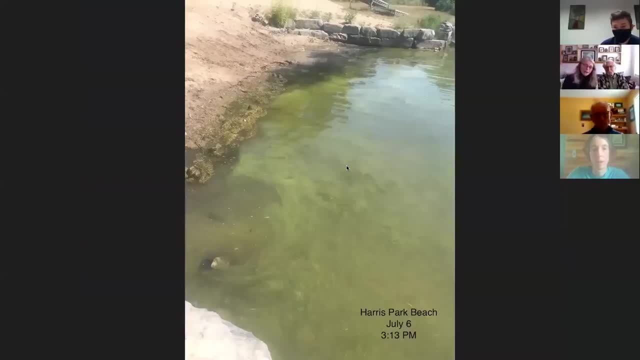 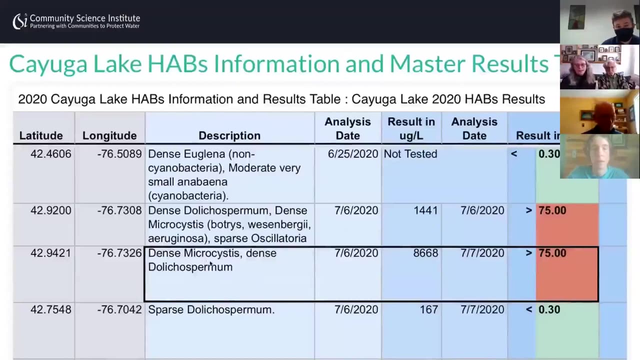 and it was also quite bad there. Luckily the beach was closed. So there we go, The results from bloom two. this shows that it had dense microcystis, which I understand is unusual for that early in the season, and it had a high chlorophyll and also significant toxicity. 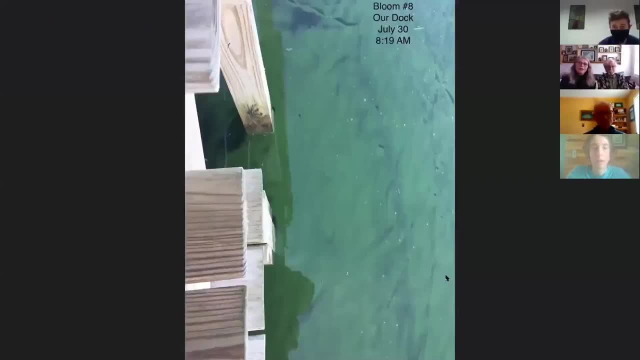 The second bloom I want to show you was later that month, on July 30th, bloom number eight. The notable things about this bloom was that, you know, it didn't have a lot of water so it didn't just happen then, but it began to start next week. 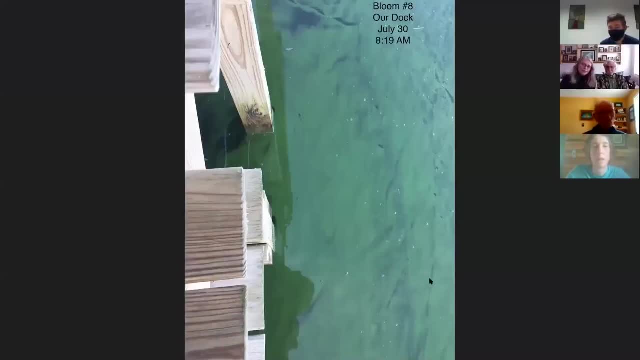 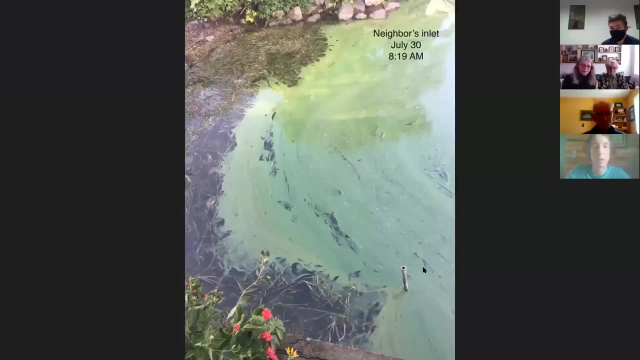 We often see incipient blooms early before seven o'clock sometimes, but this one, by a little after eight, was looking quite intense, And this was where we sampled from our neighbor's inlet at that time. The other thing that's notable about this bloom was that it persisted into the next day. We have a little trouble sometimes distinguishing when we planted ourselves out later. you know one on the summer day, the guy who planted in the evening. we then decided to plant the flowers just a little later, but they had a little more time. 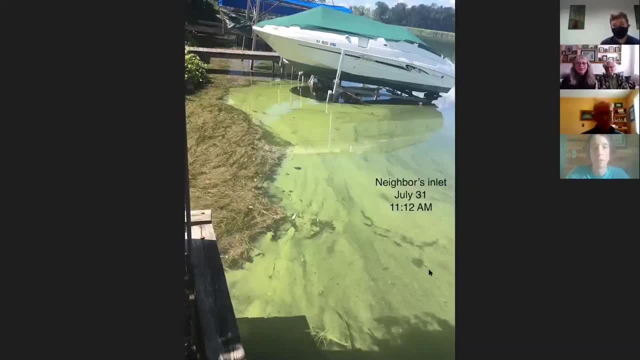 So we got a really good look at the flower. we'll get a lot of fields. didn't have enoughを. one bloom ends and another begins, So the rule of thumb that we've been using is 24 hours without detecting a bloom. This was clearly the same bloom. 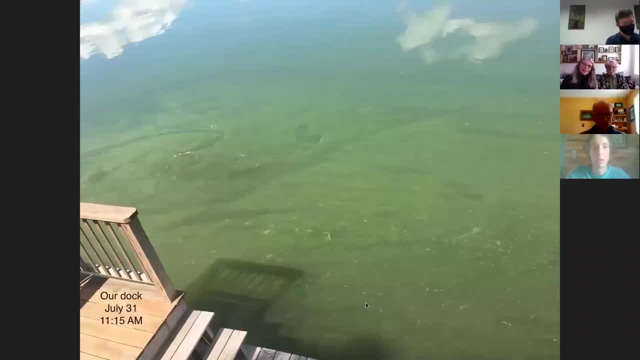 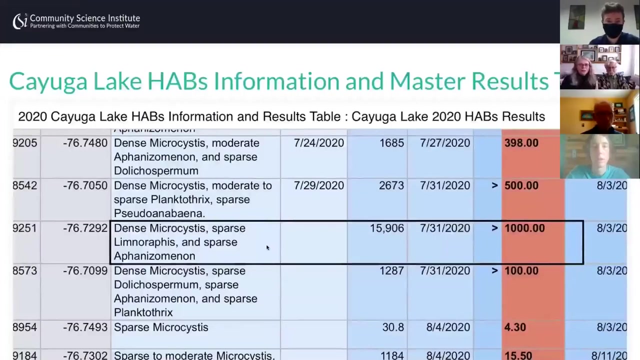 And looking out from our dock at that time on the second day, you can see how far out it extends into the lake. There are times actually, when this whole end of the lake has kind of a greenish cast, And here we show from the master results table at CSI. 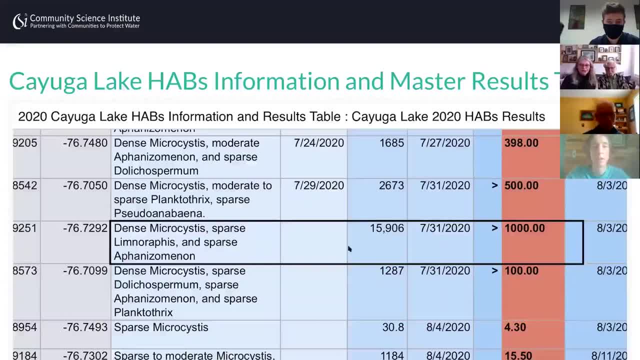 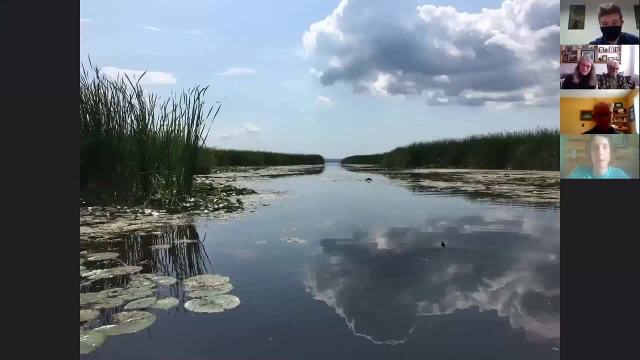 the dense microcystis was also characteristic of this bloom. It had an even higher chlorophyll and a scary number for the microcystin toxin. So it's an attractive place that we live in, Attractive to birds and wildlife and people like us. 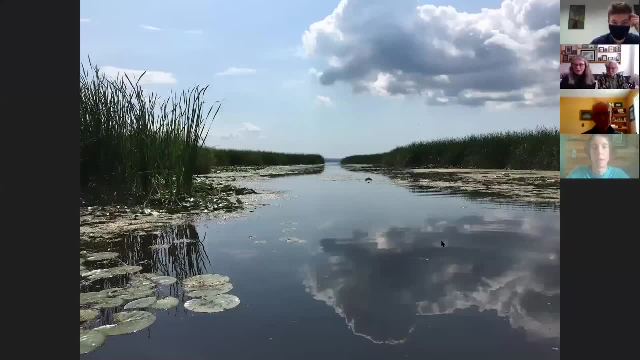 who like the gentle waters To paddle around, but it's also conducive to haves with the sheltered shallow, warm, relatively calm and, we think, nutrient-rich water. So, to conclude, we do have concerns about the lake as a whole and about our little corner of it. 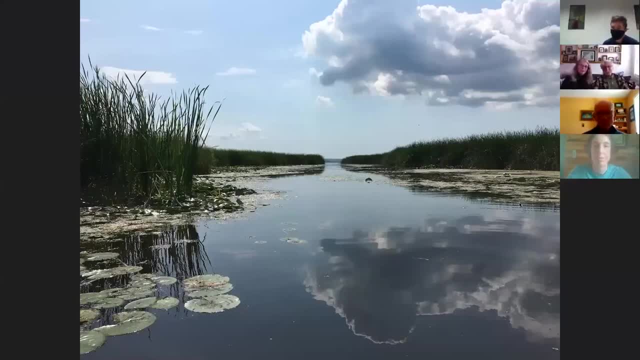 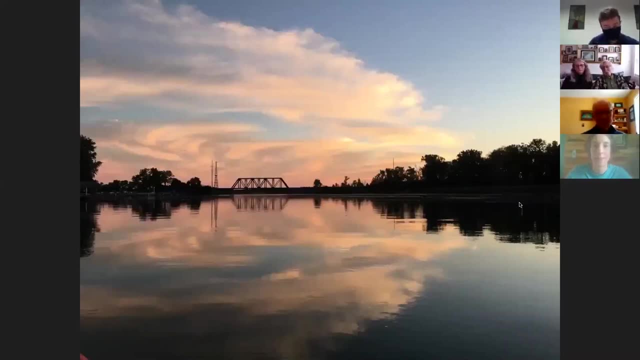 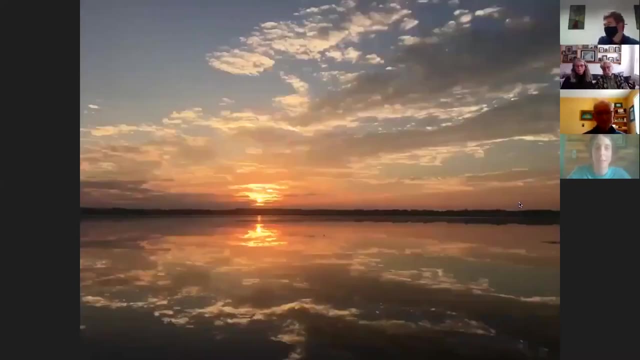 but it's still a beautiful place And just to point out more of the beauty, we'll show a few of Shelly's images of the many, many sunsets you get to watch If you live here, and it is an environment that is worth nurturing. 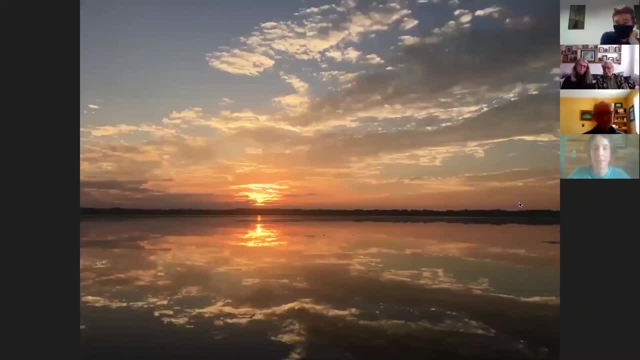 And we are grateful to scientists for helping us find out how to be better stewards. And now we'll turn you over to an actual scientist, Adriana. I'll mute myself first. Thank you so much, Shelly and Sai. It was really great to get that perspective. 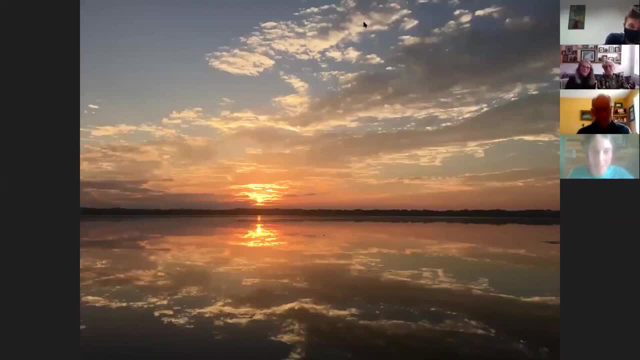 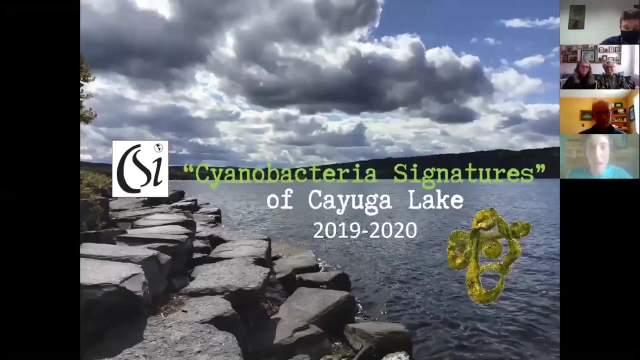 And you have such a beautiful slide here and sunset that I loathe to bring my screen up, but I will do that. Here we go, OK. Another view from the south end of Cayuga Lake. So what I'm hoping to do in my short time with you. 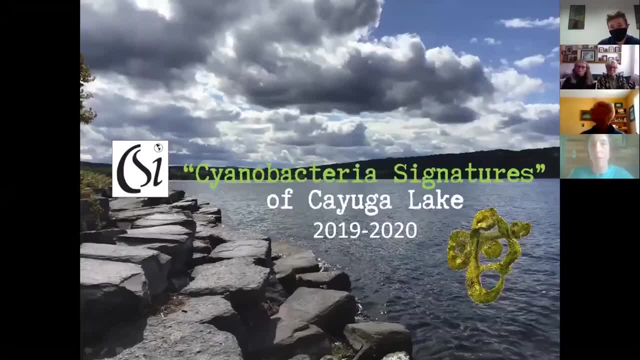 is just take you on a little tour of what we do with the second bullet point that Steve mentioned earlier and of looking at the ecology of the lake through the monitoring program, looking at non-bloom times and what we see in the waters. 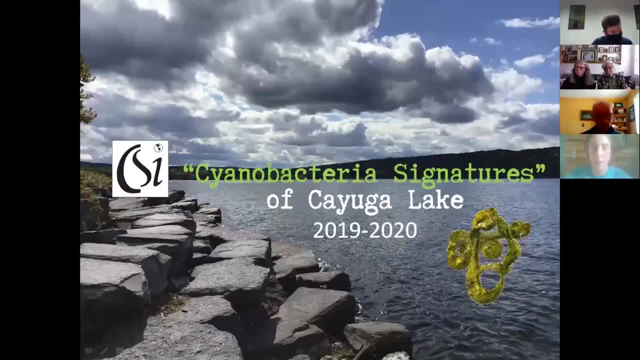 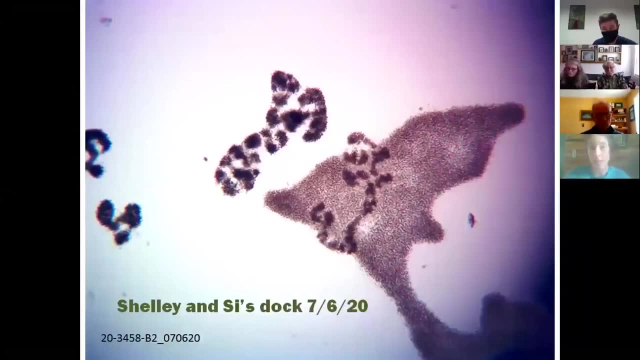 Cyanobacteria and otherwise. we're going to focus mainly on cyanobacteria and show some pictures. So to start off with, there are always multiple perspectives on any view of the lake, And you guys just saw some photos of some intense blooms up at the north end of the lake near Shelly and Sai's dock. 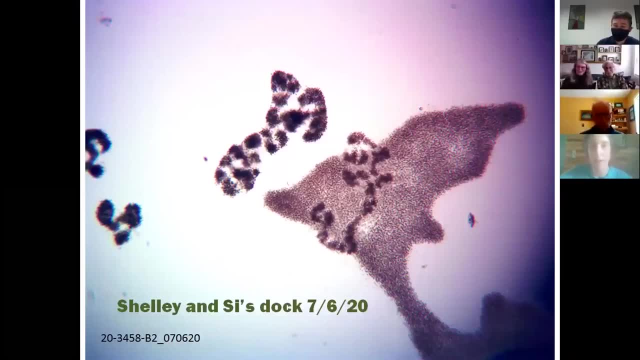 And I labeled this Shelly and Sai's dock. but I realize now that the photos that you showed were also of other places and you may have sampled in other places. So when we received the sample at CSI's lab, I take a drop of water from bloom samples. 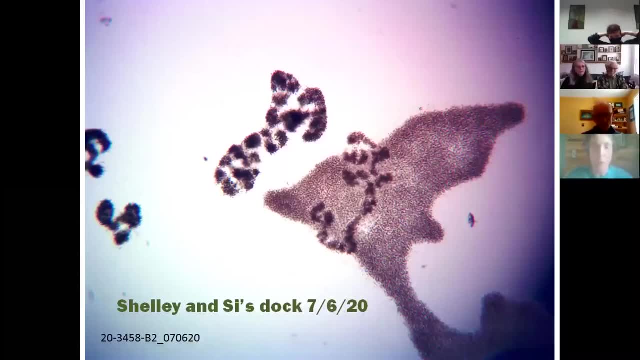 and look at them under the microscope. So this was that early July bloom looked something like this And of course it's a whole wild landscape as you scan through. This is a couple of millimeters field of view of what you might see. 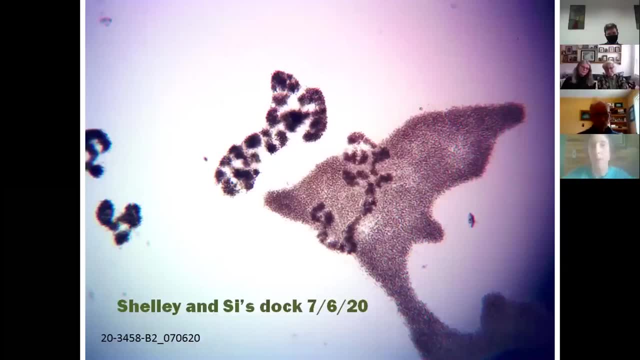 And this is microcystis, how it appears under the microscope. Each of those little dots are little individual cells that accumulate in these colonies. This was actually the later bloom, So you can see a little greater density of the microcystis. 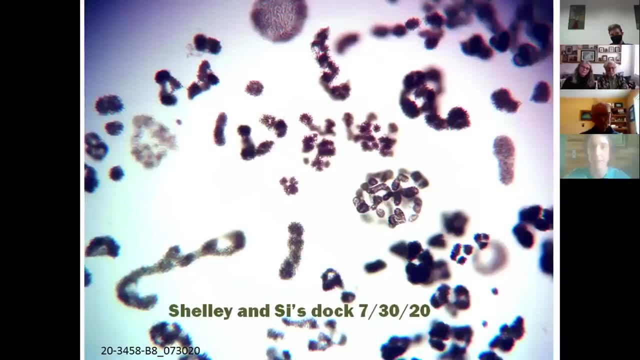 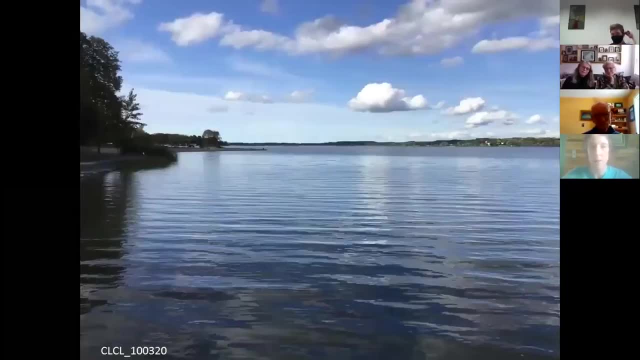 And here probably three different species at least of microcystis. But what about on a day when you're not seeing much out there in terms of cyanobacteria bloom? I know a lot of the HAB's Harrier volunteers. 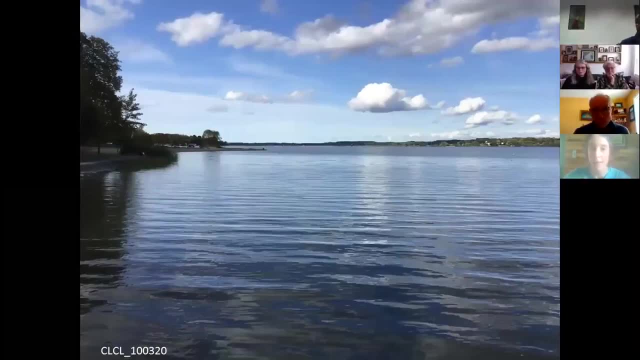 are really good at spotting the little flecks, the characteristic flecks that start to appear before you get enough accumulation of things like microcystis to form a bloom, And sometimes, if you look at that point, you can definitely still see colonies of microcystis. 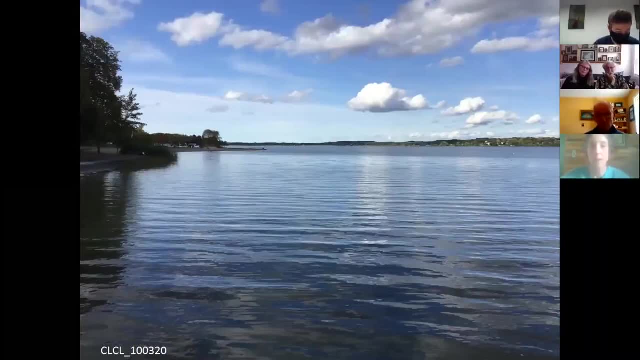 But on an average day on the lake when bloom isn't happening, if we just took a drop of lake water, we would have to search around quite a bit to see organisms there. They tend to be more spread out. So in order to look, 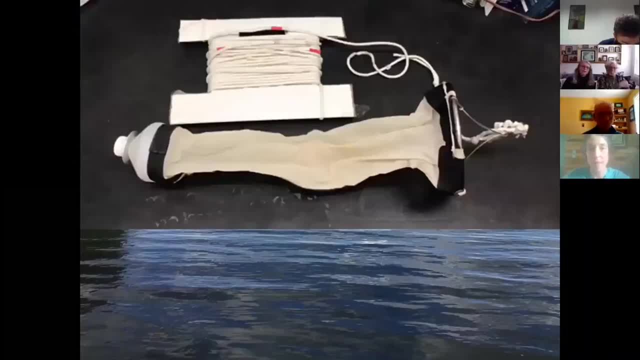 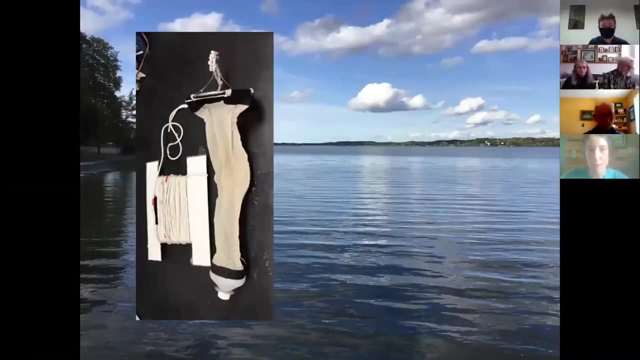 At these non-bloom samples. we use a plankton net And this is basically. you can imagine it as a sock made of mesh- really fine mesh- If you sawed off the, if you cut off the tip of the sock and you replaced it with a sawed off water bottle. 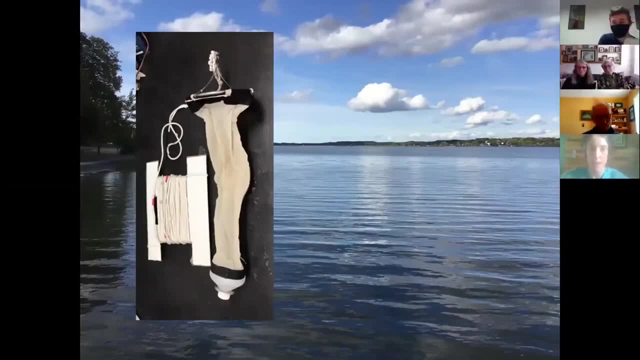 top with a little lid that you can remove, And the other end of the sock is like a metal ring that keeps it held open, And this is all attached to a rope. There's a little weight on the bottle end And in order to collect our plankton, 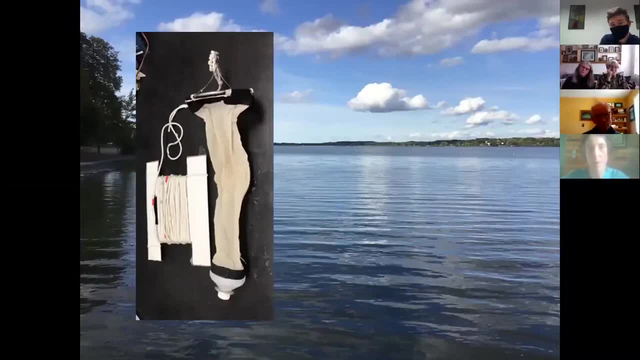 samples, we throw our plankton net out about three meters, pull it back. do that 10 times along the surface of the water. You can also get really fancy plankton nets and use them to sample at depth and have it close while it's down under water and pull your sample up. 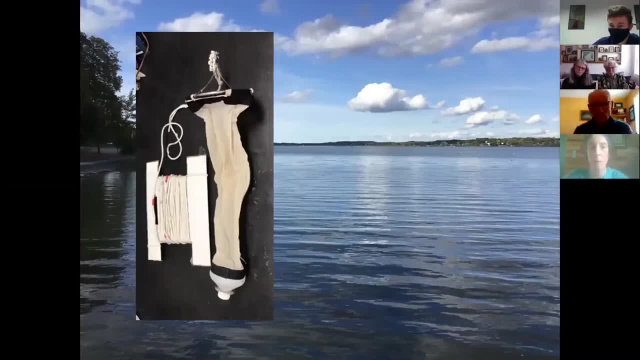 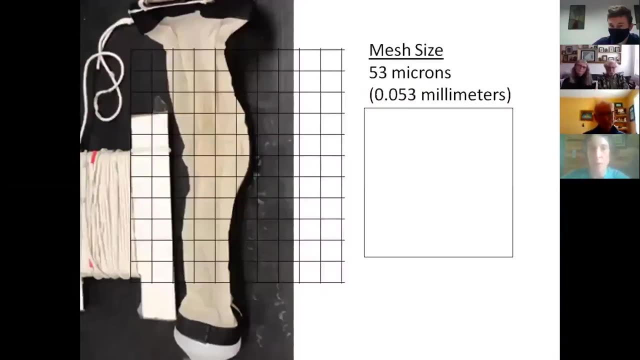 But we've been mainly focusing with our surveys on what's happening right near the surface. So the mesh size that we use is 53 microns, which is pretty small. If you go any smaller than that, I think things tend to get clogged up. 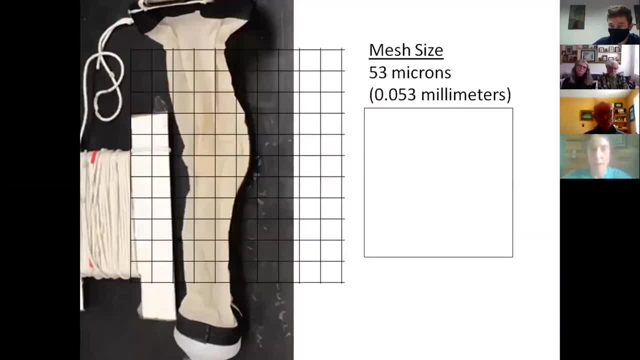 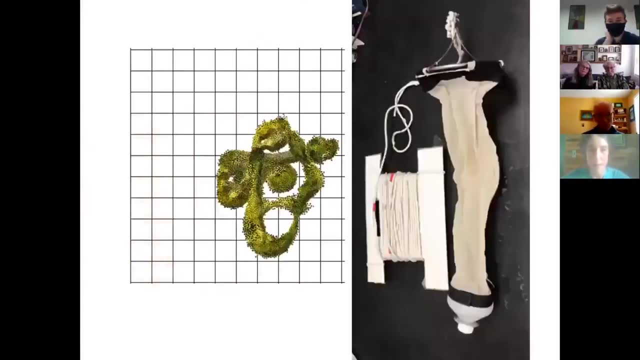 But just to give you a sense, there's about in one micron, there's, or in one millimeter, there's about 1,000 microns, And here's an example of a microcystis colony being trapped by the mesh of my net. 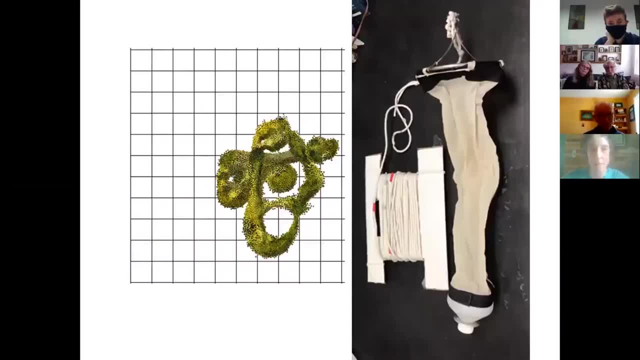 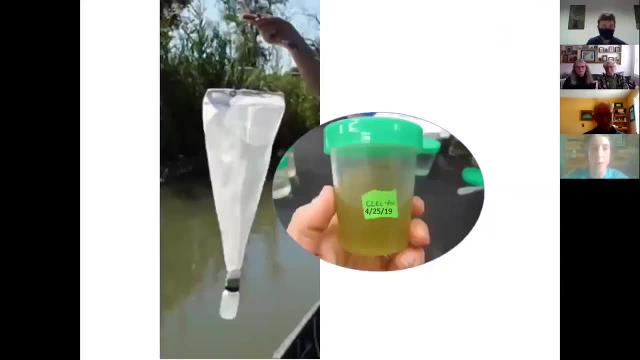 That's about how, if this is like 300 microns across this colony, this is about what that would look like: caught on the mesh, The material accumulates in the bottle at the bottom of the net, And this is a slightly different model than the one 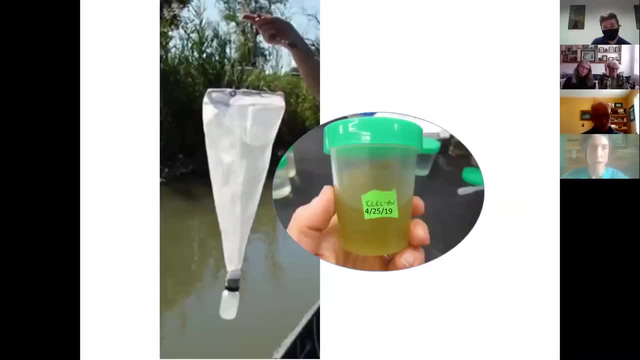 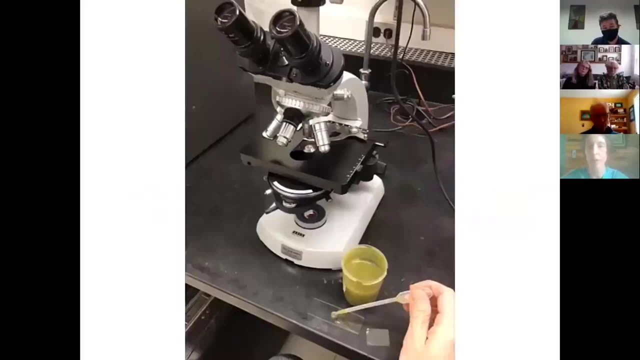 that we use in the picture. But then you take the bottle off at the bottom and pour it into another sample container, bring it back to the lab and take a drop out of it. The sample that you see is a little thicker than kind of a normal non-bloom conditions. 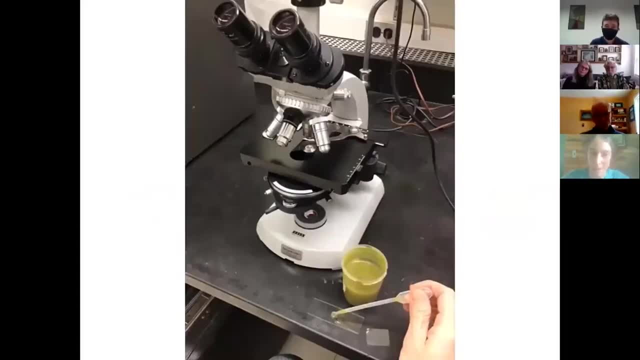 This was actually a sample. I took this picture just a couple of days ago. It's a leftover sample from July where it was Bloom conditions many places on the lake. This was a sample from Cayuga Lake State Park where it was sort of pre-bloom conditions. 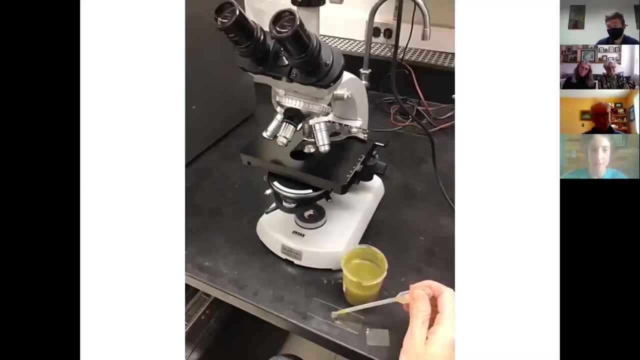 And when you concentrate it it gets pretty thick like that. Now this smells really terrible. I wish I could project the smell to you opening this jar. But basically, I just wanted to show this idea of taking a drop and then we look at it under the microscope. 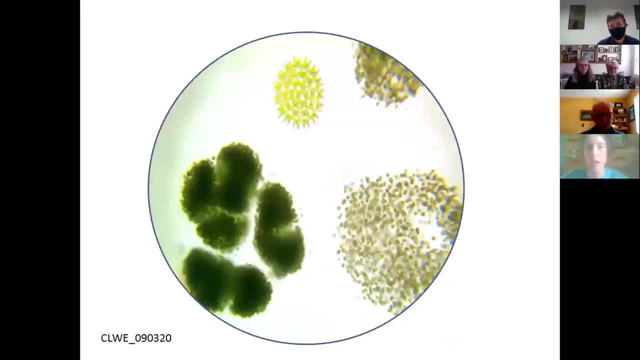 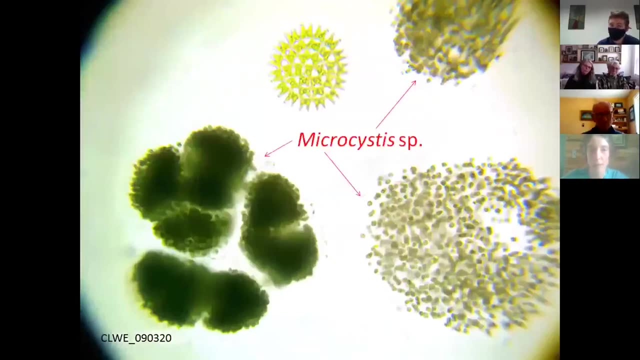 This is not that same sample. This is from the Wells College doc, from our summer surveys, And if you're getting familiar with recognizing microcystis, you could see You can see that there are some microcystis there. Microcystis tends to look a little darker and less colorful. 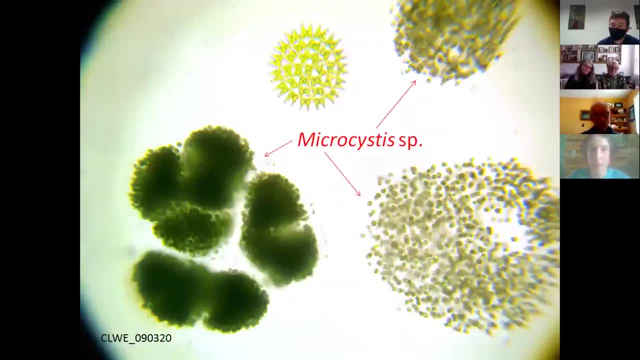 than some of the green algae, like this pediastrum, this colony of pediastrum up here. The reason that microcystis and some of the other cyanobacteria that we find in the lake tend to look less colorful is because they. 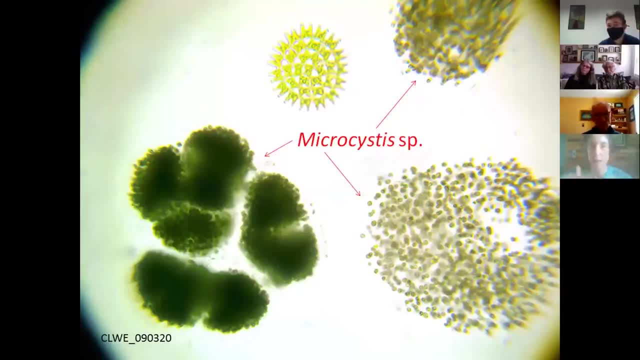 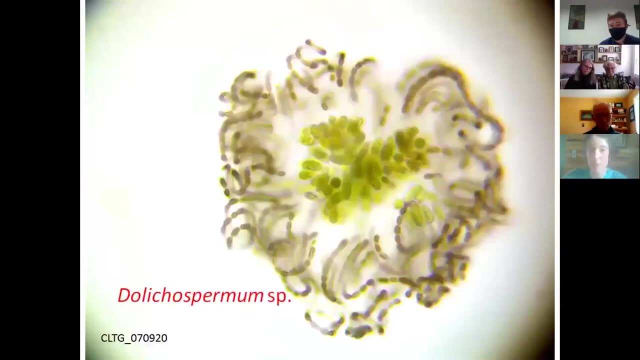 have erythropes in them, these little gas vesicles that allow them to regulate their buoyancy and move up and down in the water column. Here's some Dolichospermum, So this is another common bloom-forming cyanobacteria that we find in Cayuga Lake. 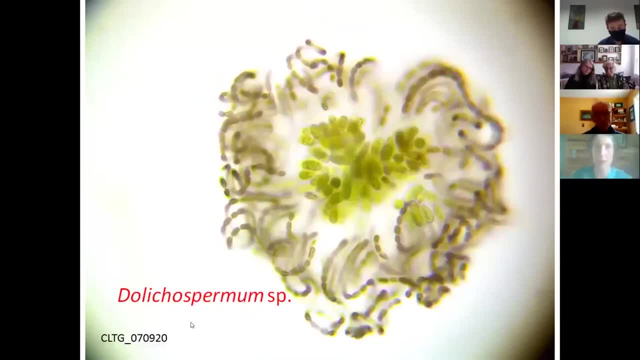 This is an interesting picture because the center of it has an accumulation of aconites which is sort of a resting stage for cyanobacteria- for some cyanobacteria, So when conditions are not so great for them, they can go into this sort of resting form. 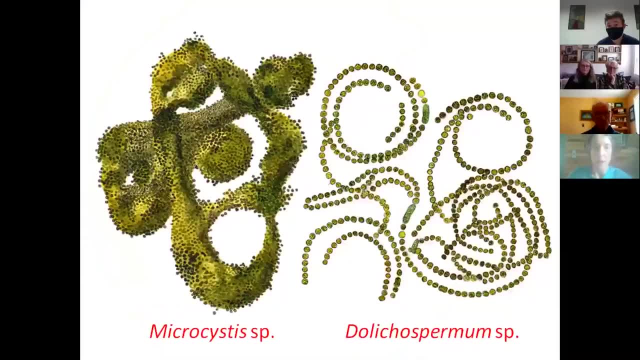 and then kind of come back later when things look better. So just to give a brief introduction to what are cyanobacteria: Microcystis and Dolichospermum are the main bloom-forming cyanobacteria that we find in Cayuga Lake. 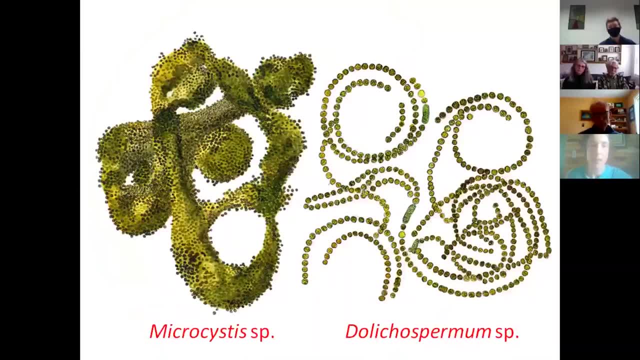 We do find some other bloom-forming cyanobacteria, but typically these are the ones that are dominating the blooms, And the microcystis blooms tend to be associated more with the microcystin toxin that we find at the lab. 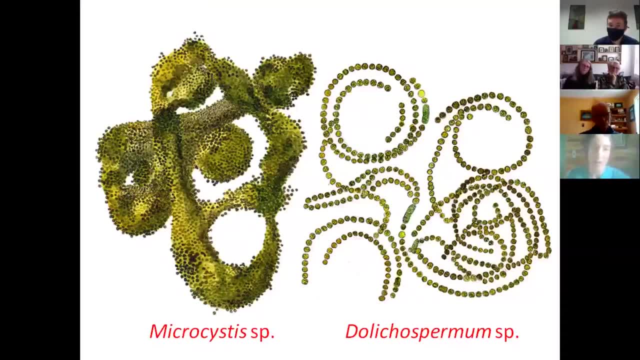 So cyanobacteria are prokaryotic organisms, So they have no nuclei and they're very ancient. They've been around since early Earth. You could basically say that cyanobacteria invented photosynthesis, or at least the type of photosynthesis. 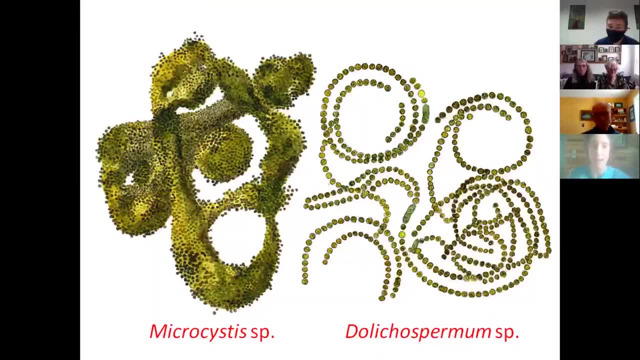 that we're familiar with, where carbon dioxide is taken in and then oxygen is given off as a waste product. They're actually much more efficient than green plants at doing photosynthesis and giving off oxygen, And it turns out that green plants- the chloroplasts in them were originally 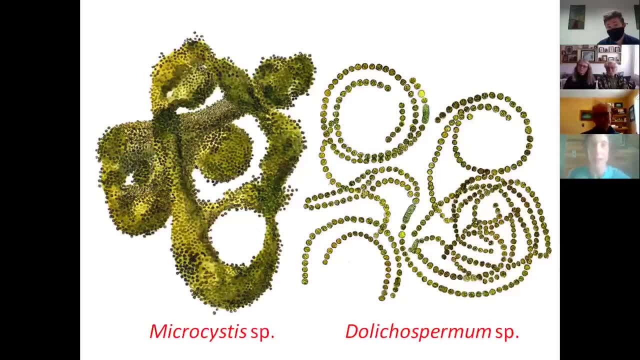 free-living cyanobacteria that, through symbioses, now are in the leaves of all plants. So all photosynthesis on Earth. you can thank these cyanobacteria, And they're everywhere And everywhere where there's water, even water in the air. 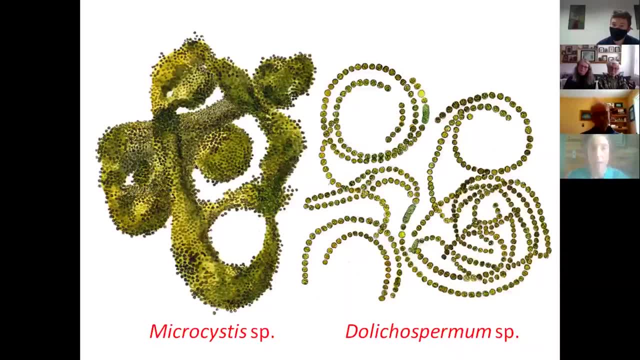 sometimes can have cyanobacteria in it. They do some really interesting things. So some of them, as I've mentioned, and including both of these, Microsystis and Dolichospermum- they have aeratopes so that they can regulate their buoyancy. 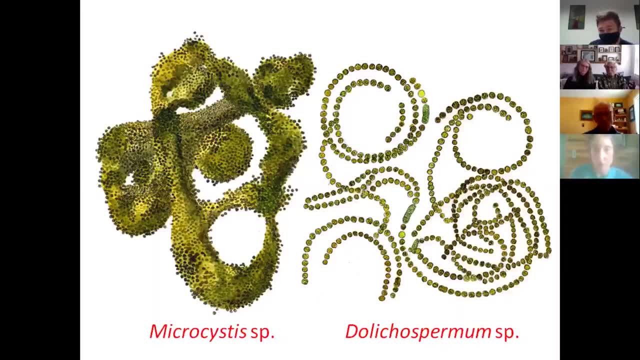 moving up and down in the water column depending on how much sun they want to get in particular conditions. They also Dolichospermum has a different sort of structure than the Microsystis. Microsystis cells are all clumped together. 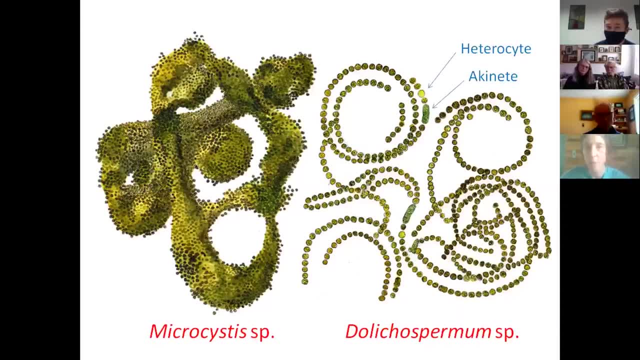 in these colonies And Dolichospermum tends to form more of these necklace structures. Sometimes they're tangled, Sometimes they're neat little spirals, But Dolichospermum also produces both the aconites that I've mentioned already, these sort of resting cells. 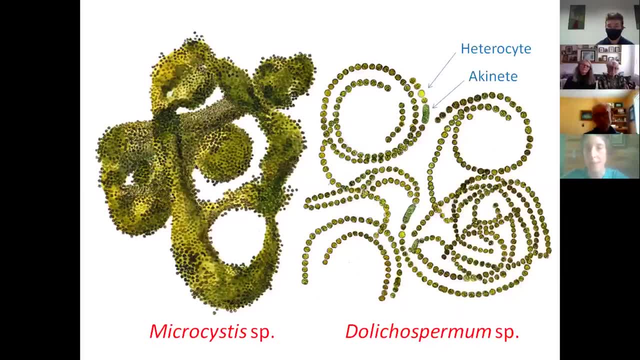 and also heterocytes, special cells where they fix nitrogen from the atmosphere. There aren't many organisms on Earth that can do that, And they are able to then utilize that nitrogen that's abundant in the atmosphere but can be a limiting nutrient for growth. 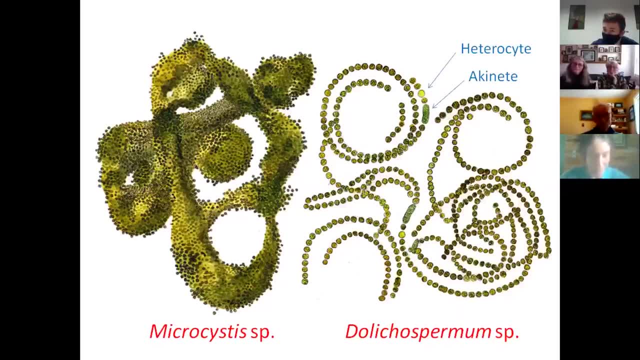 Oh boy, it's so hard. As I mentioned earlier, I could talk for a day, probably, about cyanobacteria, And this is the danger of me going too long, But I just want to make sure I cover some of the basic pieces of this. 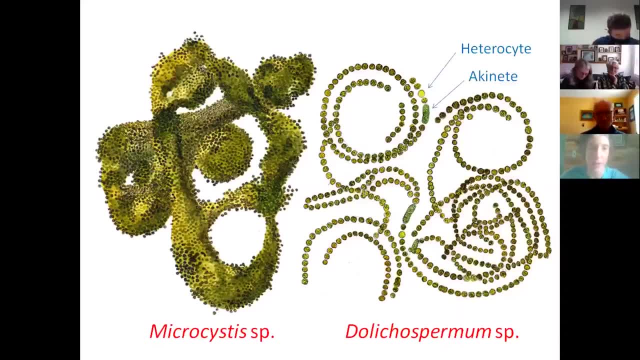 One other important factor I think to understand about cyanobacteria is that they don't reproduce sexually, So that the way that they reproduce they are sort of clones of each other, But they are able to sort of mix DNA in a way that bacteria 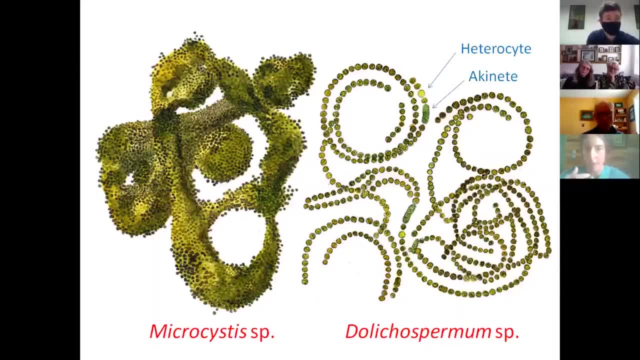 which is they can basically, essentially by bumping into each other- can share DNA, which is very different than organisms like us, who have all their DNA packed neatly into nuclei. So, for example, the creation of toxins can be shared between different species sometimes. 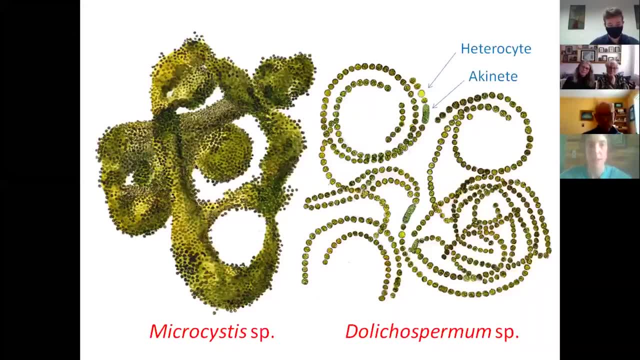 So not all microcystis may be producing microcystin toxin, but they can do it And potentially they could even share that information with other Cyanobacteria. OK, now I'm going to move on because dolichospermum. 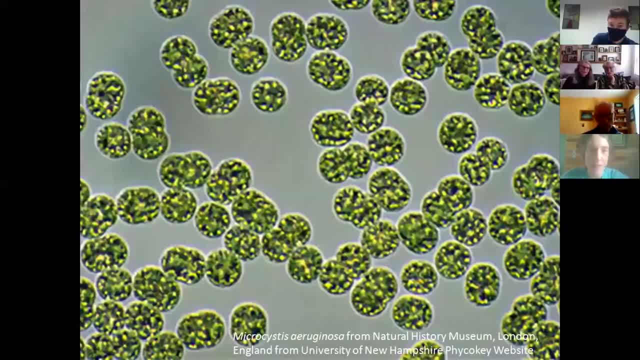 and microcystis are not the only cyanobacteria. This is actually a close up of microcystis still lingering there, But I like the picture because it shows, gives a little bit of a sense of the aerotopes which. 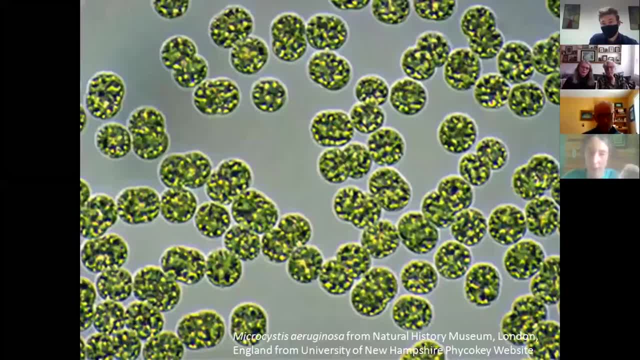 are actually very hard to see. sometimes under the microscope You're looking kind of almost for a little glint of red gleaming out, But it helps you identify microcystis and some of these other boon-forming cyanobacteria. Here's a nice photo of dolichospermum. 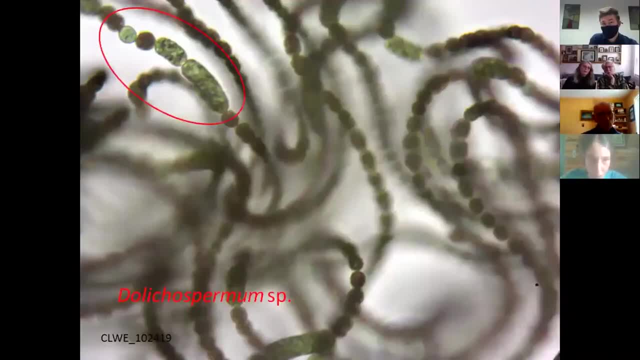 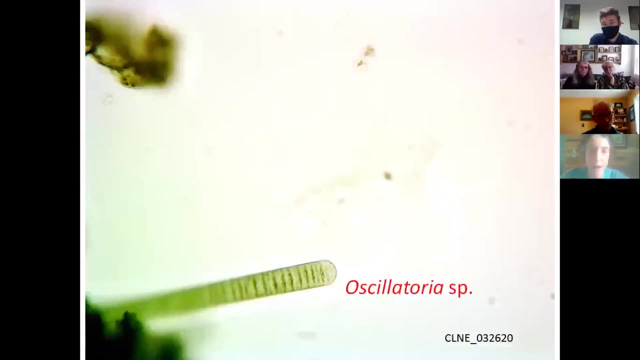 where you can see the heterocytes and aconites, Another one with heterocytes slightly different form, And then there are other cyanobacterias that we see out there And while none of them have been our main boon-forming cyanobacteria now, who knows if that could change. 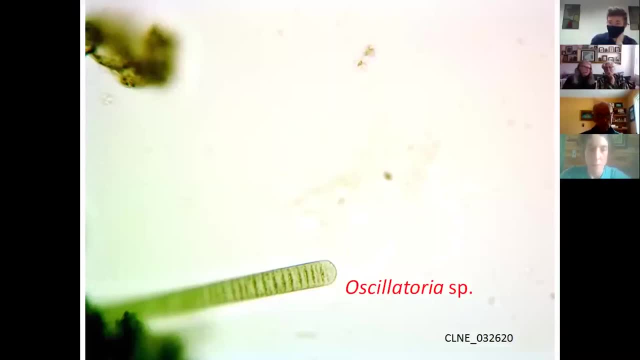 at some point in the future. Oscillatoria are really interesting. They're filamentous, This little sort of snake-like thing coming out of the bottom, And I say snake-like because when you see these under the microscope they actually do slither across your field of view. 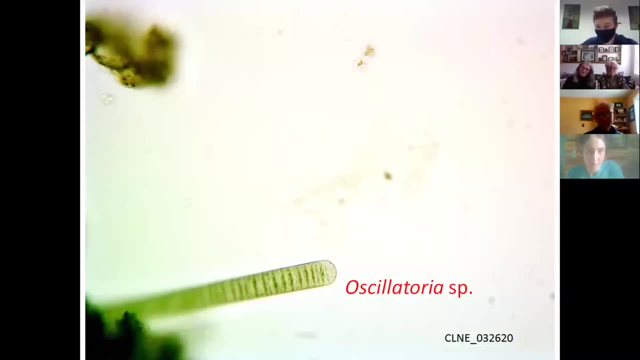 They have a way of secreting substances that make it so that they can move. It's really kind of fascinating. But Oscillatoria are known toxin producers. They don't have aerotopes, So typically they're sort of benthic or dwelling. 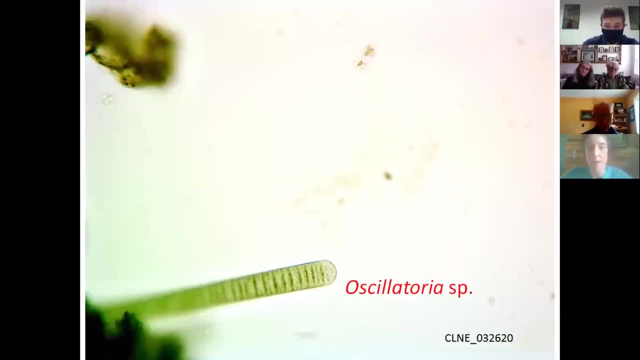 on the bottom, Although this summer at East Shore Park I started seeing clumps that were Oscillatoria floating on the surface. So maybe through the oxygen that they're producing, creating little air bubbles, they're able to float on the surface at times. 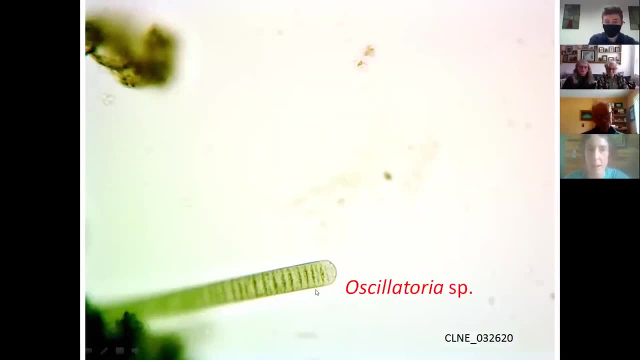 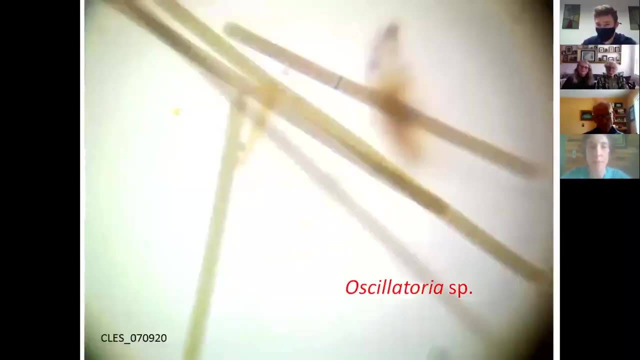 And back in 2019, there were like three dog deaths in one day on this particular pond in North Carolina And they were associating those deaths with Oscillatoria. Here's some more Oscillatoria from this past summer at East Shore Park. 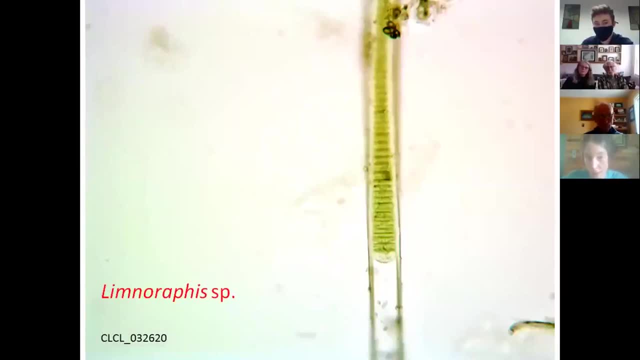 And there's another cyanobacteria that looks really similar to Oscillatoria, But it actually does have aerotopes And it can be bloom forming. There are places where I've seen blooms- not in our area but other places- formed by limnoraphis. 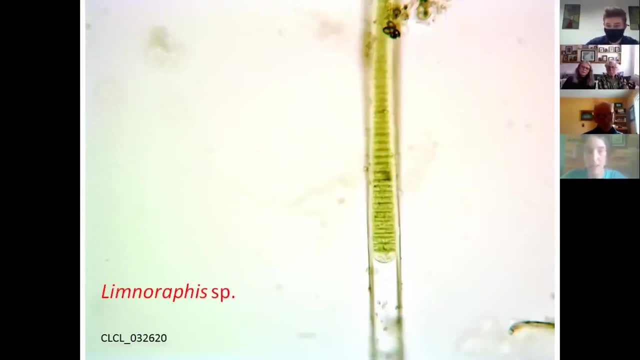 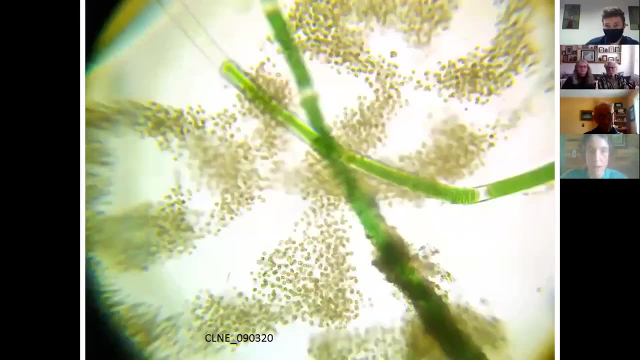 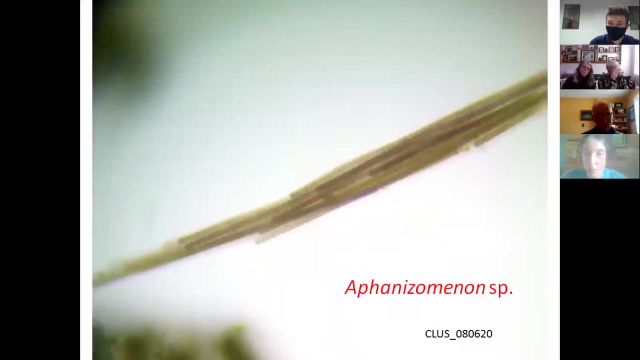 Also produces some different toxins, And this one has a sheath around it, So otherwise it looks very similar to Oscillatoria. And this is some more limnoraphis amidst some microcystis. Afanizomenon has this interesting way. 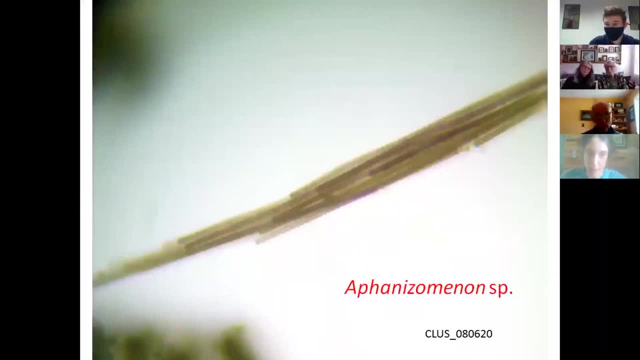 It's called a phytocephalus. It's called a phytocephalus. It's called a phytocephalus. They're filamentous, But they also form these clumps, And we've seen an afanizomenon bloom in a local pond recently. 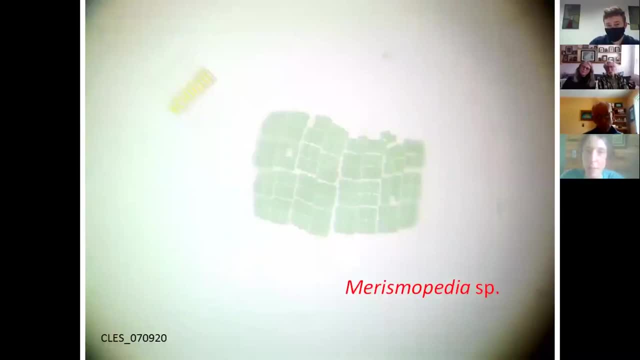 And, lastly, of the cyanobacteria that I'm going to show to you today. a marismapedia is a really fun one to find, And I'm not aware of it forming blooms, But it's like these little computer microchips. 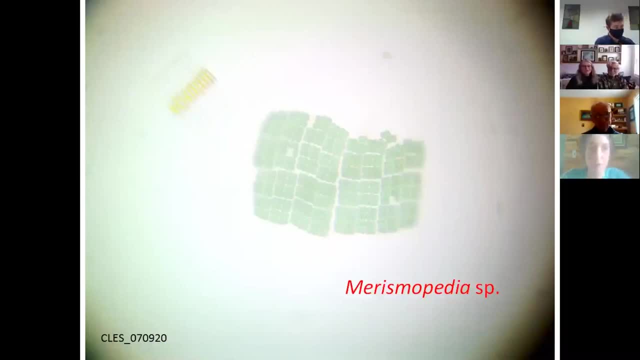 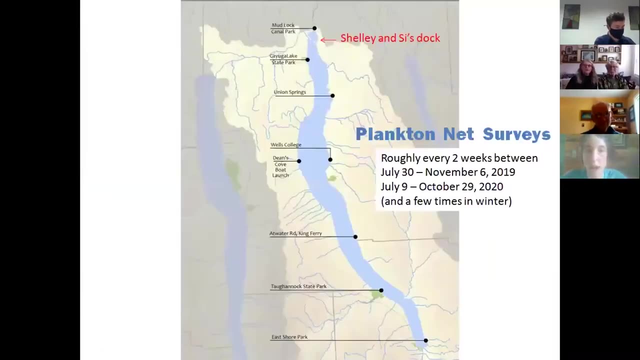 or something in the way that they reproduce and are just beautiful. And then there's a little Fragilaria up there, So you'll see that over here in the corner. So our planktonet surveys happened roughly every two weeks between the time periods listed here. 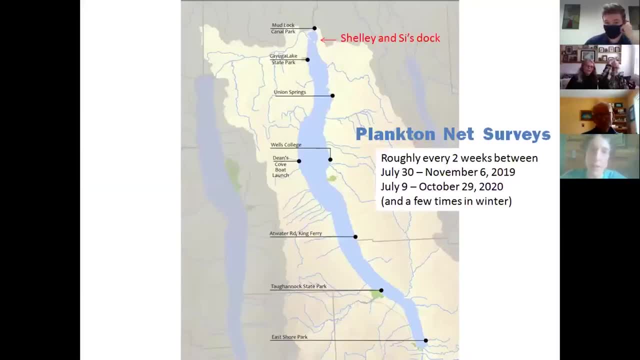 in both the bloom season of 2019 and 2020.. So these were the locations where we've been sampling. The locations were chosen because they were easily accessible And most of them are public locations, public parks and such- And we thought that that would also be more relevant to people. 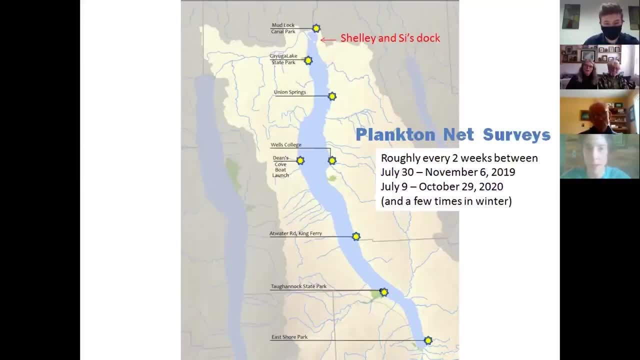 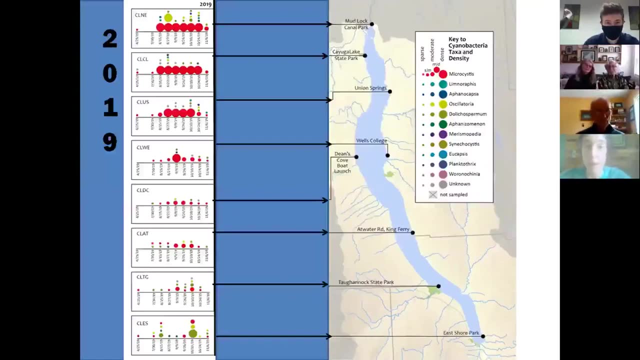 spending time on the lake, knowing what's happening in those areas. Let's see. this is an example of some of the results in terms of looking at the cyanobacterias that we've seen in at the different locations. So the size of the little dots. 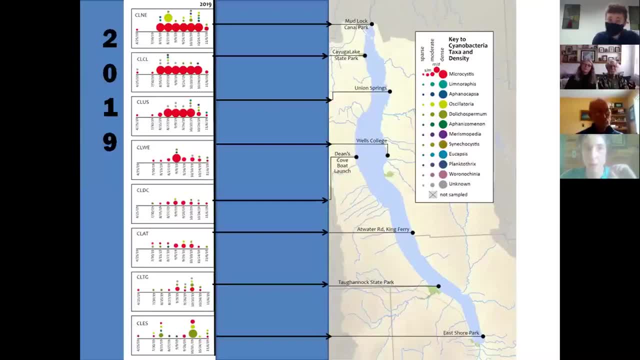 corresponds to whether samples were sort of dense, moderate or sparse with those particular cyanobacteria, And I'd encourage you to check out the CSI water bulletin which is on the website for if you want to look at this closer, We also explain how we determine the difference between dense, moderate and sparse. But 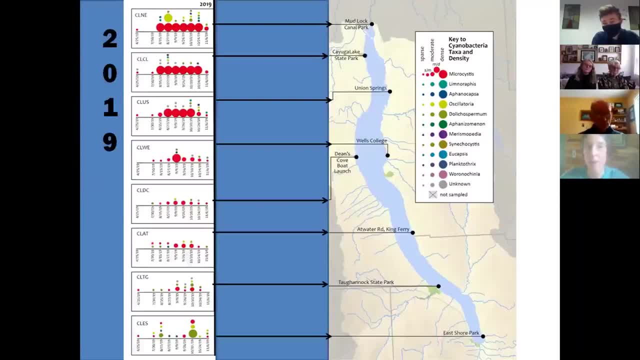 you can see that in the summer of 2019, this pattern started to creep up where there was really dense microcystis, typically at the north end of the lake. So these three locations up here- So Shelley and Tsai's dock is right up and up here, and then it's still very 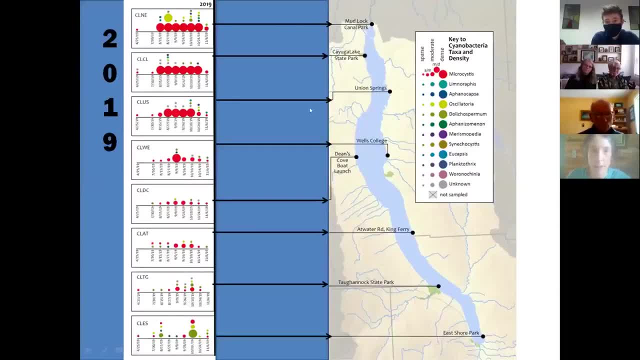 shallow in this whole part of the lake up in here And it just got to be this normal thing that when I'd go around the lake doing taking my samples I just sort of expected and was not- was usually not surprised by what I saw moving around. 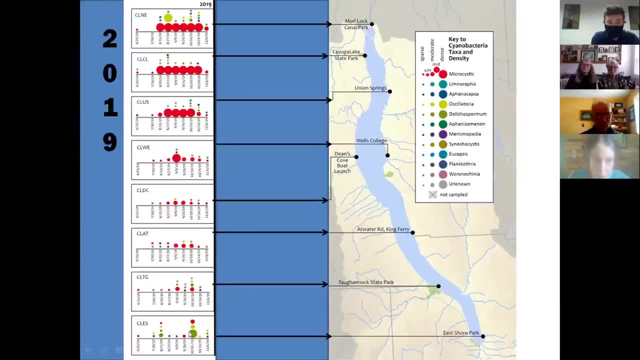 the lake And occasionally there were other dominant species and that we saw. Now just I have to emphasize that the samples that I have here are plankton net samples. So when I talk about dense microcystis in the plankton net samples, it's not the same thing as dense. 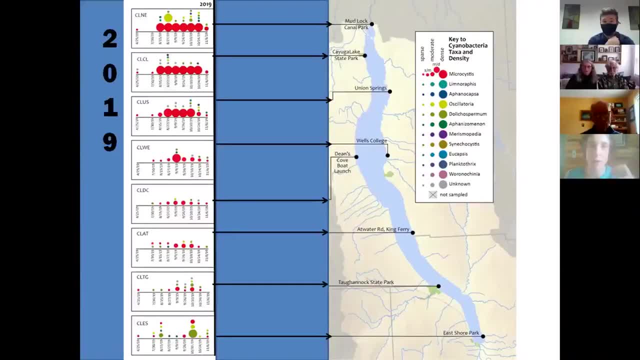 microcystis in a drop of water from one of the samples that a volunteer brought into the lake. Those are bloom conditions. Most of the time, these are not bloom conditions, but occasionally we've got bloom conditions as well. In 2020, things. 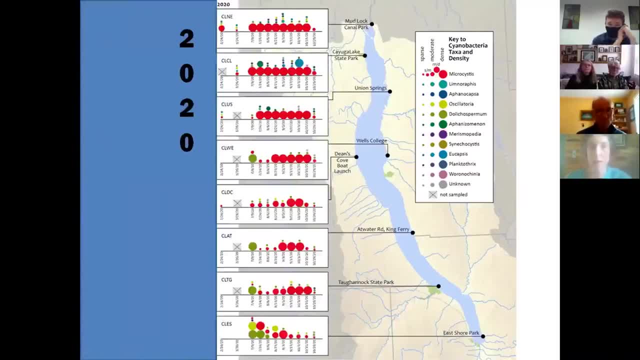 look different. I was rather surprised that rather than just finding the concentrations, the heavy concentrations of microcystis at the north end of the lake, we found them pretty much everywhere at different times, and so if you put look at those two years side-by-side, there's 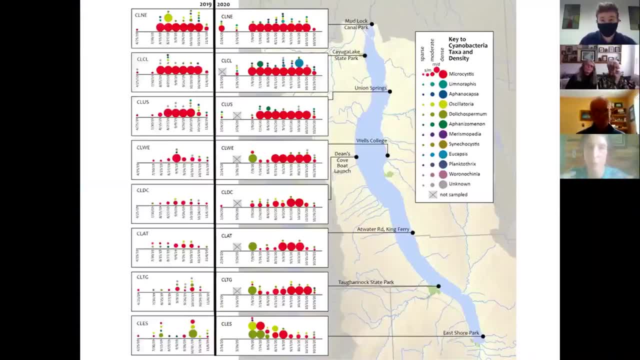 this sort of interesting pattern- or we've been calling it a cyanobacteria signatures- that we've been seeing in the lake, and this corresponds interestingly to the toxin- the high toxin blooms that Steve will talk about later- that, in 2019, tended to mostly be at the north end of the lake. 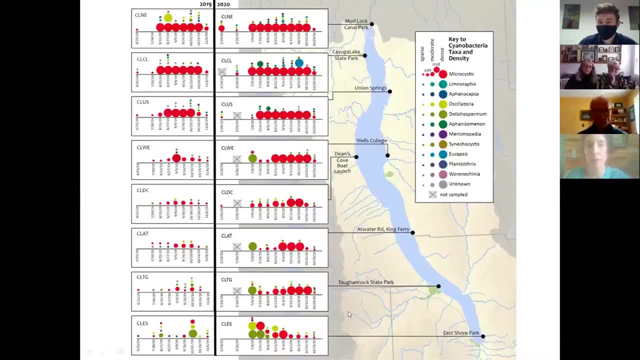 lake and in 2020 we also saw them in other parts of the lake. I'm just going to wrap up with a note on. I think I'm sure all of the CSI's HAB-Terrier volunteers are well aware that there's much to be gained from just that process of observation. I'm sure if we could talk to all. 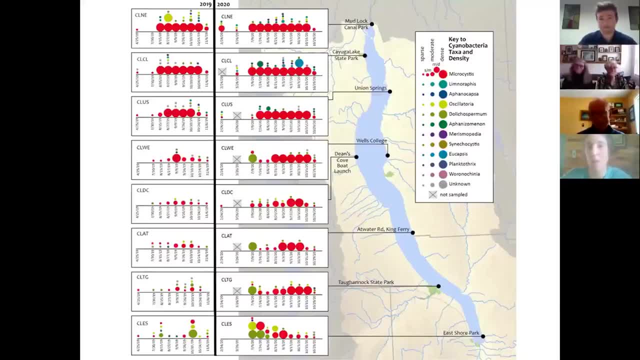 of our volunteers. we'd hear stories about the things that they noticed because they were out there looking for cyanobacteria, And I would say the same thing about this plankton survey. it's really interesting, even just the process of driving around the lake every two weeks and 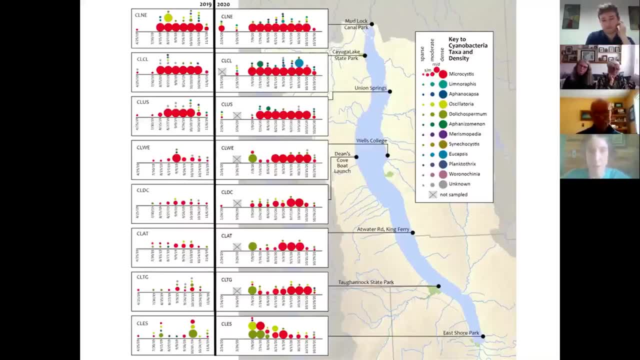 the things that you see. I saw times when there were fish kills up at the north end of the lake that I never would have otherwise known about, or in some heavy construction that was happening right on the lake shore. that could potentially influence what's going on in different areas, and 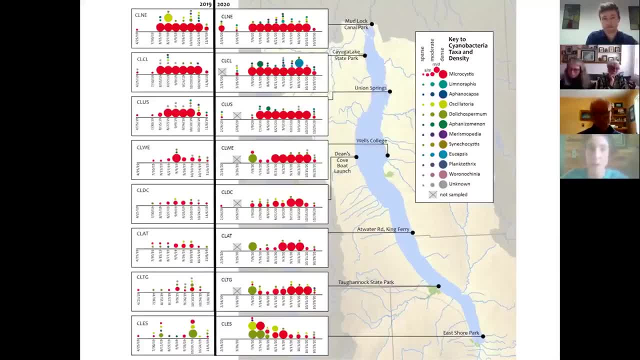 you kind of know that when you see those things and when you're out in the field. And in terms of the plankton survey, I think that's something that some of the organizations and organizations surveys. I think one of the most important things to remember about all of this when we're thinking. 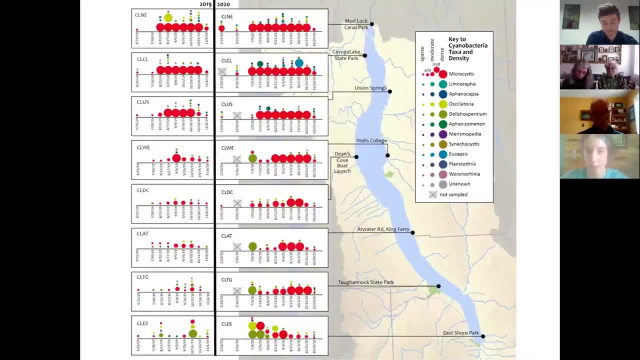 about harmful algal blooms and the cyanobacteria in our area that are causing them is that the cyanobacteria aren't out there in a vacuum. They're a natural part of our lake ecosystems. It's unusual perhaps that we're seeing around the world greater concentrations of these appearing in 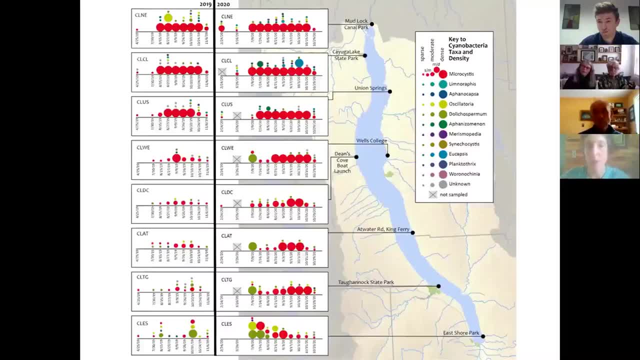 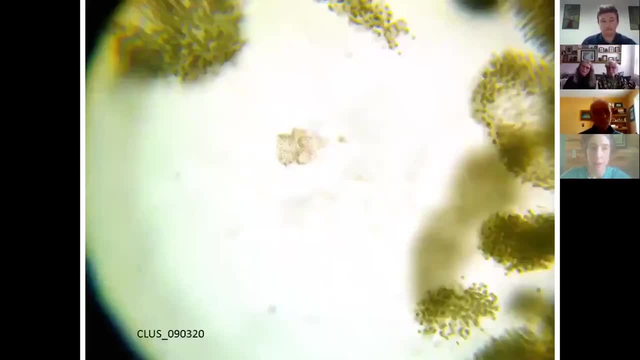 different areas, but it's not happening in a vacuum. There's a whole lot of other life out there and it's all connected one to the other, And I'm going to end with some photos of some other things that I've seen out there, just to remind us that you know, as we're thinking about harmful 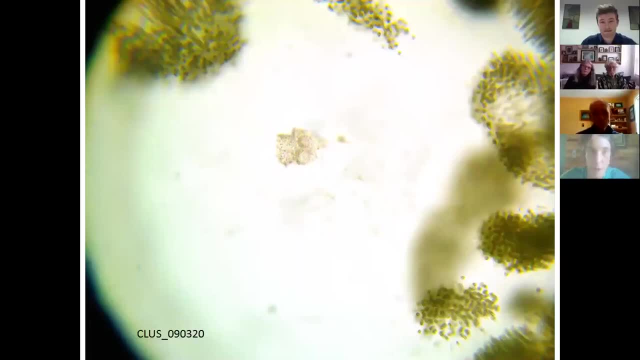 algal blooms that there's a whole lot going on out there in the lake, So microcystis around the outside. you might be looking under your slide at something like this and all of a sudden somebody like Caratella rotifer pops in. Here's a better photo image of them. They're really beautiful. 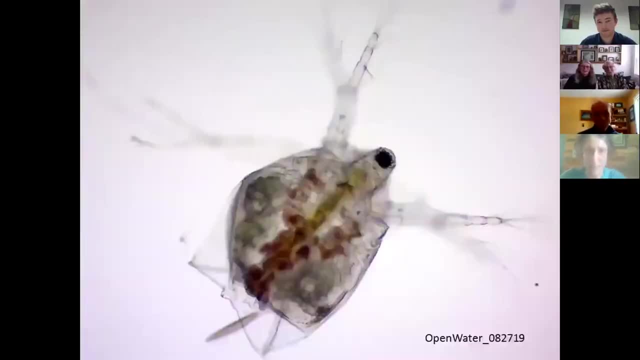 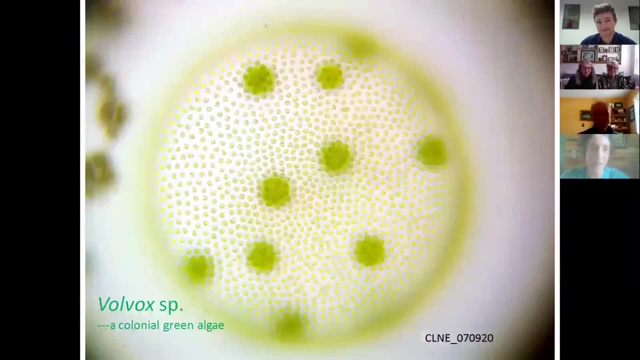 hard to photo Or something crazy like this. Here's a close-up of- yes, that actually is its eye- And volvox. these are kind of classic microorganisms that Van Leeuwenhoek, back in the 1700s, recorded him seeing under his early microscopes. They're a colonial green algae. 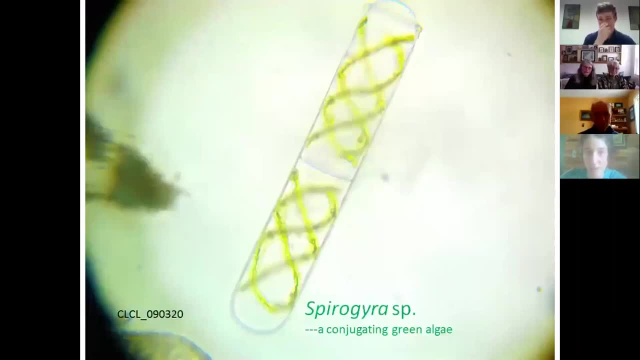 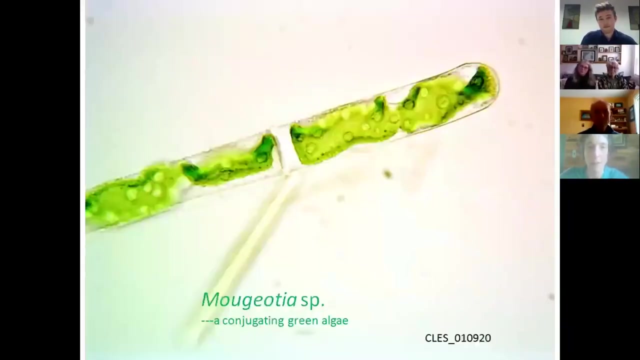 Or Spirogyra, which is a conjugating green algae. They have these spiral chloroplasts that go around the cells and they're actually ancestors. We've learned somewhat recently that these are ancestors of our land plants, plants And Moogotia also. they have these really cool. 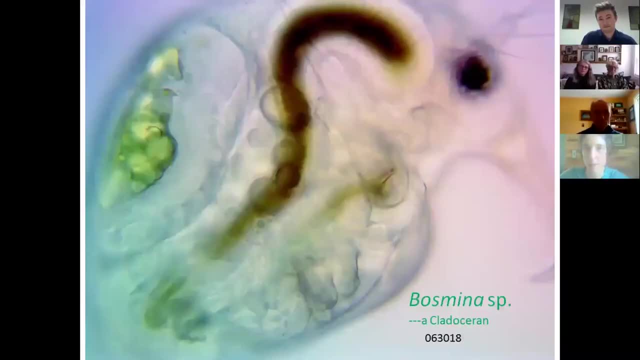 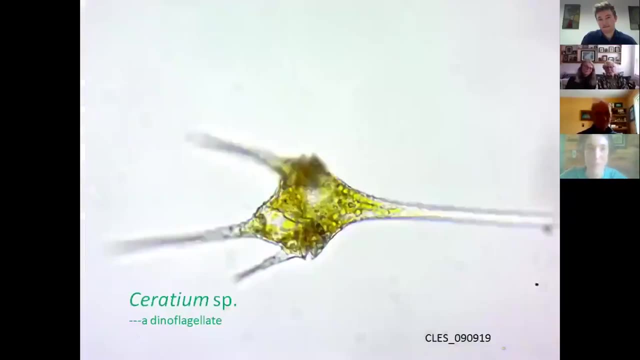 chloroplasts that are plate-like: Bosmina, who's kind of the charismatic mega-fauna of the micro world, really cool. Zooplankton, Serratium that photosynthesize and move. There are a lot of organisms like that. They not only do their work in the microplastic environment, they do it in the 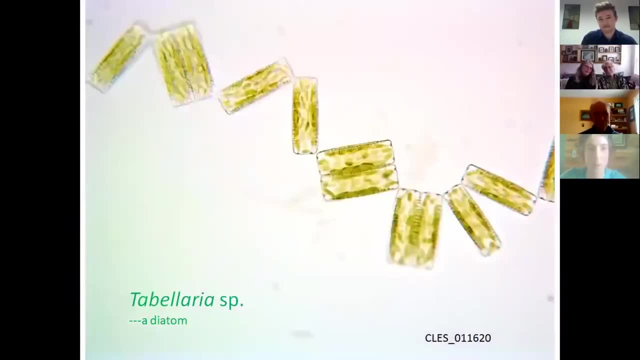 marine environment. They do a lot of things in the marine environment And there are a lot of photosynthesized, but they can eat things as well, And this diatoms which this tabularia is really beautiful. these are like little glass boxes made of silica. 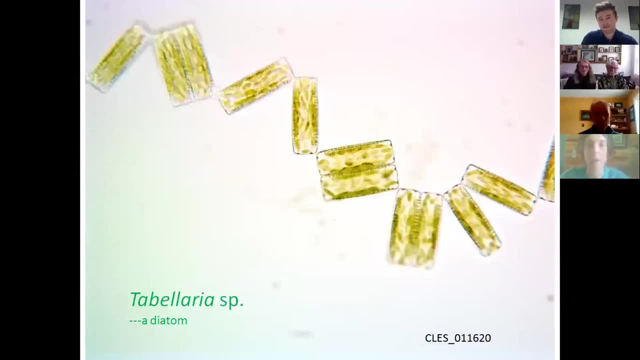 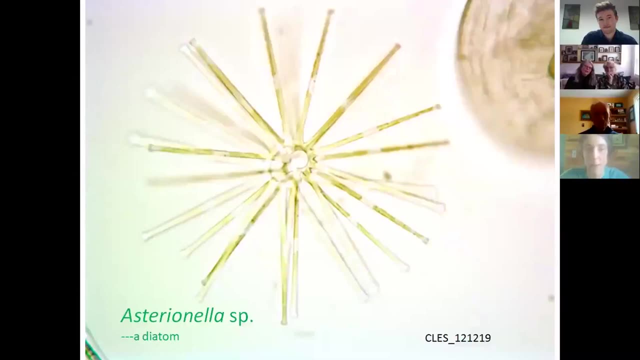 that are very common in the lake, especially in the winter, if you were to go out there right now. And lastly, Asterionella, another amazing diatom that's out there. I'm gonna leave you with this picture that hopefully I can. 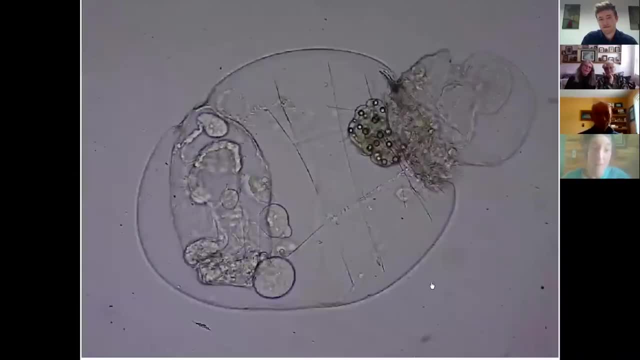 make become a video. This is a splanchnia, another rotifer. It was a rare occasion where it must have gotten trapped and it's damaged in some way, so I was actually able to look at it up close in one place for a while. just reminding us. 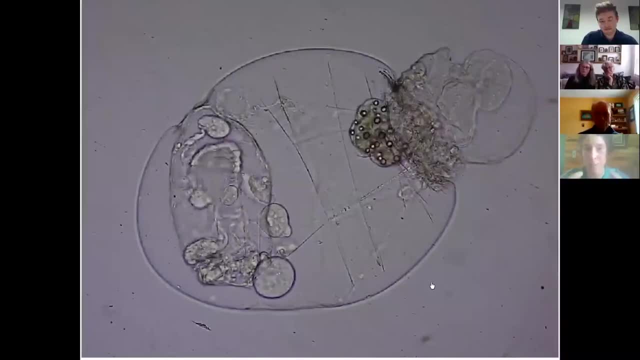 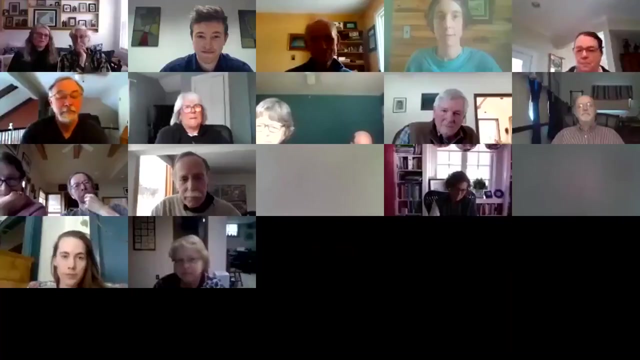 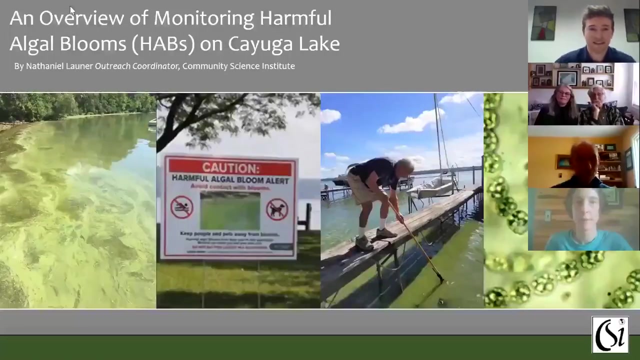 that that lake is a living organism itself, with all these living breathing parts of it. So thank you. I will turn it over to the next presenter. Great thank you, Adriana, And I also want to start by saying thank you to Shelly and. 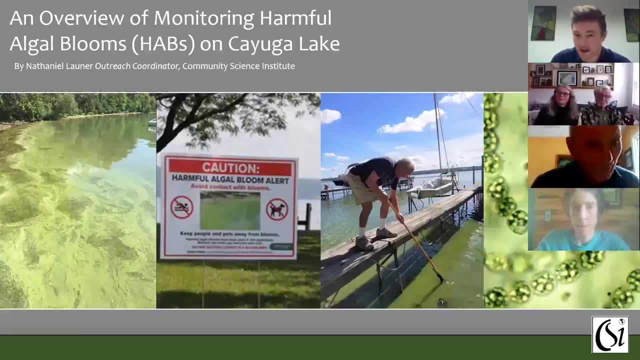 Sai and all of our other HABs Harrier volunteers, many of whom are with us today, without whom this program wouldn't be possible and who really make a huge contribution to helping monitor HABs And protecting Cayuga Lake. So today I'll be providing an overview of our 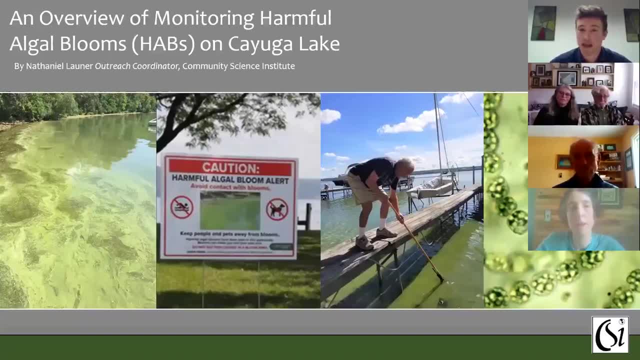 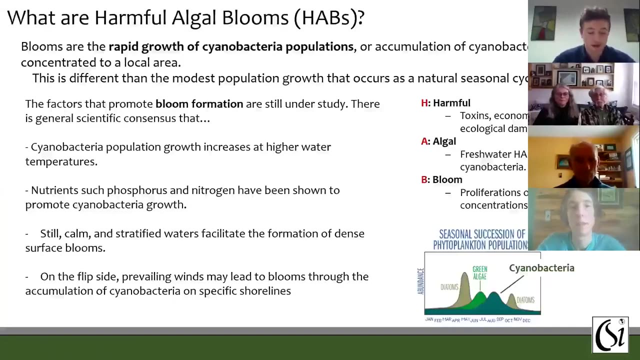 volunteer harmful algal bloom monitoring program and some of the results from our 2020 bloom monitoring program. So so far, we have discussed types of cyanobacteria found in Cayuga Lake and we have seen examples of what harmful algal blooms 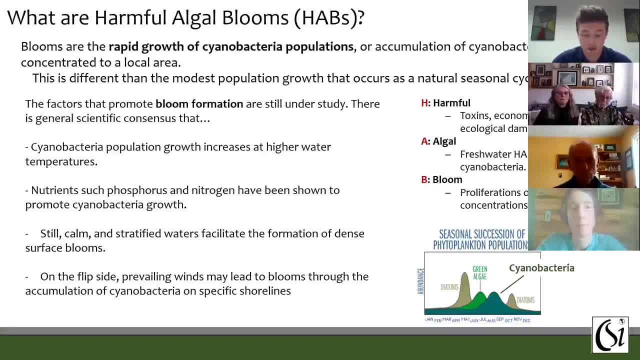 are and why they can be studied and how they can be used to protect our lake. And certainly not all phonemes have been so damaging and disruptive to lake shore homeowners. But what is a harmful algal bloom And it's hard to kind of. 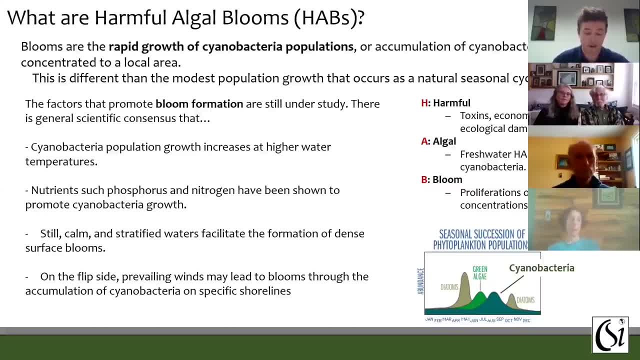 describe but harmful algal blooms are. HABs for short are the rapid growth of cyanobacteria populations or the accumulation of cyanobacteria concentrated to a local area. They can often look like pea green soup or surface scums. on the water, like those pictures that show on the screen. So if you go to the website and just look for the bottom right, the title of the slide list, As you can see, those are all. there are a few of them, Just take it a. 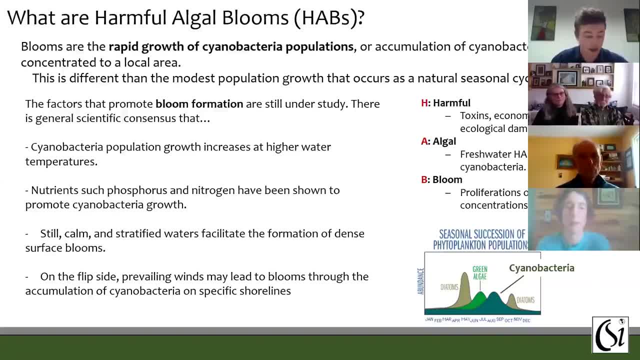 look at them and just find out what each one is talking about. So another thing that Shelly and Sai showed you, And this means that those intense blooms that was shown during their presentation are the result of the dense accumulation of the individual cyanobacteria. 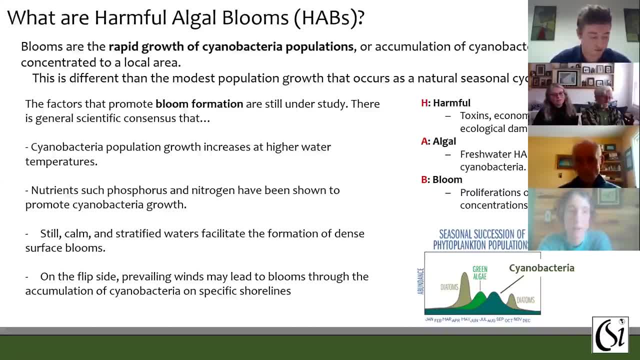 cells and colonies that Adriana was showing pictures of. Now these blooms are called harmful because cyanobacteria can produce toxins, as we've discussed, and those toxins can be present at high concentrations during these dense accumulations. They're also called harmful because they 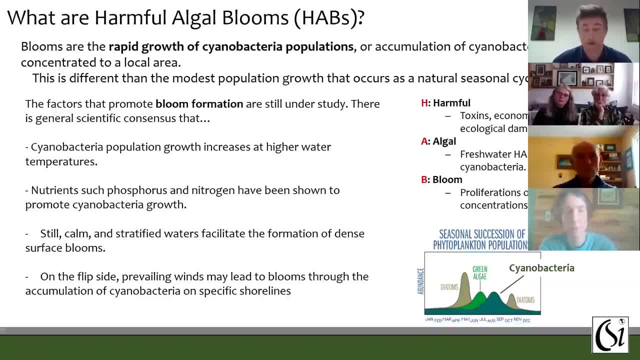 can damage the local economy by, for instance, disrupting tourism and recreation, and because they can cause ecological damage and disruption. Now, this rapid growth, or accumulation, is different than the modest growth that occurs as part of a natural seasonal cycle. Shown below is a simplified chart showing the 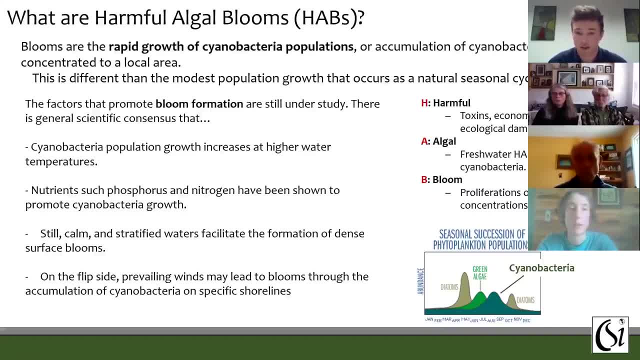 natural seasonal succession of phytoplankton populations, Including cyanobacteria, in freshwater lakes, throughout the year, And you can see that different types of phytoplankton, their population, naturally tends to increase throughout the year and that the population of cyanobacteria in a lake. 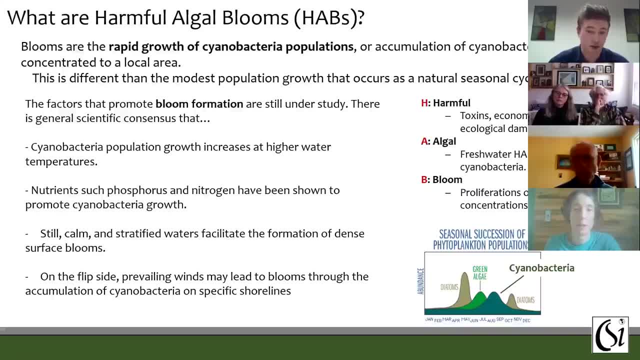 naturally tends to increase right around the summer months. But again, this natural increase in population in a lake is still far lower than kind of the spike in population or the dense accumulation of cyanobacteria That results in what we call a harmful algal bloom And the 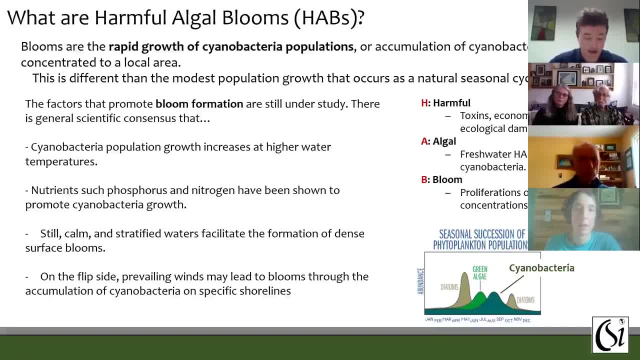 factors that promote these blooms are still under study and they can be numerous, But there is general scientific consensus that cyanobacteria population growth increases at higher water temperatures, that nutrients such as phosphorus and nitrogen have been shown to promote cyanobacteria growth And that's 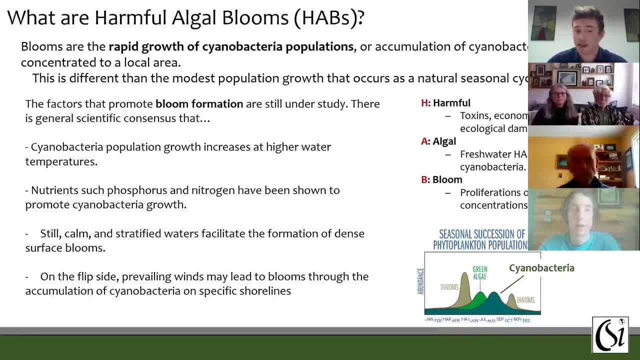 still calm and sustainable, And stratified waters tend to facilitate the formation of dense surface blooms. On the flip side of that, though, prevailing winds can sometimes lead to blooms because they cause cyanobacteria to accumulate on specific shorelines. So in 2017, there were many reports of harmful algal blooms. 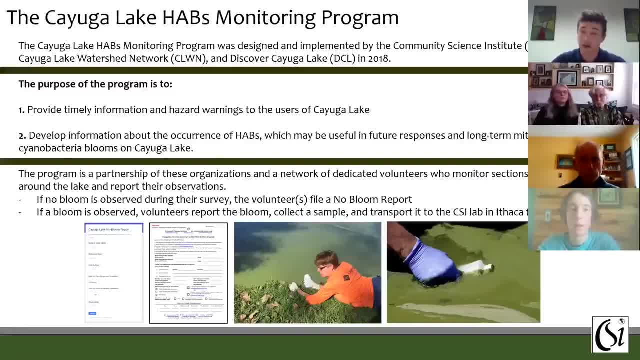 on Cayuga Lake, And this caused widespread concern about the health of the lake and the impacts that these blooms might be having. And, in response to this emerging water quality threat, the Community Science Institute implemented the Cayuga Lake Harmful Algal Bloom Monitoring Program, in collaboration with: 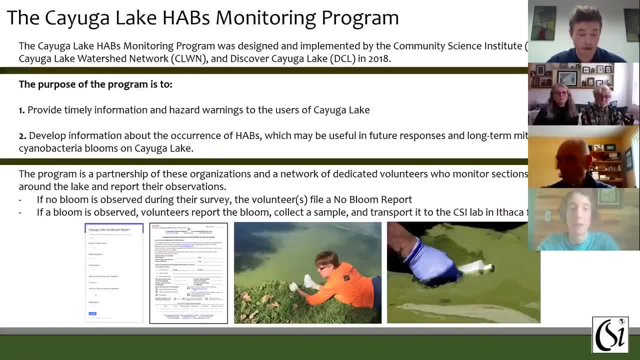 the Cayuga Lake Watershed Network and Discover Cayuga Lake Now. the purpose of the program is twofold. The program serves to provide fast alerts and hazard warnings to the users of Cayuga's waters, but also to develop information about the 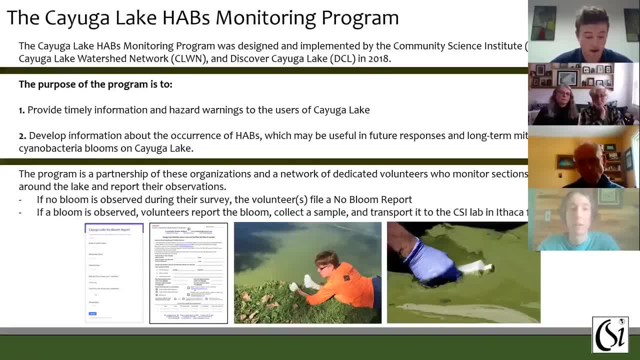 occurrence of harmful algal blooms. that might help us better understand their occurrence on Cayuga Lake in the future, And so the program is a partnership of these organizations and volunteers around the lake, And these volunteers, titled HABS Harriers, attend a two hour training. 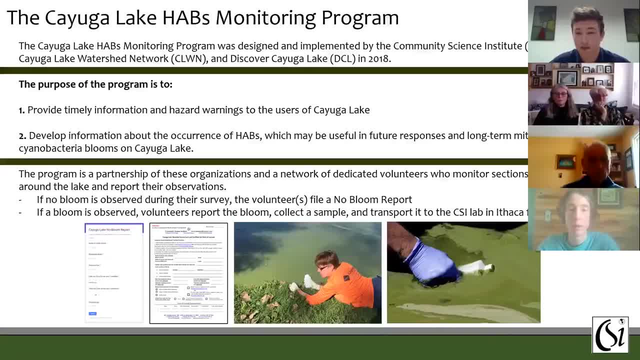 session in June where they learn how to identify harmful algal blooms and collect a sample, And then, following this, they monitor a section of shoreline on the lake once per week from the start of July until the end of September. If they don't observe a bloom during their weekly survey, they 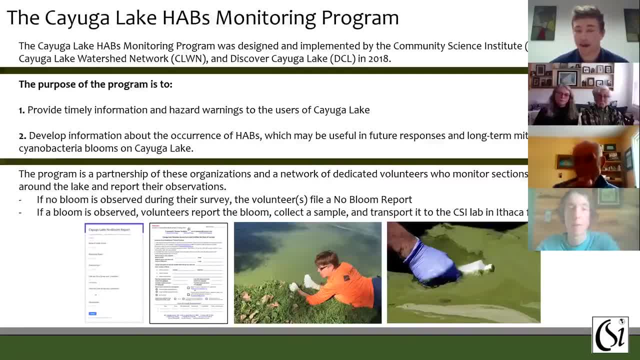 file what's called a no bloom report, signaling that the shoreline is clear of harmful algal blooms. However, if they do observe a bloom, they report the date, the time and the location immediately and also send pictures of the bloom, And then they also collect a sample of the bloom and transport it to. 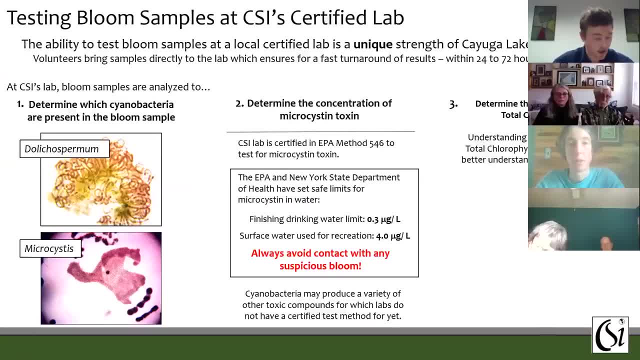 CSI Lab for analysis. Here at the lab, we test the bloom for to determine the type of cyanobacteria that formed the bloom, to measure the level of total chlorophyll A, which is a measure of bloom density, and to measure the concentration of microcystin toxin. Now, as many of you may know, microcystin 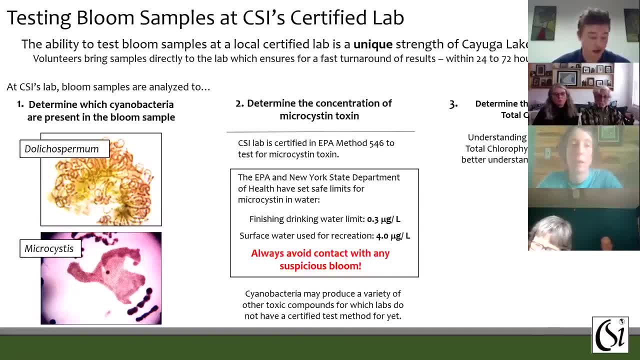 is considered to be the most common toxin associated with harmful algal blooms in New York State and one for which the Department of Health has set limits for safe recreation and finished drinking water. So the limit for microcystin in finished drinking water is 0.3 micrograms per liter and the 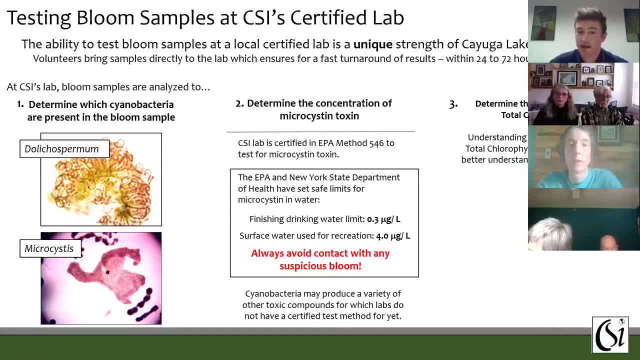 limit for microcystin in water used for recreation is 4 micrograms per liter, And it's really important to note that these limits are for water during non- bloom conditions, so you should never get exposed to an active bloom. Active blooms- 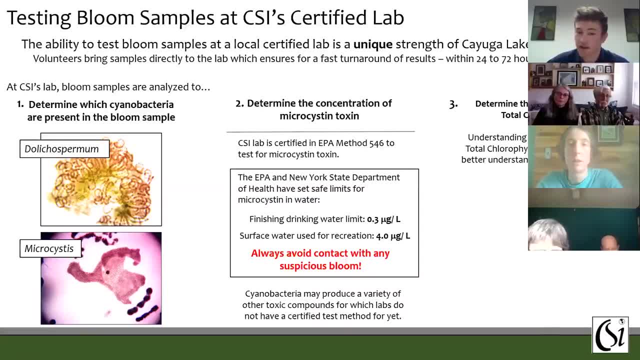 are always dangerous, regardless of whether you're using a microcystin or not, regardless of their microcystin concentration, because cyanobacteria are known to produce other toxins which we don't yet have an accurate and rapid way to test for. 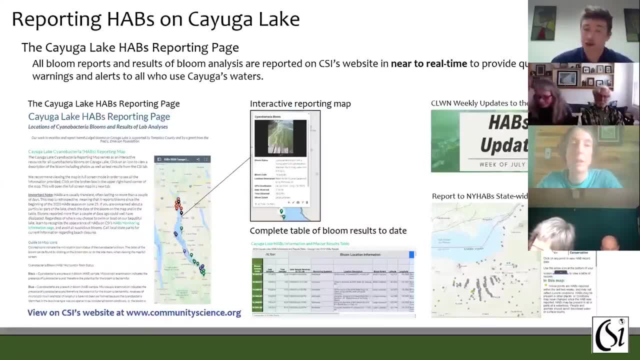 So once a bloom report is received at CSI, the description, the information provided by the volunteers, the photos and the location are posted on our Cayuga Lake HABS reporting page on our website in near to real time, And this page contains an interactive map. 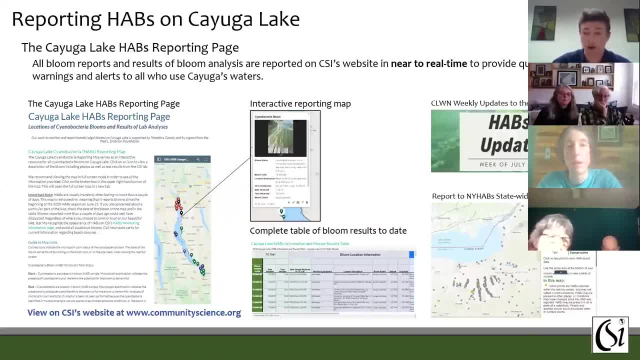 of the bloom locations and a table containing all of the information and the results of laboratory analysis. So the results of the analysis, including the microcystin toxin measurement, is posted on the page within 24 to 72 hours of receiving a bloom sample. 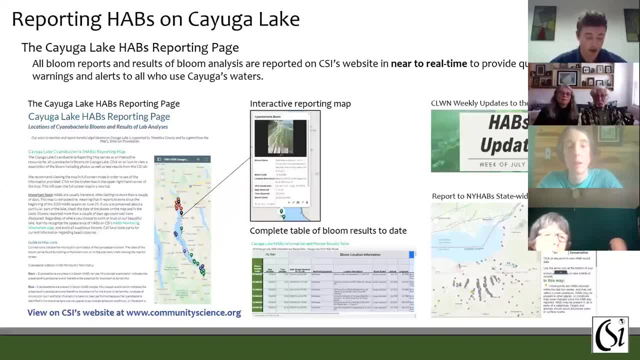 And this rapid turnaround is really important so that we can get accurate information to management, decision makers and the public alike, so that they can make safe decisions about recreating on the lake and using its waters, And then to further inform and alert communities around the lake about current. 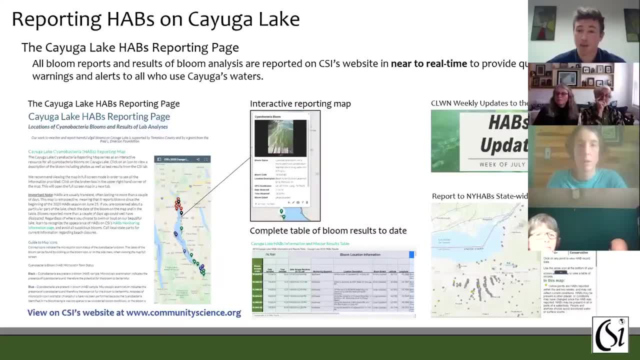 and recent harmful algal blooms. The Cayuga Lake Watershed Networks sends out weekly updates in which they include the most recent record of harmful algal blooms and the results lab analyses, and also some really useful information about local beach closures and anything else that you might need to know about the current status of harmful algal blooms on the. 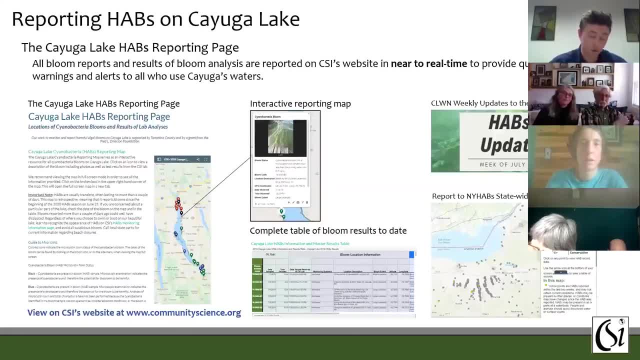 lake And, each week, bloom. data collected through our program is also sent to the New York State Department of Environmental Conservation and they post this data on their statewide NIHAB's reporting system so that people across the state and even across the country can be alert. 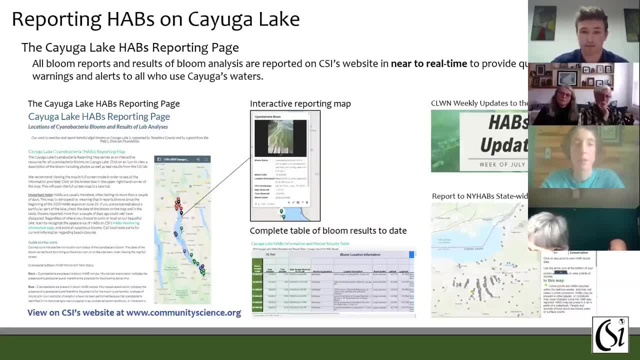 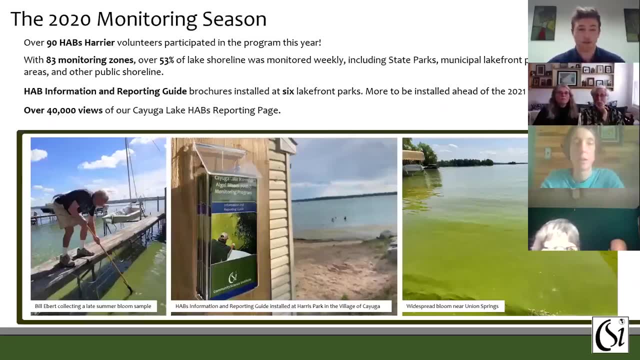 to when and where these blooms are happening. So over the past three years, our harmful algal blooms monitoring program has grown steadily. In 2020, over 90 volunteers participated in the program and they monitored 83 lakeshore zones. 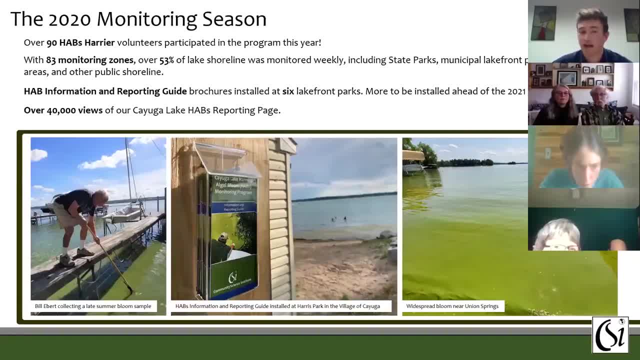 which covered roughly 50 percent of the entire lakeshore, On a weekly basis. This past summer, our Cayuga Lake HABS reporting page received over 40,000 views, which demonstrates that it is a widely used source of accurate information for harmful algal blooms on Cayuga. 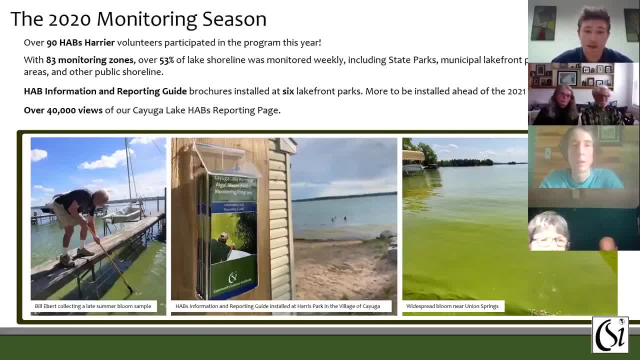 Lake, And further additions to the program this year include the publication of a Cayuga Lake Harmful Algal Bloom Information and Reporting Guide in the form of a brochure, and these brochures have been stocked in weatherproof holders at six lakefront parks so far. 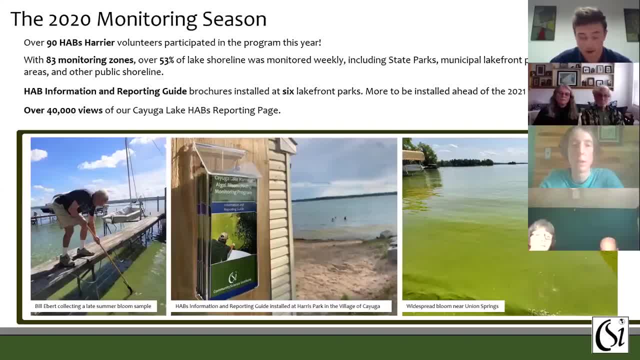 And we hope that these brochures will serve as an important outreach tool to inform lake goers about harmful algal blooms, how to recognize them and what to do if they encounter one. One additional thing that we included in the program this year was testing a select number of blooms. 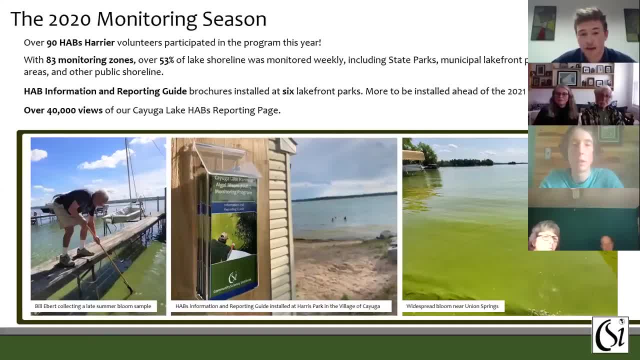 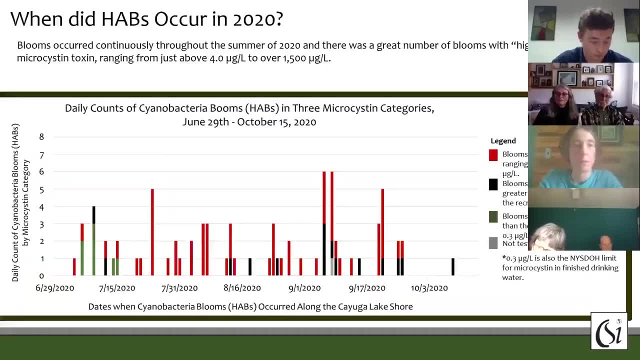 for anatoxin A And our technical director, NOAA Mark, will present on that following this presentation. So blooms in 2020 were frequent and intense. Shown here is a daily count of harmful algal blooms that occurred on Cayuga Lake during the 2020. 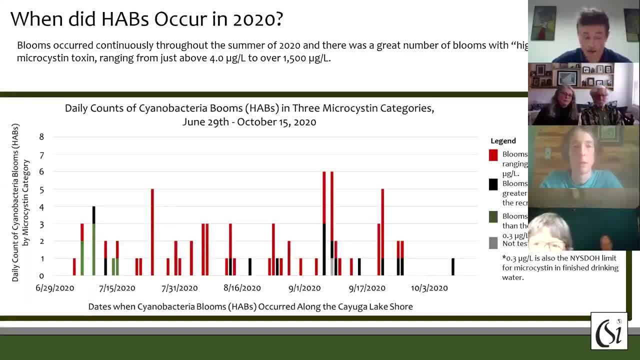 monitoring season, And in this chart, as in the ones to follow, we have classified the blooms by their microcystin toxin concentration. So gray represents blooms that we were not able to test for microcystin. Green represents blooms with a microcystin concentration below 0.3 micrograms per liter. Black represents 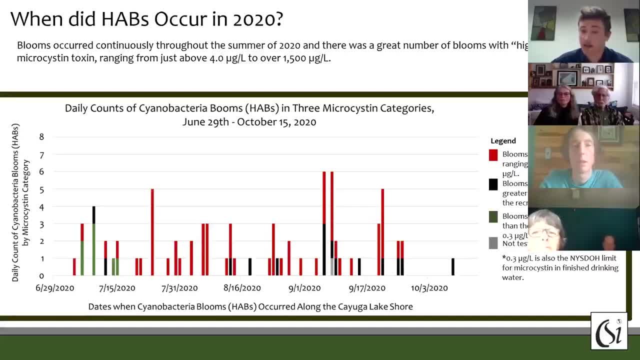 blooms with a microcystin concentration that exceeds 0.3 micrograms per liter but does not exceed the safe recreation limit for microcystin in water of 4 micrograms per liter. And red represents blooms with a microcystin. 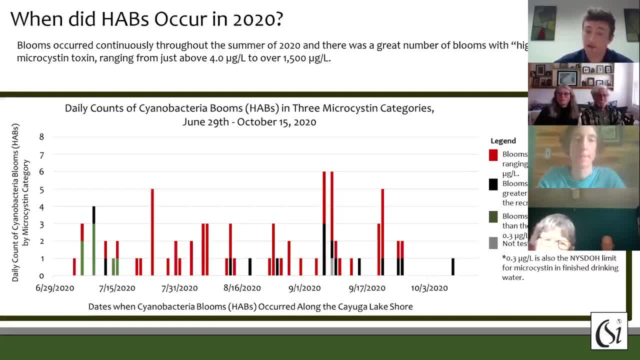 toxin level that exceeded the safe recreation limit of 4 micrograms per liter and, in some blooms, ranged as high as 1,500 micrograms per liter or 300 times that limit. And you can see here that blooms occurred continuously throughout the summer of 2020, and there were a great number of harmful algal 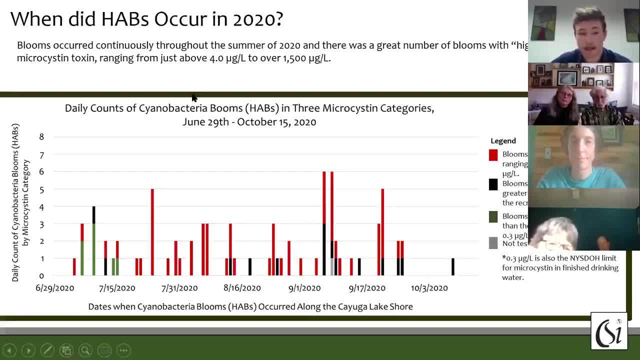 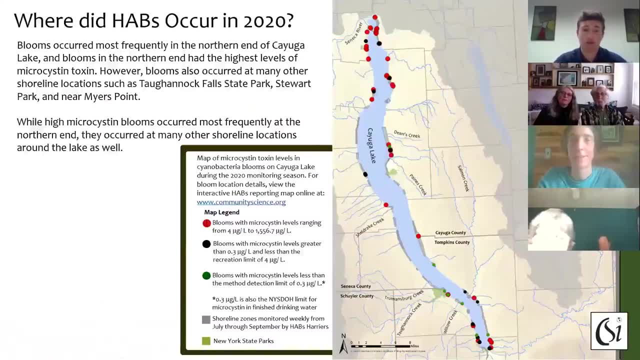 blooms with high levels of microcystin toxin, again shown by those red bars there. So where did blooms occur in 2020?? Well, shown here is a map of all 78 harmful algal blooms that occurred in 2020, and the color again represents their 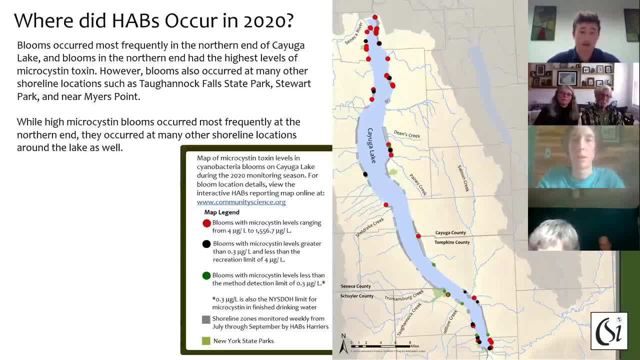 microcystin toxin concentration. So, as you can see, many high microcystin blooms occurred in the northern end of the lake, from roughly the area around Union Springs north to where Shelly and Sai monitor, all the way to the outlet at the 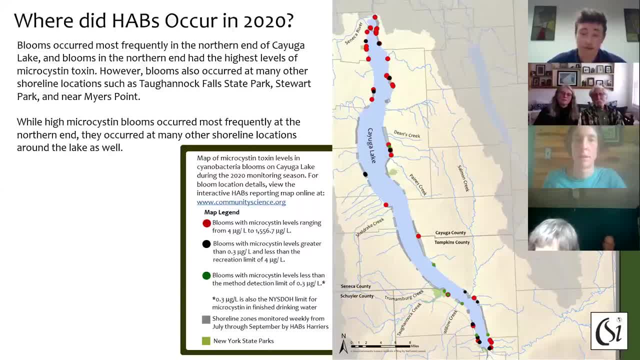 end of the lake. This section of the lake is where we observed most of the blooms and where the most blooms with high levels of microcystin toxin tended to occur. However, in 2020 we saw something interesting where blooms with high microcystin concentrations also occurred at many other lakeshore locations, such 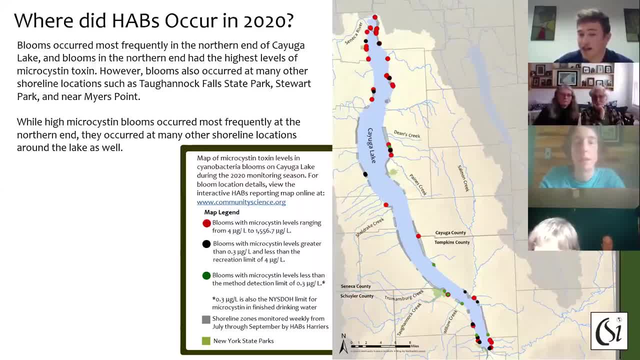 as on the shoreline of Stewart Park and East Shore Park down the coast of the Ithaca, As you can see by those red dots way down there at the southern end of the lake. So thank you, and I'll now turn it over to our technical director, Noah Mark, to talk. 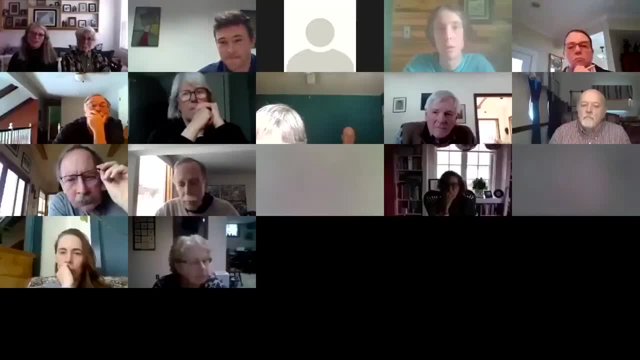 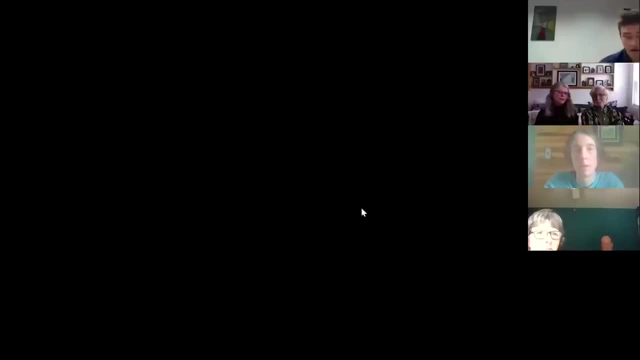 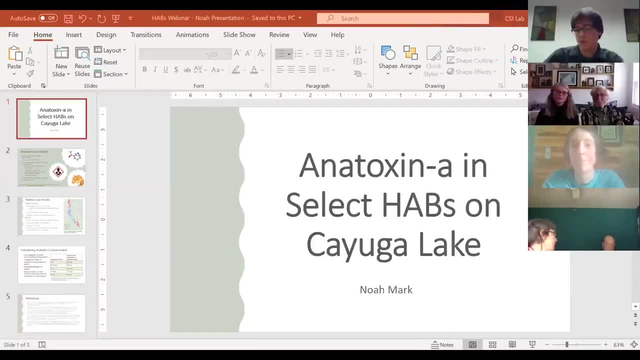 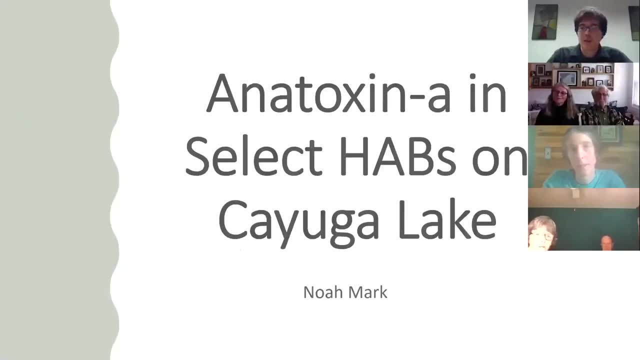 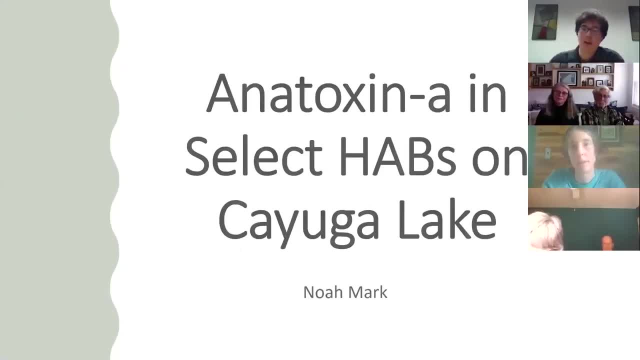 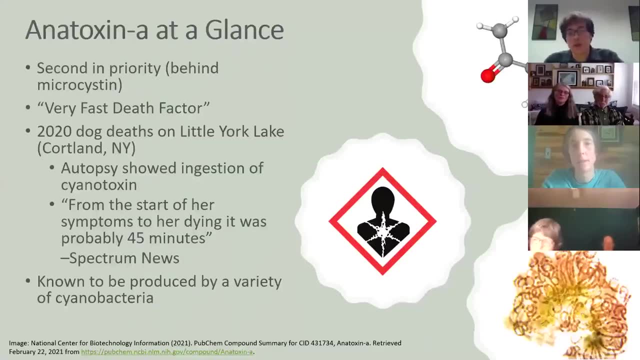 But today I'm here to talk to you about the anatoxin work we conducted last summer. So of the cyanotoxins that have been found in New York, microcystin tends to get the most attention, and rightfully so. It's been commonly found throughout water bodies in the 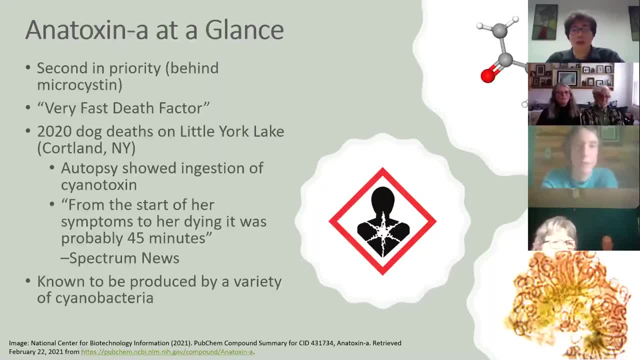 state and at alarmingly high concentrations. However, from a management standpoint, anatoxin A might be considered second in priority because of its association with animal deaths. In fact, before anatoxin A was called anatoxin A, it used to be referred to. 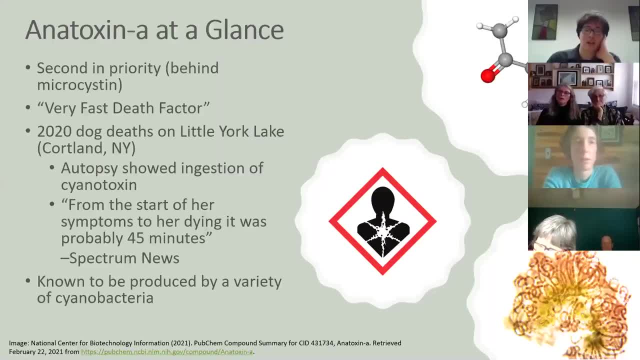 as a causing agent with very fast death factor. We may have seen this past June anatoxin A's deadly nature in action. There were two dog deaths that occurred on Little York Lake in Cortland. An autopsy of one of the dogs showed that she had ingested a cyanotoxin. I couldn't 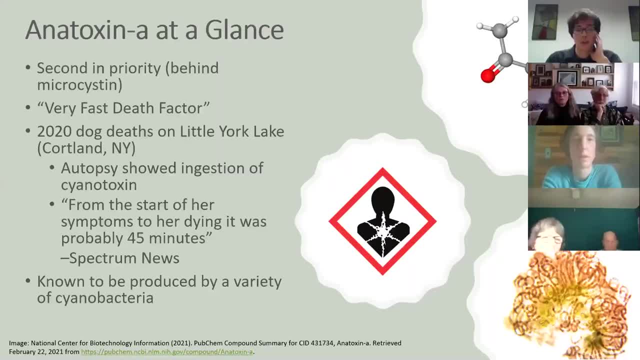 find specifically in the news which cyanotoxin, But from the owner's account the dog went into a seizure and then she unfortunately passed within about 45 minutes. So that seems reminiscent of livestock deaths that have been linked to anatoxin A contaminated waters, but again, we can't know for sure. Besides its deadly nature, 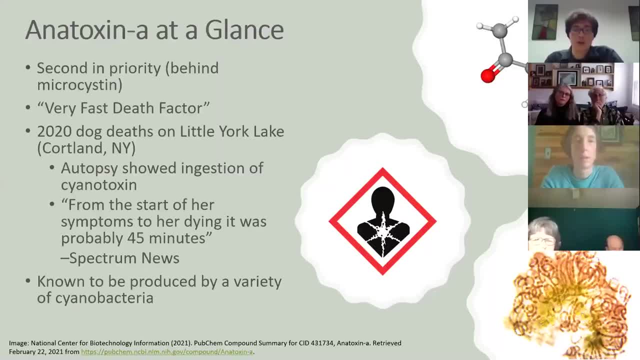 and it being a neurotoxin. another reason why CSI was interested in looking at anatoxin A is it's known to be produced by a radical A variety of cyanobacteria, including those that have dominated blooms on Cuyahoga Lake. 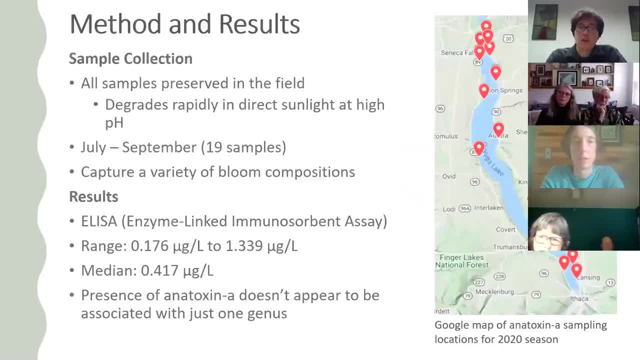 in our three years of monitoring. So one trait of this toxin is that it has a very short half-life and makes it difficult to sample, because it degrades very rapidly in direct sunlight and high pH, which are kind of the natural conditions that surface blooms are going to be exposed to. 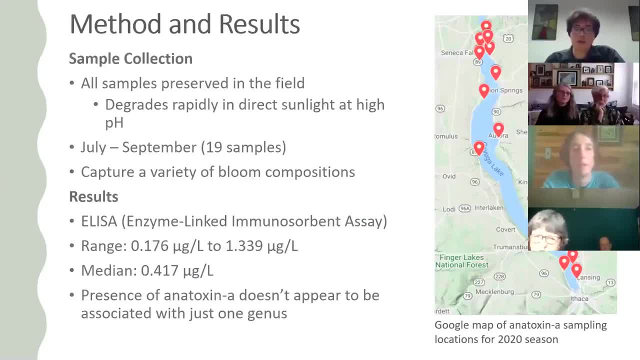 So we doled out our usual amber glass bottles that we give to our volunteers to collect HAB samples. but to select volunteers we gave them with a preservative that acts as an acidic microbial inhibitor, And so volunteers collected samples from July to September. We got 19. 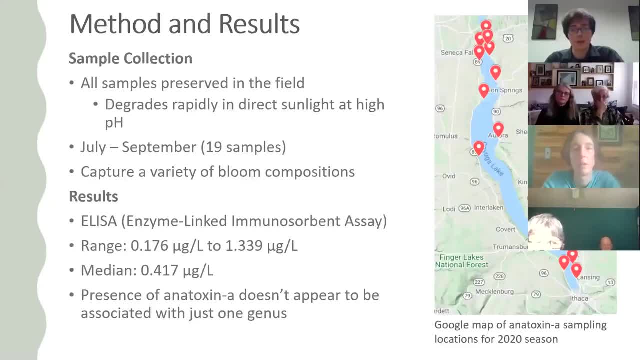 samples in total and we tried to capture a variety of bloom compositions and then look at whether there's any association with anatoxin A. So we tried to capture a variety of bloom compositions and then look at whether there's any association with anatoxin A and a single genus or genera. 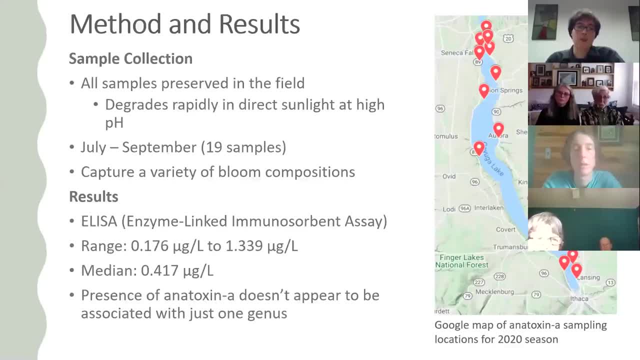 So, as far as testing goes, we used the same antibody based ELISA technology for anatoxin A that's used to test for microsystem. We got a range of about 0.1A to 1.3 micrograms per liter and a median of about 0.4 parts. 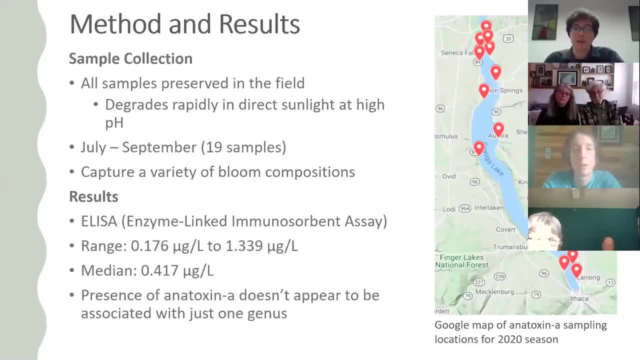 per billion or micrograms per liter. So looking at the microscopy analysis For these samples, the presence of anatoxin A doesn't appear to be associated with just one genus. We don't see that kind of tight correlation between toxin concentration and the presence. 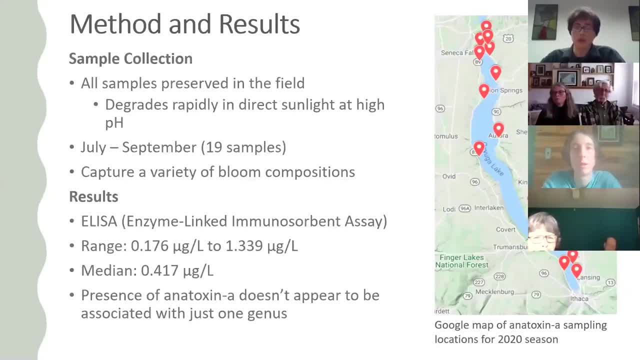 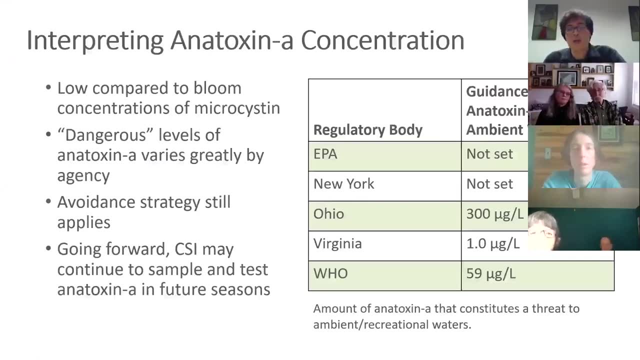 of, say, microcystis, like we do with microcystis and microcystin. So in looking at the concentrations that we got and trying to put it in context, we can certainly say that we saw low concentrations. Okay. 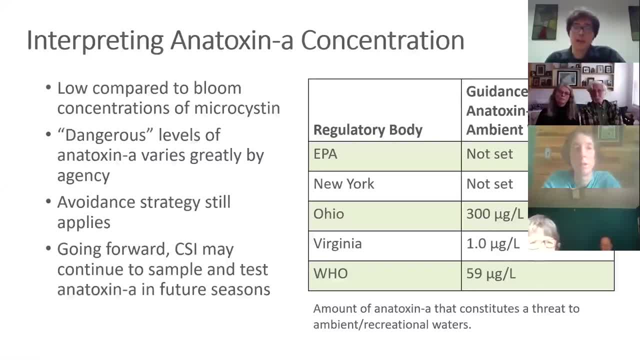 Compared to bloom concentrations of microcystin. However, when you get into what constitutes a dangerous level of anatoxin, it really depends on who you ask. Currently, the EPA and New York State don't have guidance on anatoxin in ambient water. 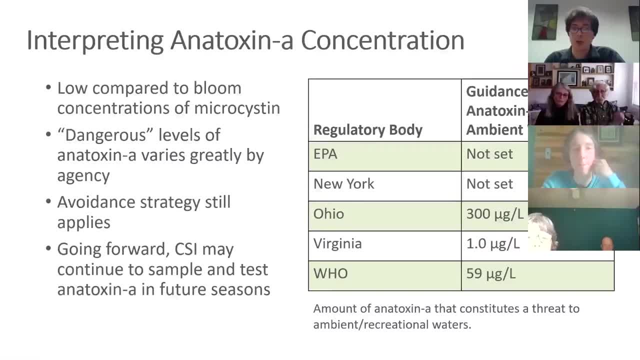 And then individual states like Ohio and Virginia. they can vary greatly on what poses a threat to recreational waters. So, because of the uncertainty, The avoidance strategy prescribed by the state when encountering a suspicious bloom still applies. Like we don't fully know what could be there. 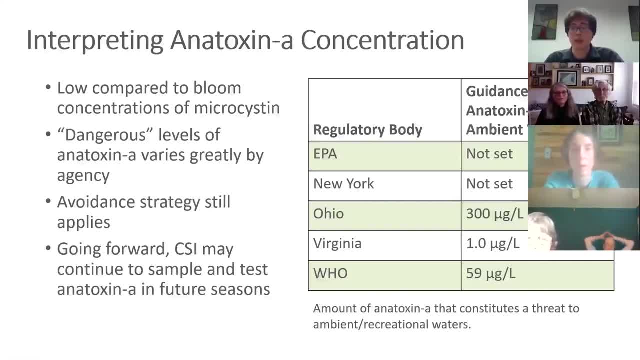 Even if a bloom, say, tests low for a microcystin, there could be another cyanotoxin present And going forward. CSI may continue to sample and test for anatoxin A in the future. It's partly commensurate with funding and interest, but I'll just leave it at that for. 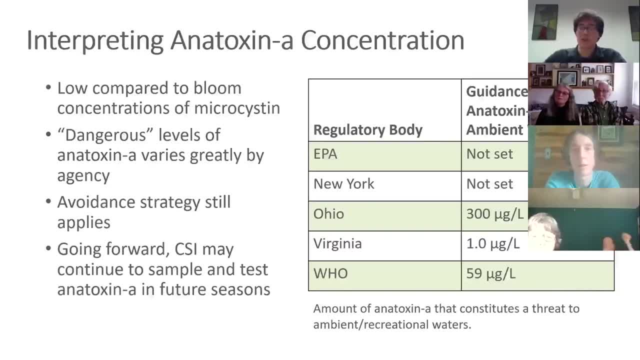 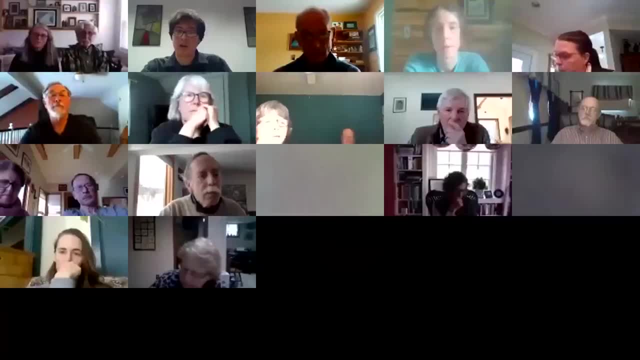 now, And I'll pass the baton to Steve. Who's going to talk about that? Let's talk about three-year trends. Okay, Thank you, Noah. I'm going to try my hand at screen sharing. Let's see. Here we go. 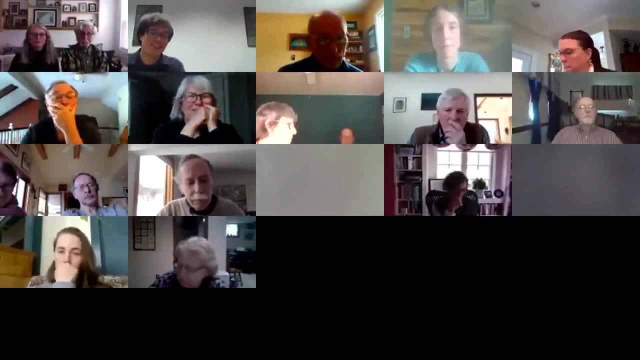 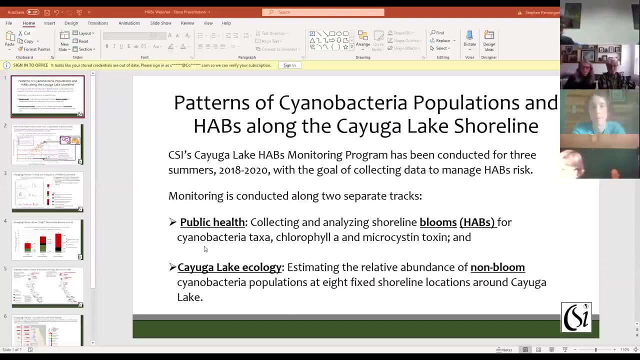 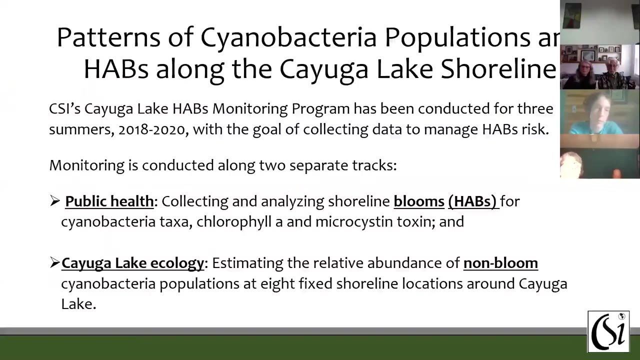 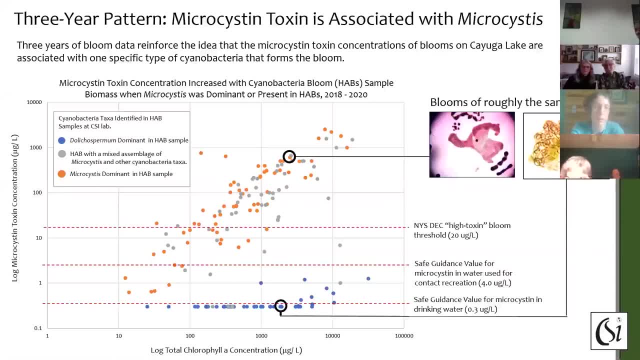 Okay, I would like to talk about and wrap up today's presentations by talking about some of the patterns that we've observed in the three years that we've been monitoring HABs on Cayuga Lake. So the first pattern has already been mentioned. 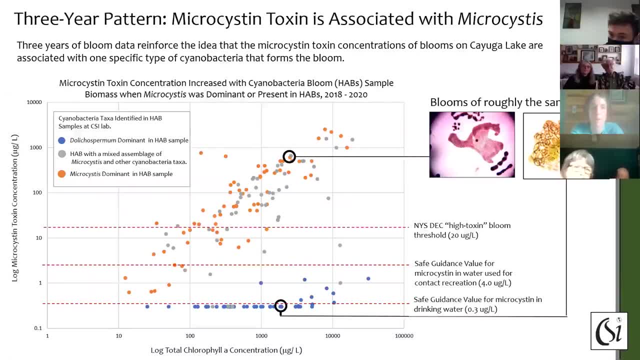 I'll just make it a little more explicit. The concentration of microcystin toxin in a harmful algal bloom is correlated with the presence of one particular type of cell, particular type of cyanobacteria called Microcystis, And on this graph the dots represent. 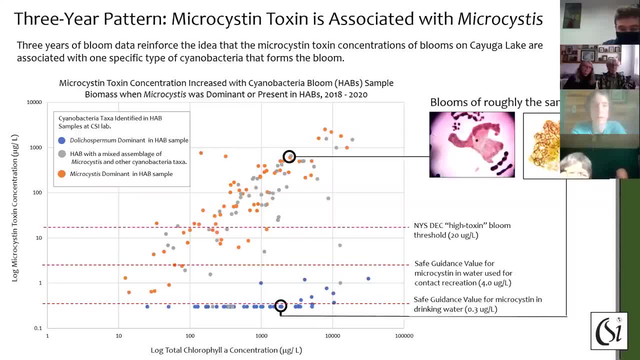 Cayuga Lake HAB samples from the last three years, And the orange dots are samples that are dominated by, or were dominated by, Microcystis and you can see that familiar image there. to the right, The blue dots are dominated by Dolichospermum, with little or no Microcystis and an image. 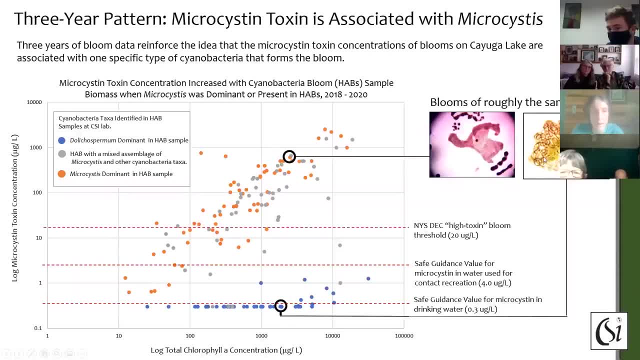 of that is here. you saw that earlier in Adriana's talk- and gray dots represent mixed assemblages of cyanobacteria that include Microcystis. So on the x-axis is the concentration of total chlorophyll A, which is a measure of balloon density, and on the y-axis is the 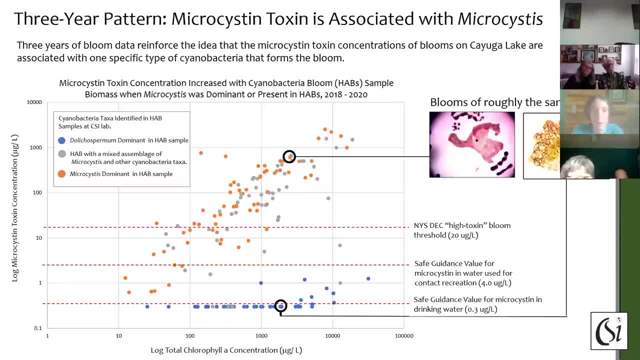 concentration of protein-based chlorophyll and, on the x-axis, is the concentration of concentration of microcystin toxin And, as you can see, the denser the bloom, generally speaking, the higher the concentration of microcystin toxin if the bloom contains microcystis. In other words, 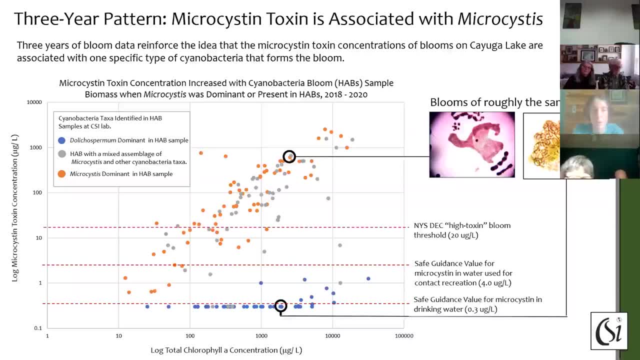 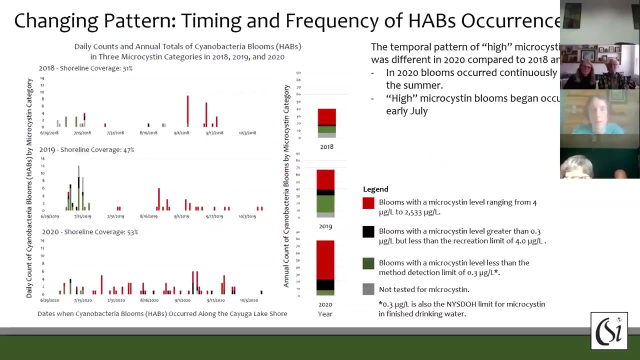 if it's a gray dot or an orange dot, But blooms that do not contain microcystis, like the dolichosperm blooms shown by the blue dots, also contain little or no microcystin toxin. The second pattern that we've noticed has to do with the frequency of HABs occurrences and their 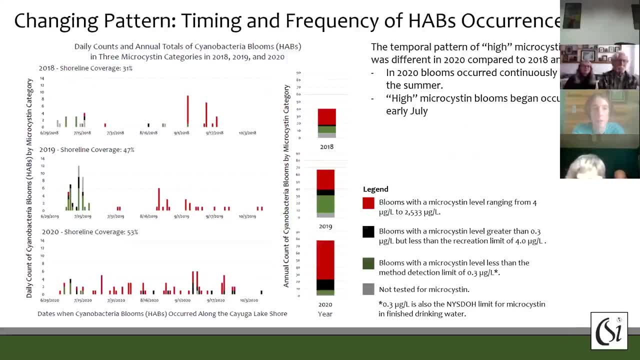 timing during the season. Nate described the timing and frequency in 2020.. And I would like to go back a couple of years and review the frequency and timing in 2018 and 2019.. And that is shown in the graphs on the left, which 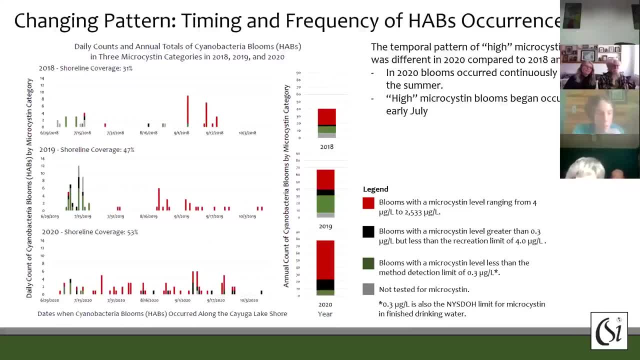 show the daily counts of HABs in each year, 2018,, 2019, and 2020, with the date on the x-axis and the number of HABs on the y-axis, And the harmful algal blooms are color-coded. 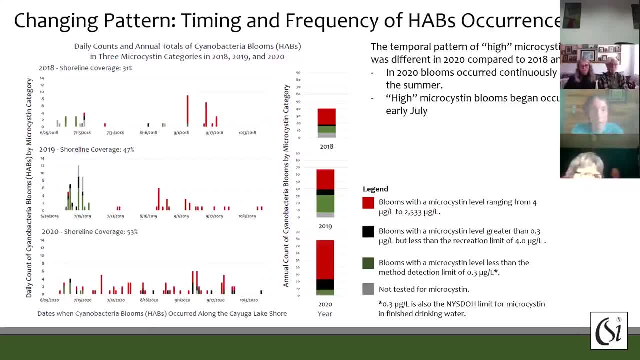 as has been described previously, with gray, not tested. green, less than the drinking water limit: 0.3 micrograms per liter. black, between 0.3 and 4 micrograms. blue, to the recreation limit and red above the recreation limit of 4 micrograms per liter. 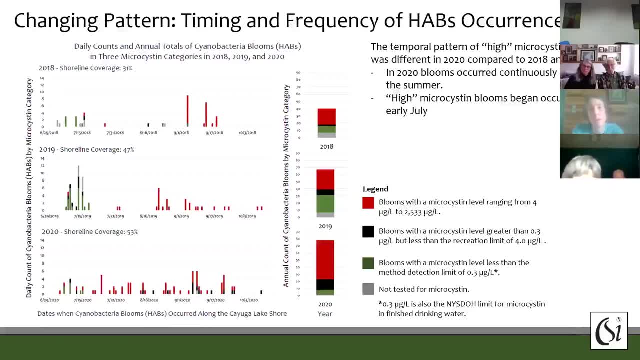 And some of the microcystin concentrations were as high as 2,500 micrograms per liter, that which is about 600 times the recreation limit. So, as you can see from the graphs on the left, 0.3 micrograms per liter. the recreation limit is about 2,500 micrograms per liter. Almost all of the 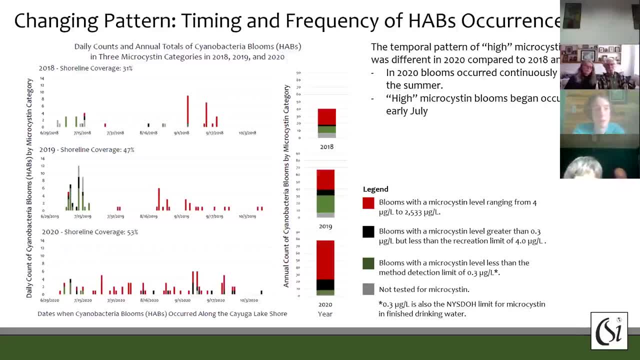 biology courses The late season. HABs in 2018 or 2019 contain microcystin above four micrograms per liter and that is- and that is- a result of 2018 and 2019, there were three general phases of HABs. 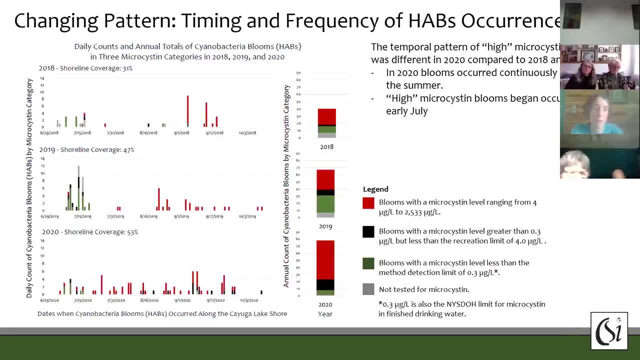 occurrence, There was an abundance of elementary habes in July, a lull in the期 of several weeks and therefore a late July and August, and then an increase, as I mentioned, in HABs in late August and September and there were only a very few of the early season HABs that contained microcystin greater than four. 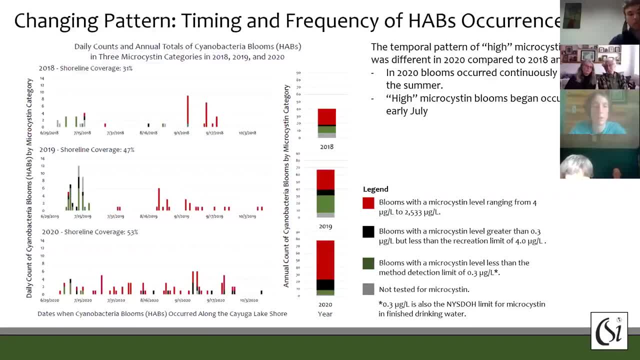 micrograms per liter, which is the recreation limit. But in 2018 and 2019,, as I mentioned, virtually all of the late season HABs contained microcystin greater than four micrograms per liter. But now look at the bottom graph: the pattern in 2020.. It changed and we saw. 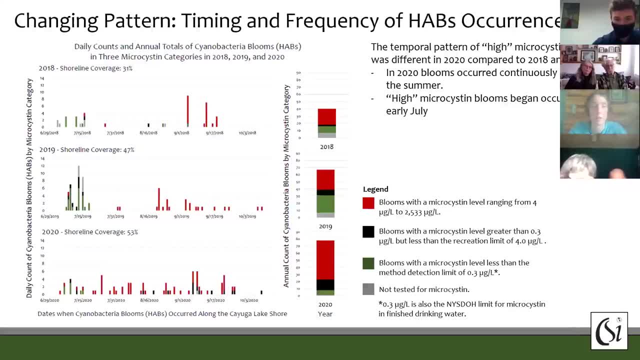 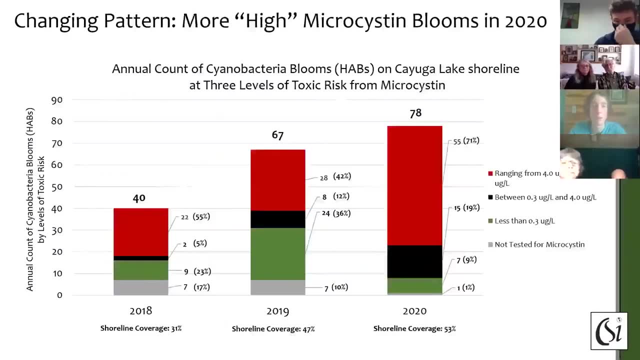 high microcystin HABs throughout the season from July to September. Another pattern that changed is the number of high microcystin HABs. This graph shows the number of blooms in each microcystin category in 2018,, 2019, and 2020.. 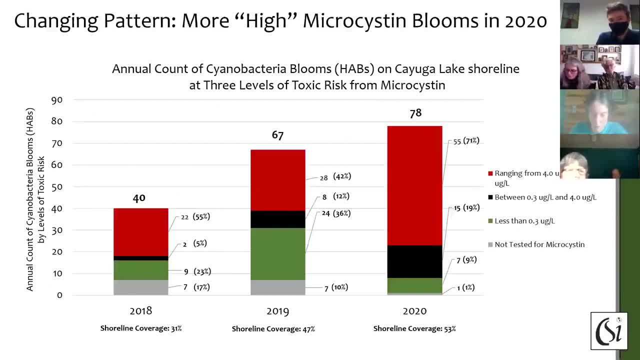 As you can see, in 2018 there were 22 high microcystin blooms, in 2019 there were 28, and in 2020 there were 55,, which is almost twice as many as 2019 and 2018.. 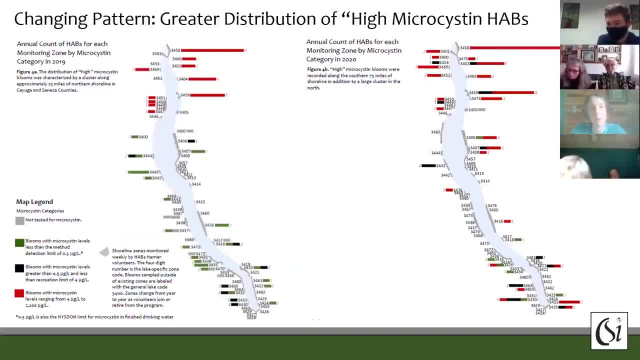 Another change in 2020 was in the distribution of high microcystin HABs around Cayuga Lake, And the images on the map in this figure show the zones in gray that were controlled by HABs, HAERIER volunteers and the number of each zone. The horizontal bars indicate. 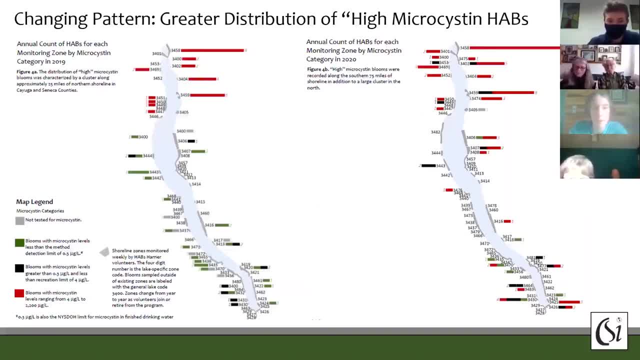 the number of harmful algal bloom samples that were analyzed in each zone and their microcystin levels again are color coded. It's really interesting to see how it has changed in 2020.. So in 2019, and also in 2018, it's not shown high microcystin HABs were clustered along. the northern roughly 20% of the shoreline. In 2020, this northern cluster was observed again, but in addition, high microcystin HABs were found along the southern roughly 80% of the Cayuga Lake shoreline, including Stewart. 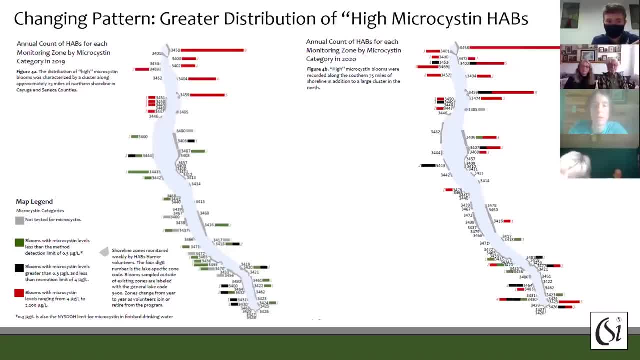 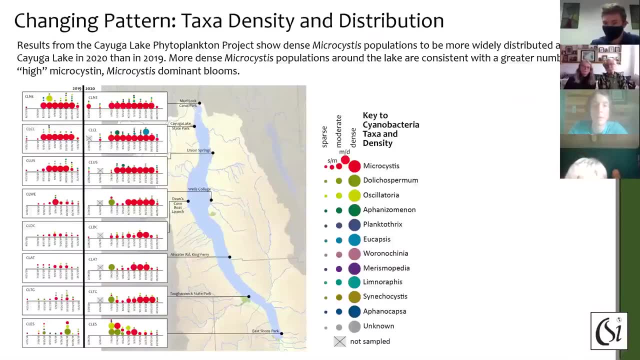 Park and East Shore Park in Ithaca. You already saw this slide in Adriana's talk. It's from the ecological track of our Cayuga Lake HABs monitoring program and it shows that under non-bloom conditions, populations of microcystis become more dominant became. 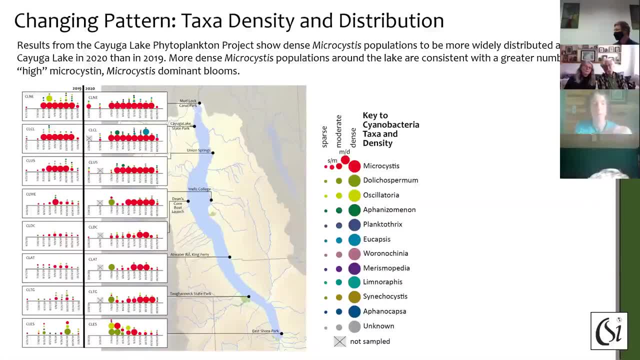 more dominant In the southern 80% Of the lake shore in 2020 compared to 2019.. So this suggests the correlation between the greater distribution, or the more widespread distribution, of high microcystin blooms in 2020 and the greater distribution of dense. 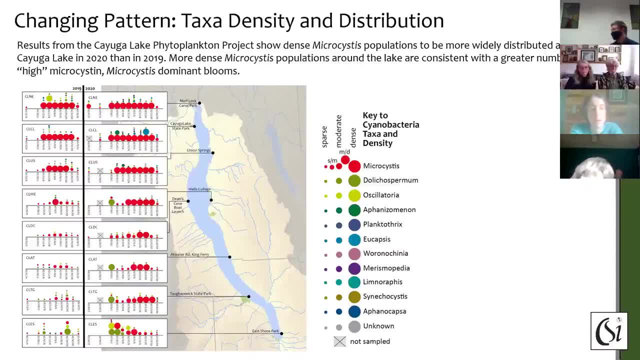 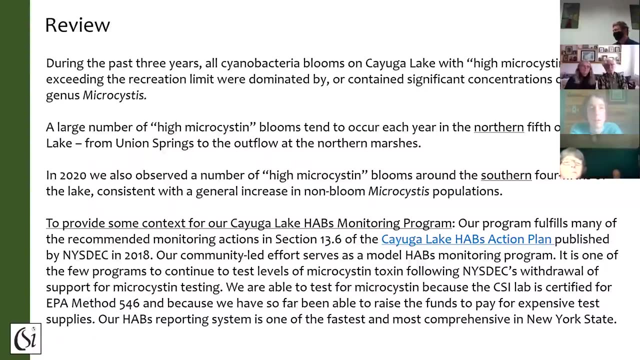 non-bloom microcystis populations around the lake. But, to be clear, this is a correlation. It's only a correlation. We can't say whether there is a cause and effect relationship. Okay, So, to review, during the past three years, virtually all of the cyanobacteria blooms. 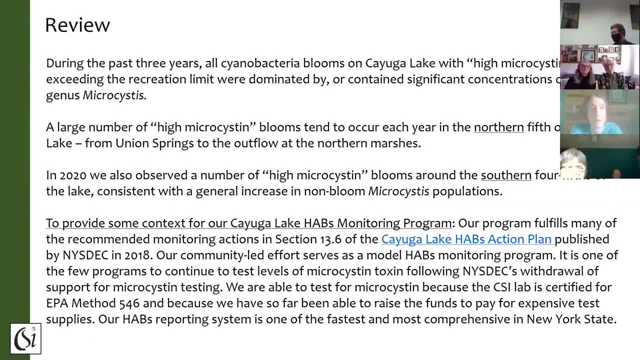 on Cayuga Lake with high microcystin exceeding the recreation limit were dominated by or contained significant concentrations of the genus microcystis. A large number of high microcystin blooms tend to occur each year in the northern fifth of Cayuga Lake, from Union Springs to the outflow with the northern marshes. 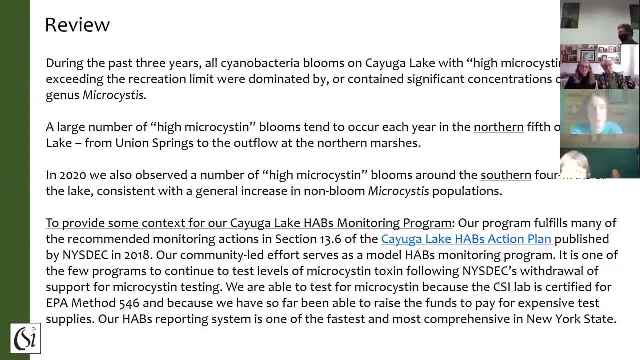 In 2020,. however, we also observed a number of high microcystin blooms around the southern four-fifths of the lake, which is consistent with a general increase in non-bloom microcystis populations. So, in closing, I'd just like to provide some context for our Cayuga Lake HABs monitoring. 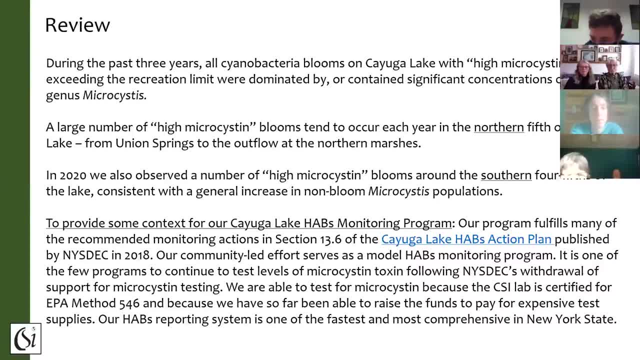 program. I believe Nate already touched on this. Our program fulfills many of the recommended actions in the Cayuga Lake HABs action plan published by DEC in 2018.. Our community-led effort serves as a model really of HABs monitoring. 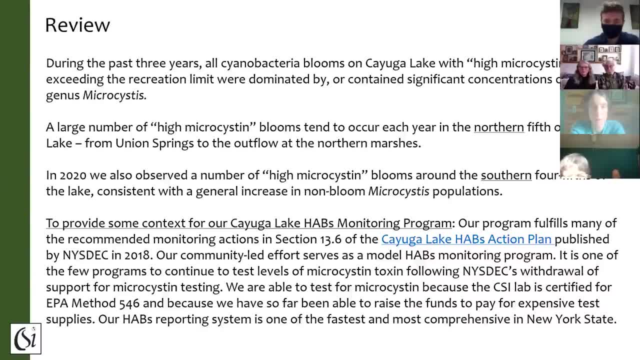 It's one of the few programs that continues to test levels of microcystin toxin following the DEC's withdrawal of support financial support for microcystin testing. We are able to test for microcystin because, as Nate and Noah mentioned, the CSI lab is. 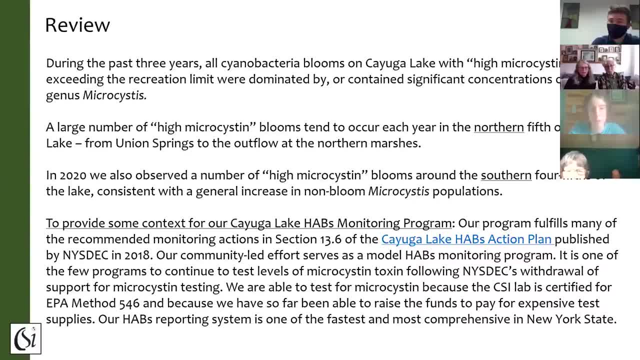 certified for EPA Method 546, and because so far we've been able to raise enough money to do it. the tests are expensive And, finally, we're proud of our HABs reporting system. We think it's one of the fastest and most comprehensive in New York State. 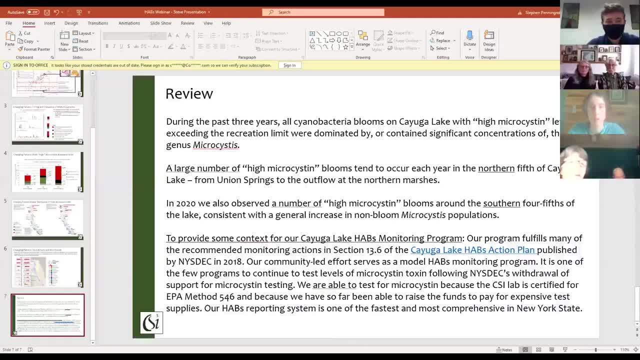 So with that, I'd like to turn it back over to Nate Great. Thank you, Steve. So now we'll open it up to a discussion section, and we will start that by asking upon some of the folks who have asked questions so far to unmute themselves and read their 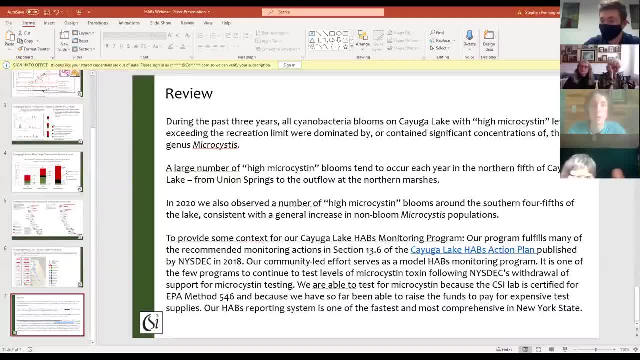 question aloud if they would like to. If they would like me to read their question, I'm happy to do so. So Jim Long asked a question. Jim, if you'd like to unmute yourself and ask it, that would be great. 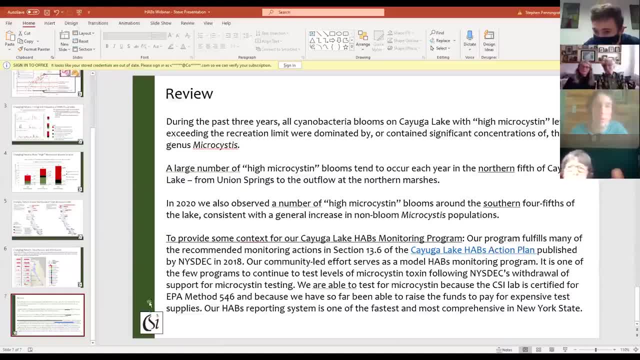 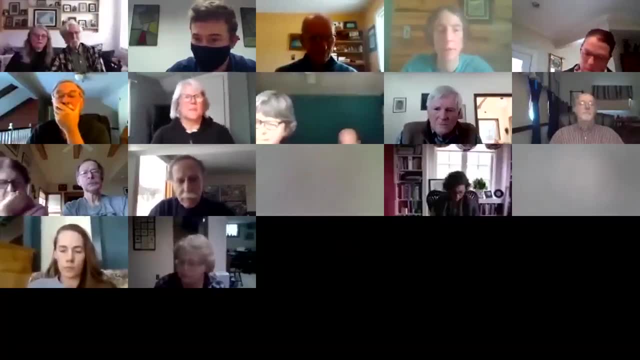 Hey, Nate, can you stop the screen share, maybe? Sure, Yeah, that'd be great, Thank you. Thank you, Adriana. You still here, You still All right? well, I'll just I'll ask it right now. 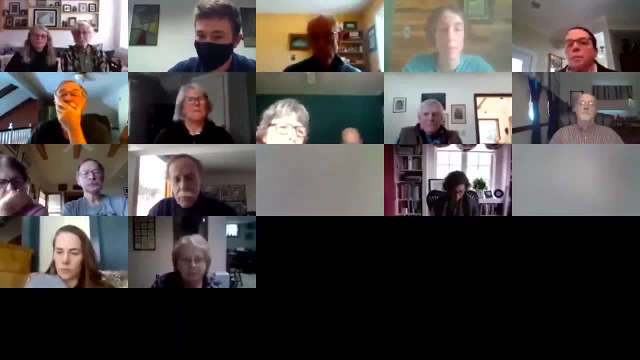 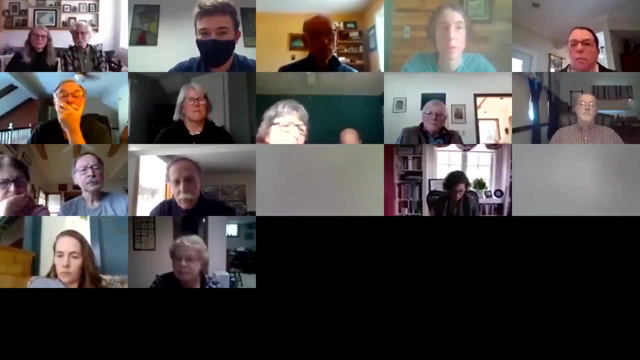 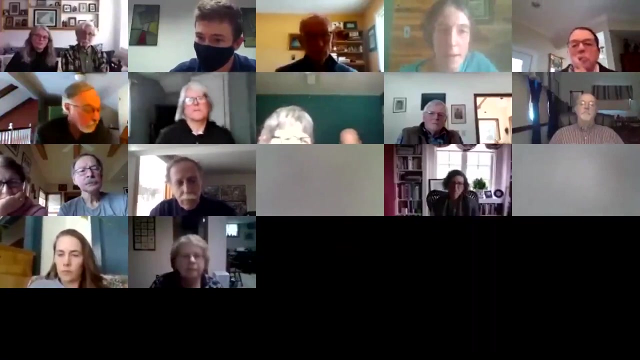 This one might be a good one for Adriana. Jim wrote: can anyone say something about the bloom that lasted many weeks? Yeah, there was a big bloom there for quite a while and I a lot of times when we looked at what was happening over there it wasn't necessarily cyanobacteria, but I think sometimes 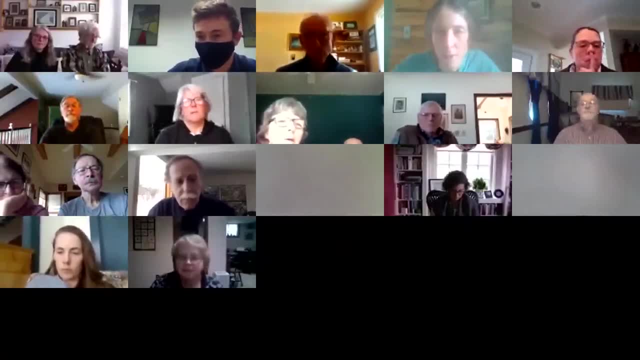 it was, And I'm sorry that I don't have my notes right here to look into that, but there were a lot of Euglena too at different times. Yeah, Yeah, Yeah, So it wasn't always cyanobacteria, but it looked pretty gnarly over there. 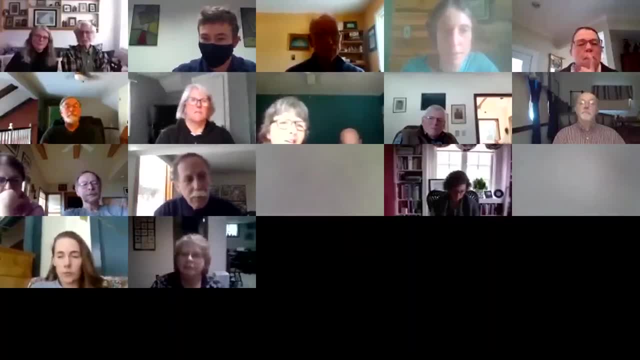 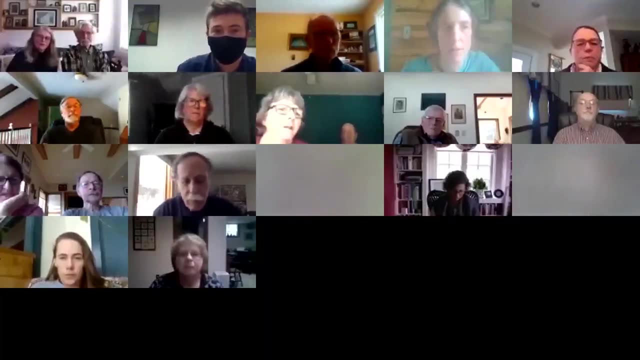 And yeah, sorry, does anyone else have anything else on that? Did we test any of those samples? Do you remember, Nate? Yeah, so we ended up testing one of the samples from the Stewart Park pond. You know, while it's not a lake sample from Cayuga Lake, we were just interested to see. 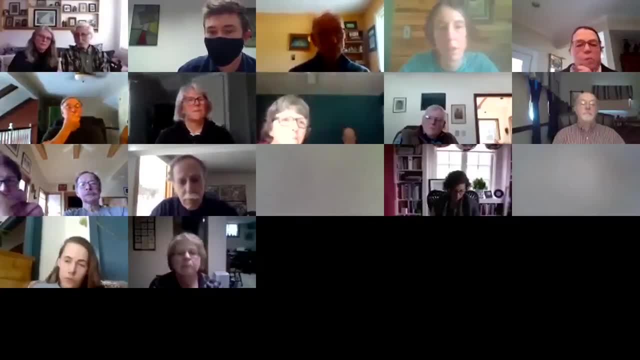 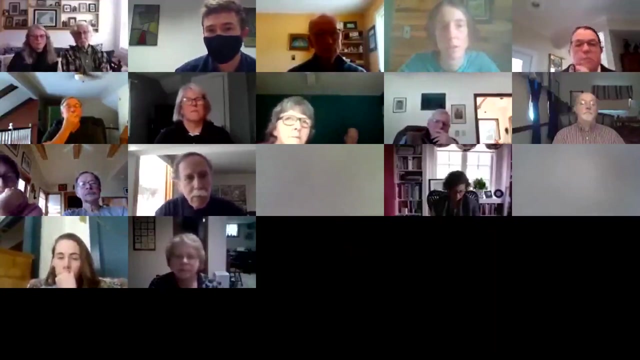 what was in there Because it is in kind of a public area, Public area- So it did have low levels of microcystin toxin, So below the 0.3 microgram per liter, that lower limit there. So low microcystin. 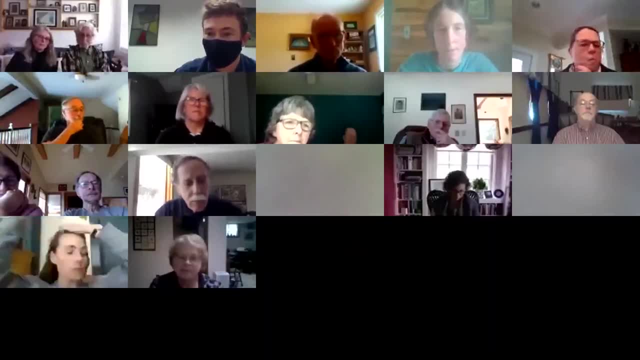 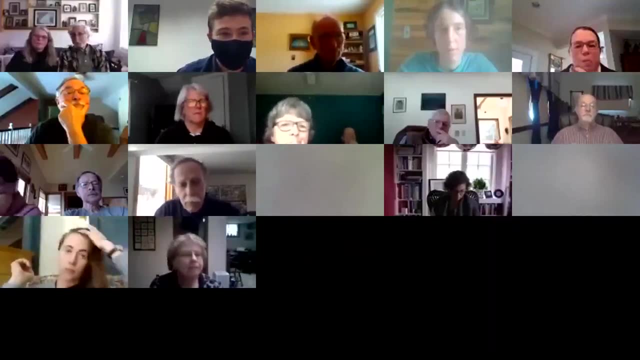 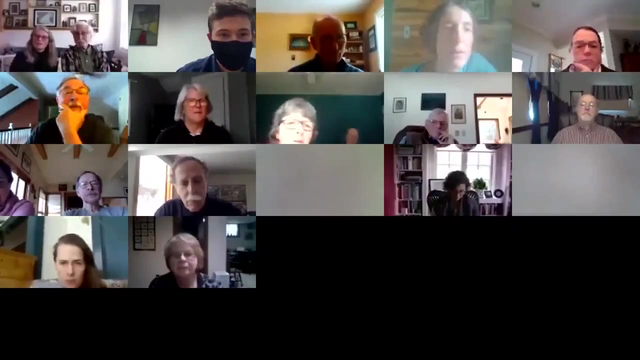 Great Douglas. Merrill had a great question. Douglas, if you'd like to unmute yourself and ask it, that would be great. Okay, Are people able to unmute themselves? Yeah, Yeah, He shook his head now, Oh, okay. 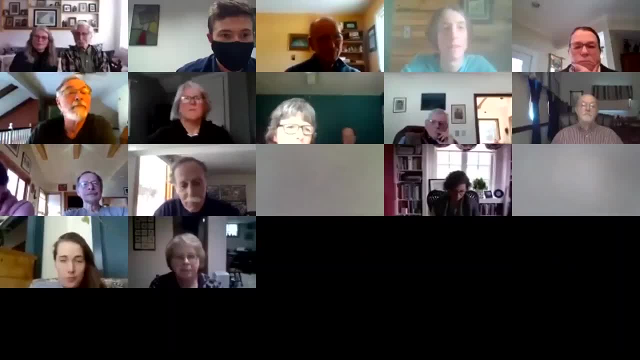 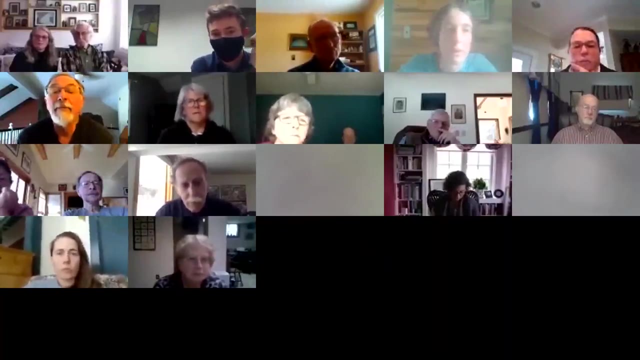 Here we go. Let me try this. There you go. Okay, Am I unmuted? You are? Yep, Yeah, I had a question for Adriana about how one differentiates the three levels of cyanobacteria. You had sparse, moderate and low. 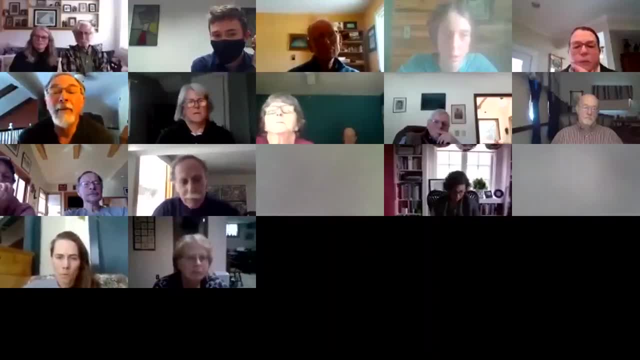 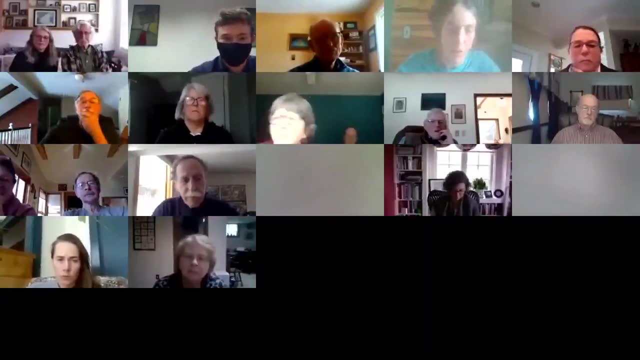 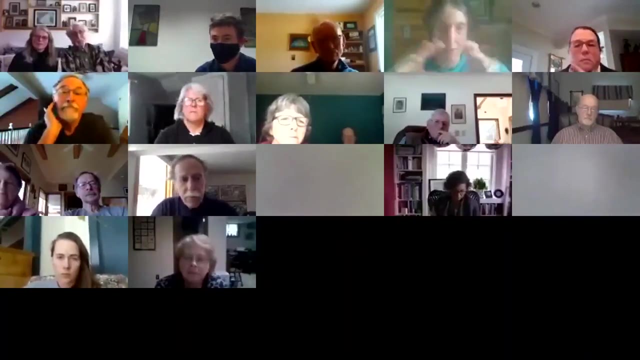 Yeah, And sparse, moderate and dense. Do you use a micrometer or how do you get to those differentiations? Yeah, So this is a little bit loose, Let me, but it's okay. So the sparse is when I'm looking in a field of view of, I think it's 0.1 milliliters for 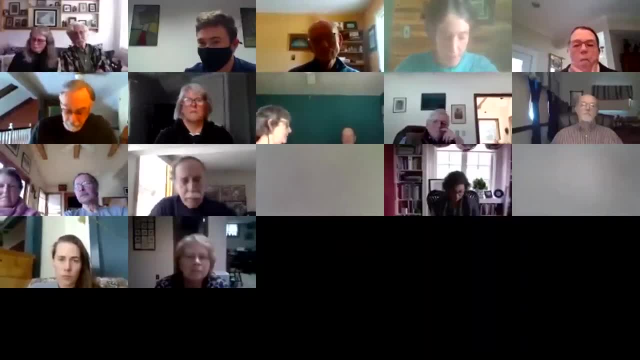 the average drop that I'm looking at Sparse is fewer than 10 individual colonies or clumps Or filaments are present. So this is more yeah, And then the sparse- let's see moderate- is more than 20 individuals. 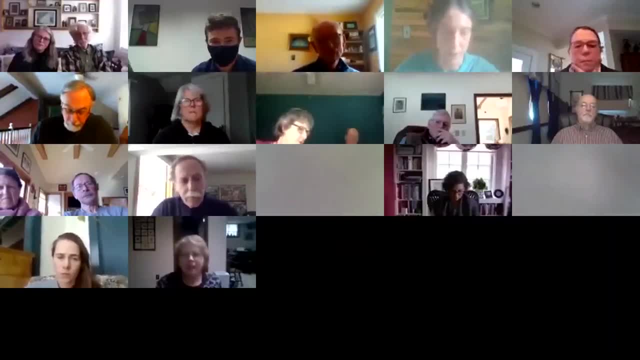 So sometimes we have this sparse, moderate, where it was kind of in between, like 10 to 20 colonies or clumps or filaments, And then dense is so more than so, moderate is more than 20, but it's under the field. 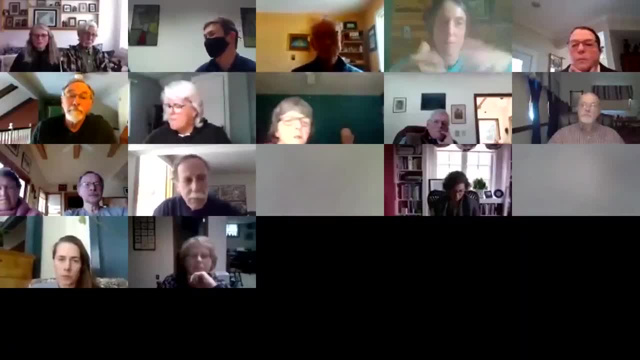 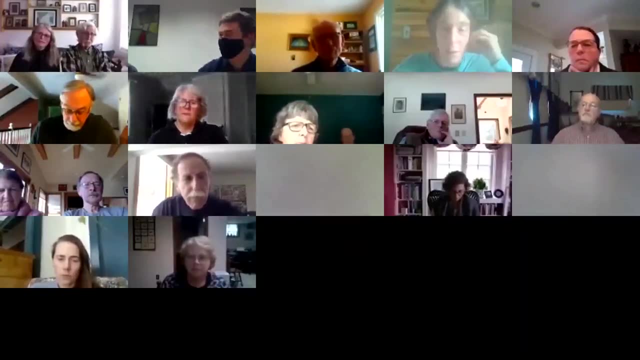 of view at any one point. So you're not seeing a whole lot right And you have to actually look a little bit. You're not seeing them in every field of view. Dense is like when it's really clearly in just about every field of view usually there's. 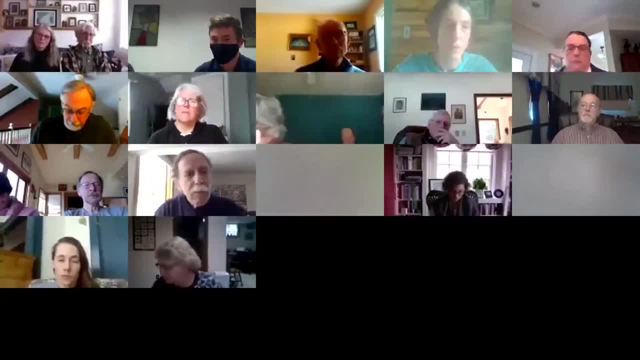 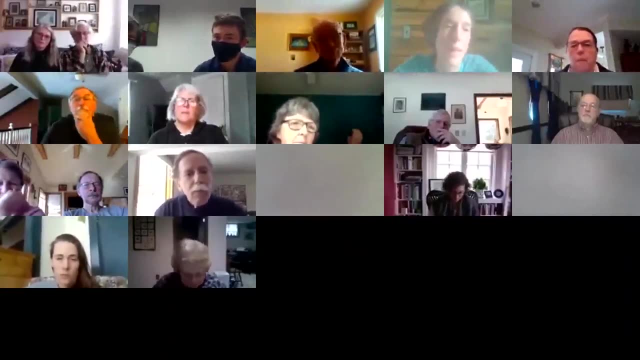 three or more colonies or clumps that are present. So yeah, we had to figure out a way without quantifying, because that's a little bit difficult and it might be a little bit misleading because it's not an exact science using the plankton net out there. 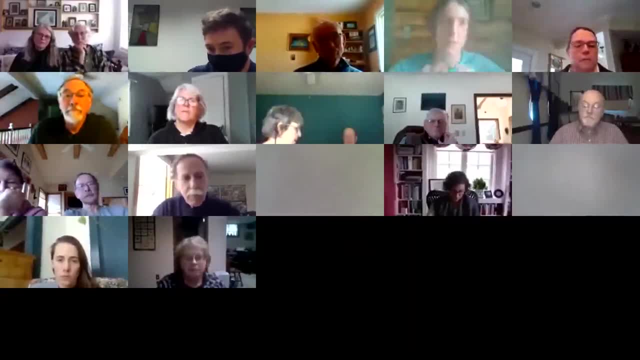 This is more of a sort of natural, Sort of naturalist view of just taking a look at what we see at different places at different times. There are ways you can quantitatively look at plankton, but it requires expensive equipment that we don't have at the lab right now. 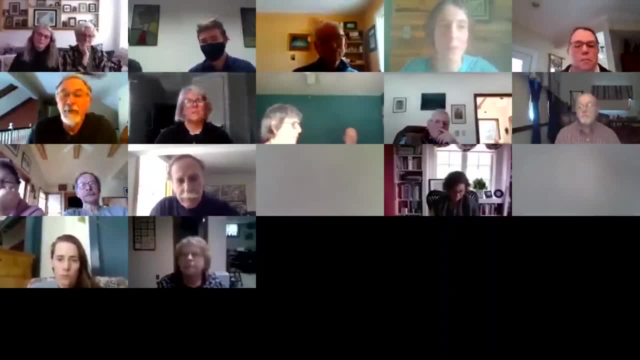 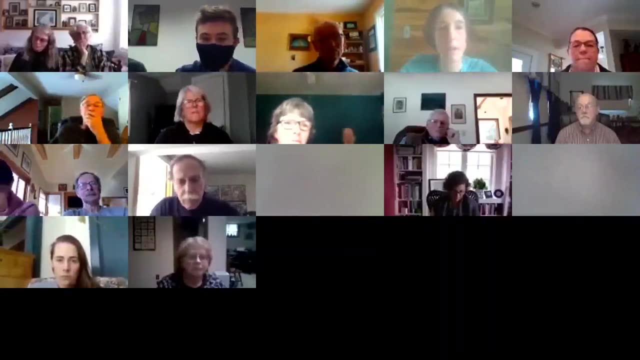 And a lot of time as well to do that. So, Okay, Thanks, All right, great. We had another question from Michelle Bamberger. Michelle, if you'd like to unmute your microphone, please, If you can unmute yourself and ask it, that would be great. 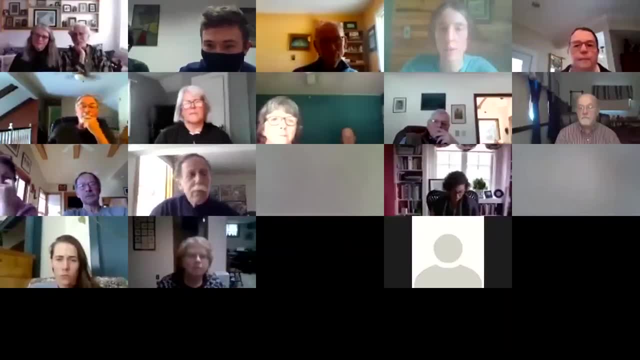 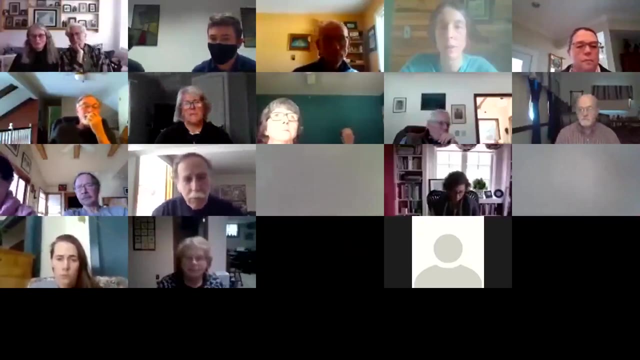 This is Robert Oswald. I'll answer. I'll ask the question. It's really for Steve. I was struck by the possibility that the microcystis blooms could have been correlated with the depth of the water, And the second part of the question is: is it? do you ever see any correlation between? 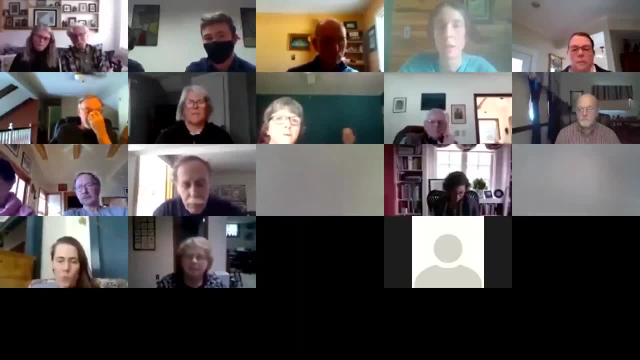 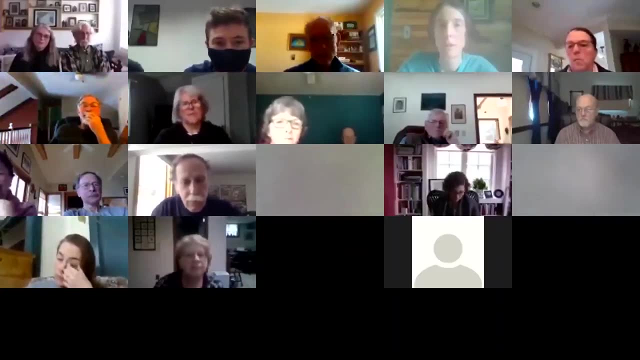 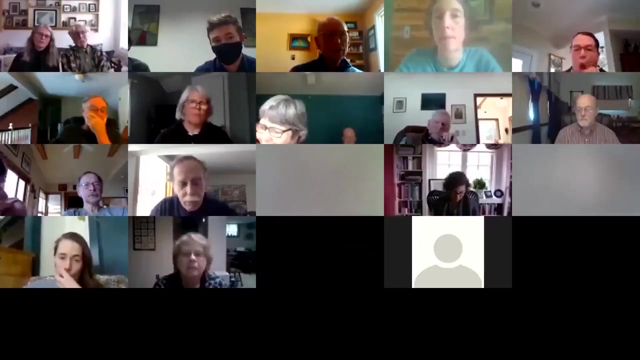 agricultural runoff and blooms. Was that for me? Yes, Okay, Okay. Correlation with agricultural runoff, I would say, well, first of all, we're not looking for it And second, I think it would be hard to determine. agricultural runoff goes into the streams. 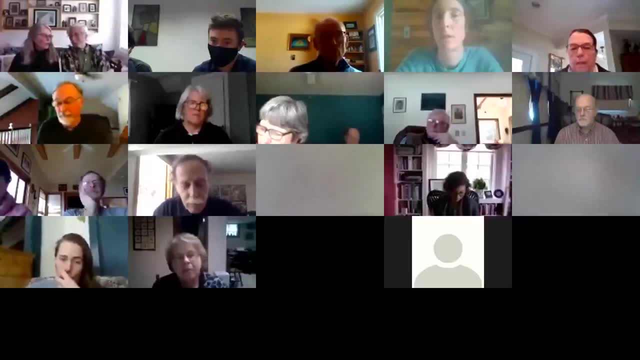 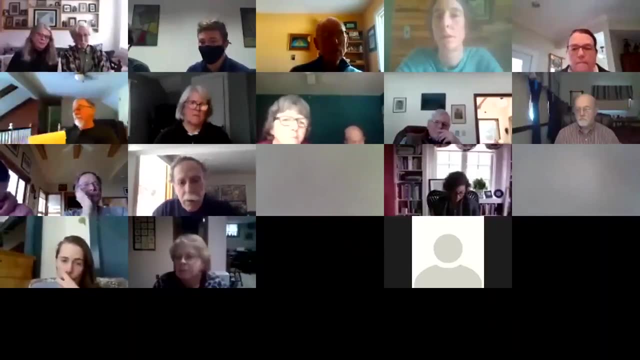 which goes, you know, which flow into Cayuga Lake. So One strategy would be to just look at the mouths of streams. We haven't done that, You know. specifically, I'm not convinced that it, that it would be worth the time, and 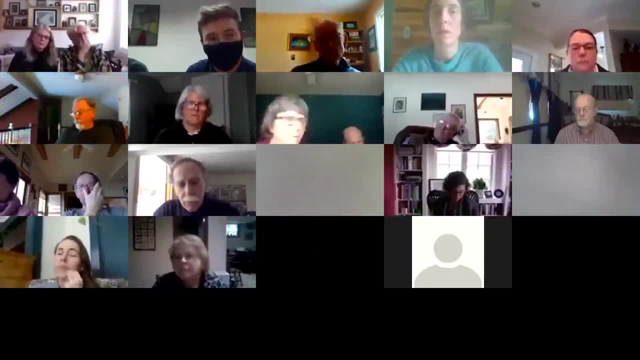 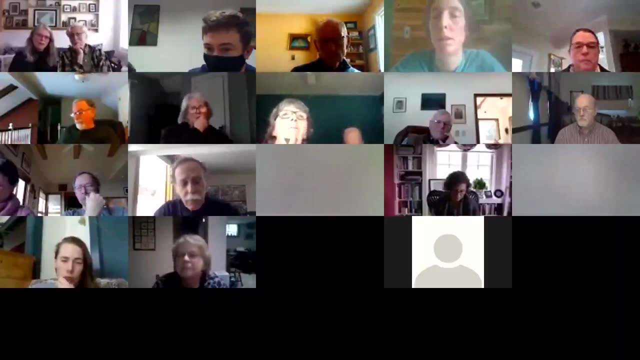 effort to do, but you know that's something that that that could be discussed and looked at. What was the other question, Robert? Is there a correlation between the blooms and the depth of the water? I think I'm going to look. 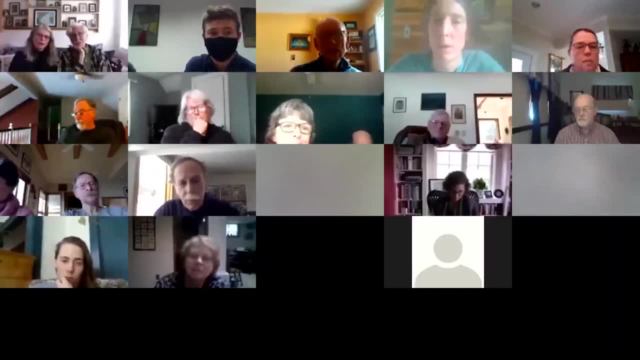 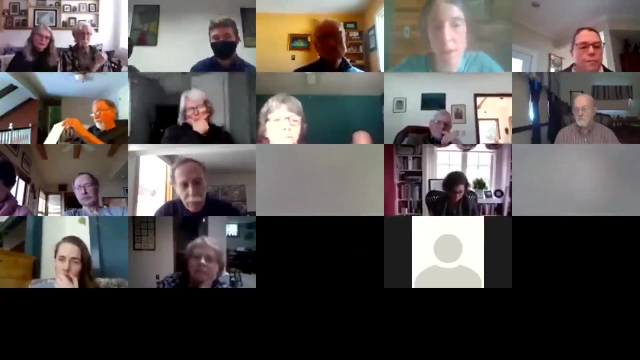 Okay, I'm going to leave that to somebody else. Who would that be? Maybe Adriana, would you be a good person to answer that question, or Nate? I mean, I think some people are looking at like. I mean, blooms tend to accumulate. 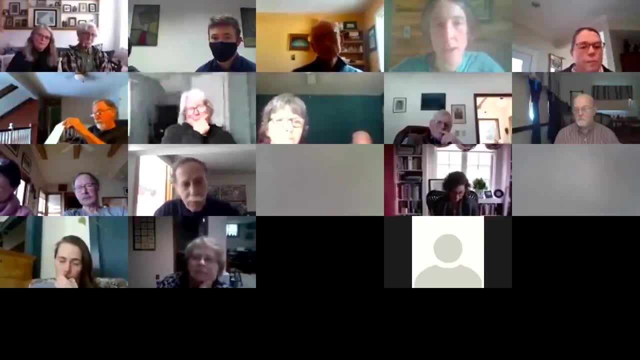 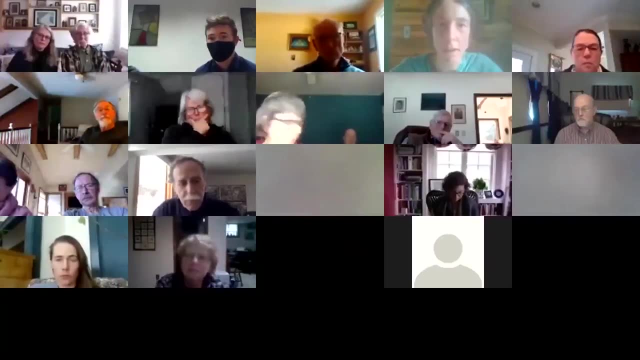 on the shoreline where it is shallower, But there are blooms that happen off of the Wells College dock, which is near the deepest part of the lake. There are blooms that happen in the shallower north end of the lake And things move around. 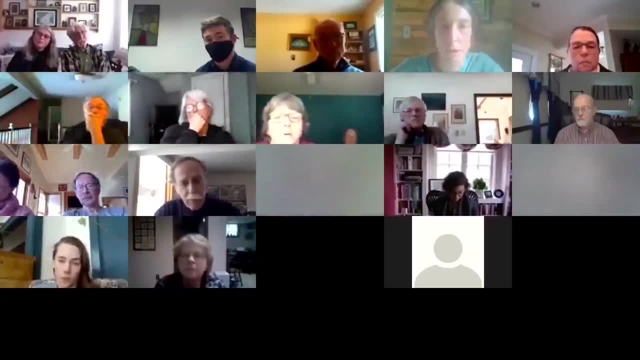 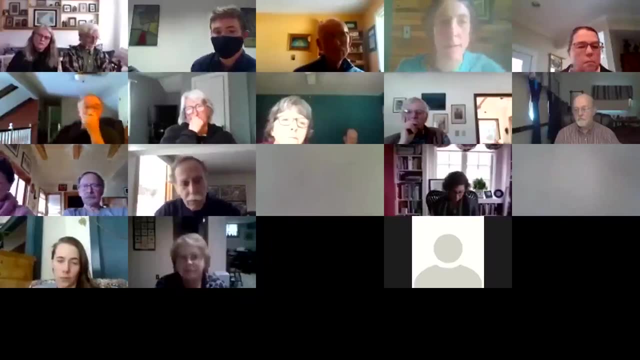 So you. certainly, when you have shallower water, it can be warmer temperatures which are conducive to cyanobacteria, but I don't know. That's about all I could add. I guess, And I think it's. I think it's also important to say that our volunteers are collecting. 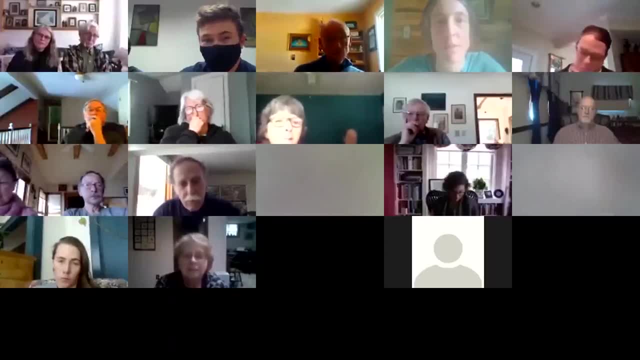 samples along the shoreline. So it is. so the water is not very deep. We do not try to sample for cyanobacteria out in Cayuga Lake. I mean, I guess it would be possible to do that, Excuse me, And we we asked Discover Cayuga Lake to you know if they see blooms, to you know. 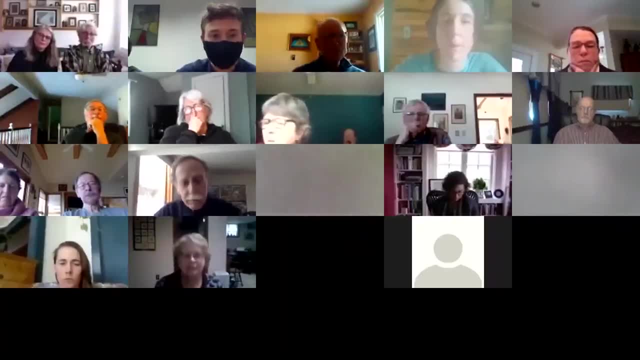 sample them right. Nate, they're kind of part of our network. if they're out in the lake and see a bloom and have the time, you know they can collect them. but by and large it's a shoreline bloom surveillance program. 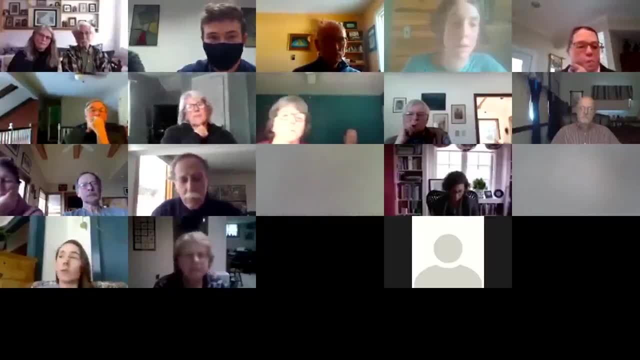 Okay, But they can't find them. So they they can't find them, but they can find them. They can find them by using the program. That's right, Yeah, Discover Cayuga Lake has been a great help with that. 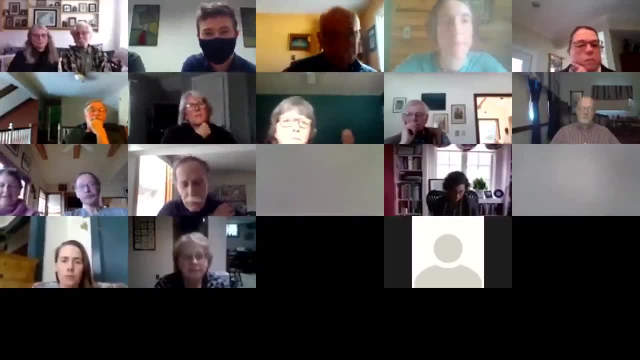 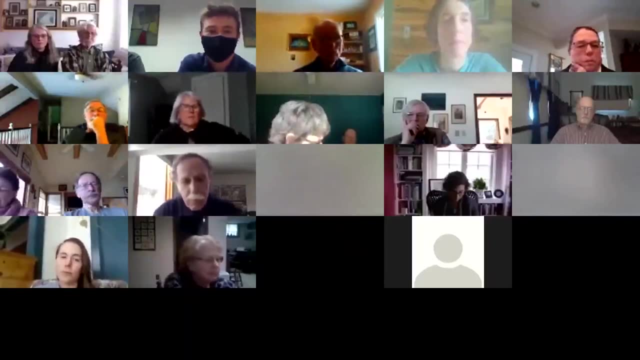 If there's any open water blooms and while they're out on the lake, we welcome them to collect a sample of that and to report it. Cayuga Lake Environmental Action Now has also been very helpful with that effort. You know, while they're out on the lake doing research, helping to collect those open water. 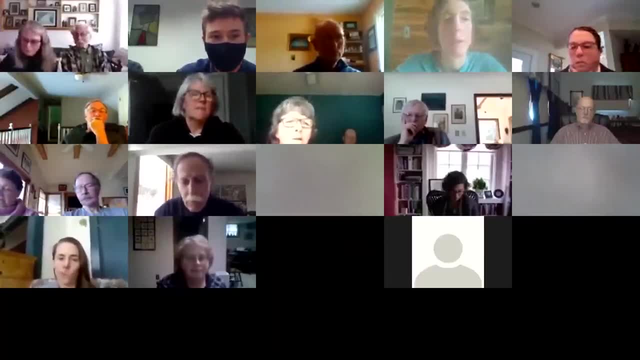 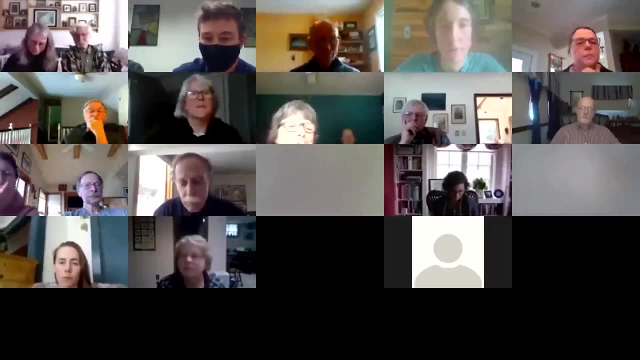 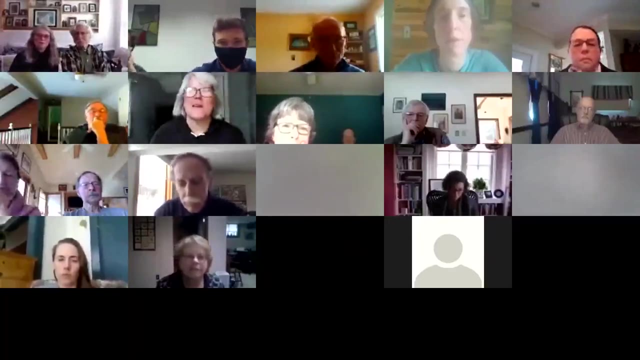 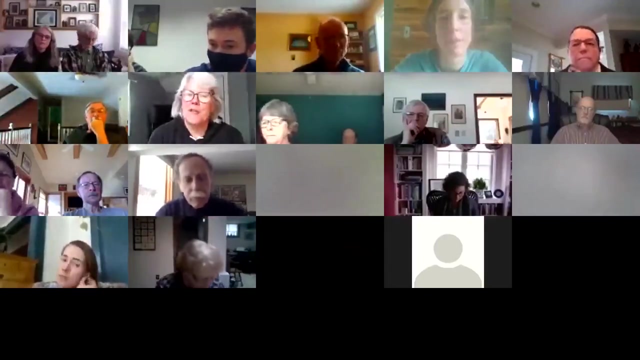 blooms if they occur. All right, Thank you. Thanks, Mike. So we had a question from Jody Price. Jody, if you'd like to unmute yourself and ask it, that would be great. My question, I think, was maybe more like a wow, I didn't know this when, Shelly and Sy, you were reporting that you had blooms that lasted 24 hours. 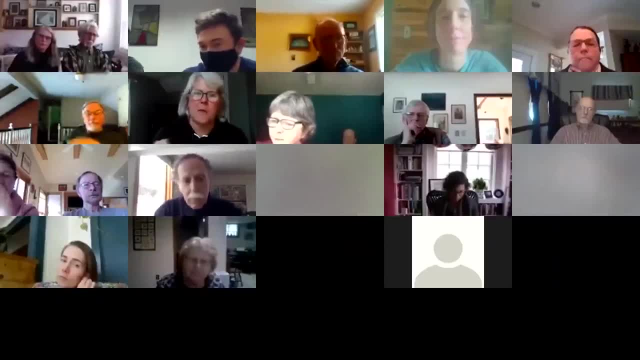 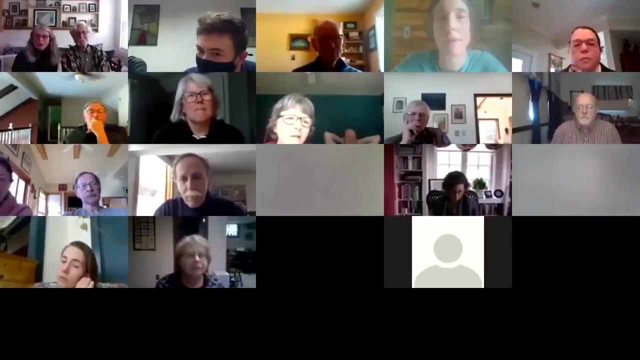 And I didn't realize that they would do that. I thought they dissipated, excuse me, after you know, the sun started to go down. Well, it does. it does get harder to detect any blooms as the sun goes down. 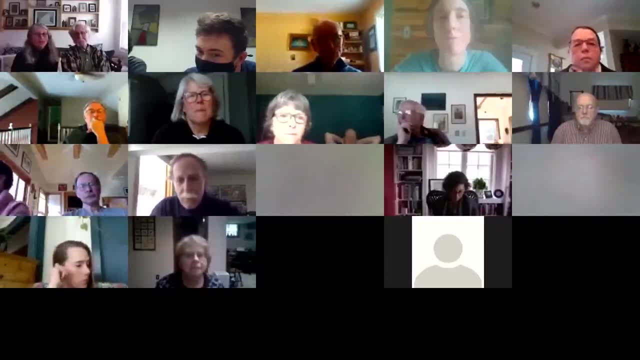 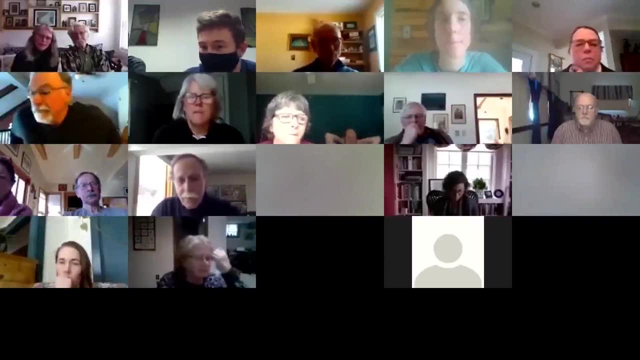 I'm not sure what they're doing at that point, But when it occurs early the next day and, can't you know, come back with a vengeance the way that it did in that one instance, I did have to, we did have to consult with Nate to determine: okay, is this a new bloom or the same thing? 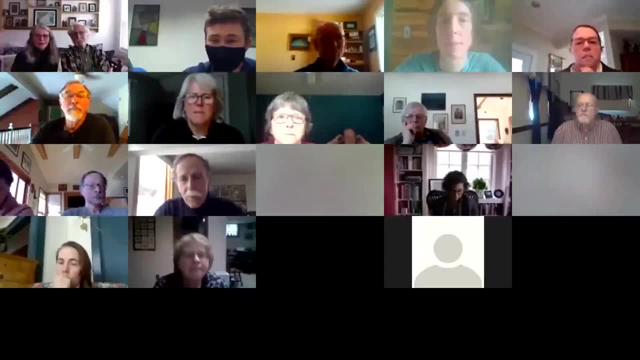 And I think with some consultation, we decided that we'd wait 24 hours in between without a bloom before we would consider it a separate bloom. But it was definitely the conditions were persisting. The wind was not, you know, usually when the 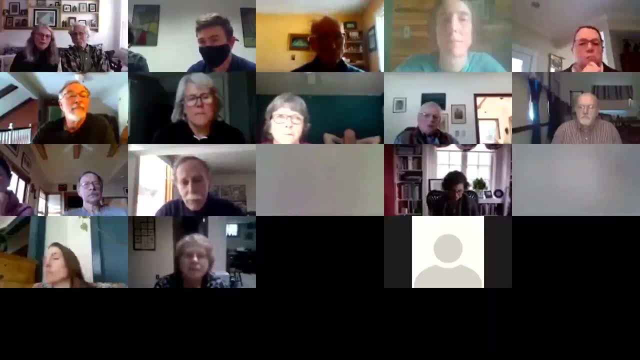 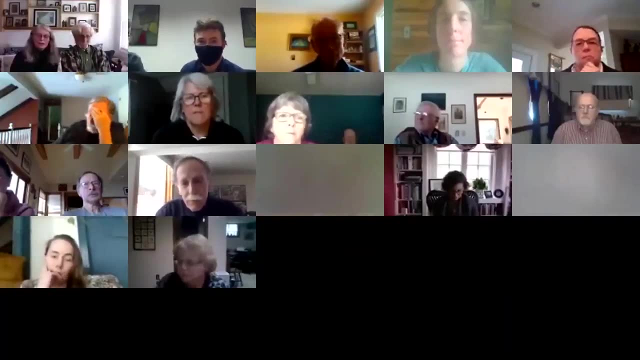 when the wind kicks up it does dissipate, but in these conditions it was just very still and very hot and sunny during the day, So the conditions were right for it to persist, it seemed. That's good to know as I look for them in our area. 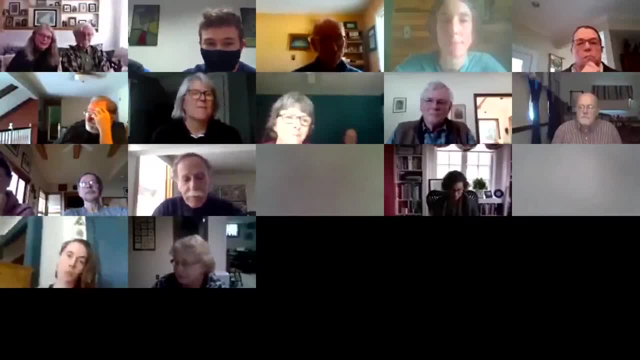 Thank you. Yeah, sure, Great. thank you, Tom St Clair had a great question, Tom. if you'd like to unmute yourself, Yeah, sure, Great. thank you, Tom St Clair had a great question, Tom. if you'd like to unmute yourself. 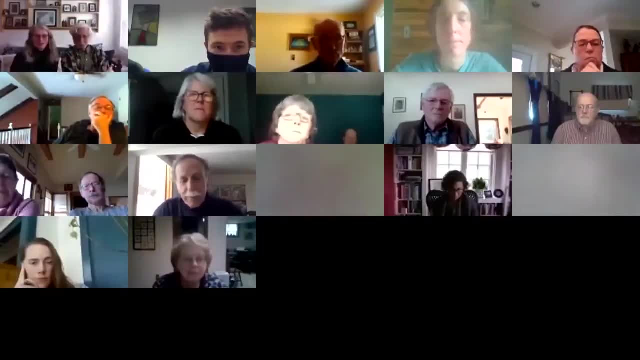 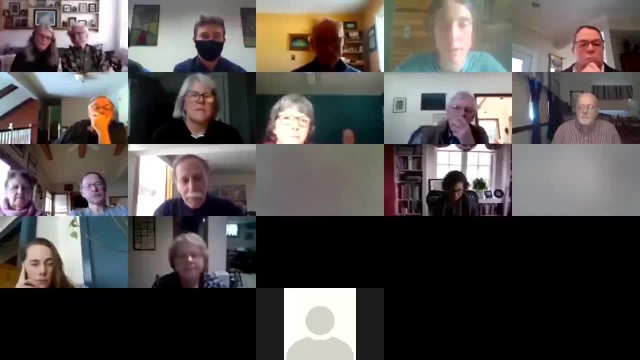 Tom St Clair had a great question. Tom, if you'd like to unmute yourself, If you'd like to unmute yourself and ask it, that'd be great Sure. Do we know if these types of blooms have been occurring for many years? 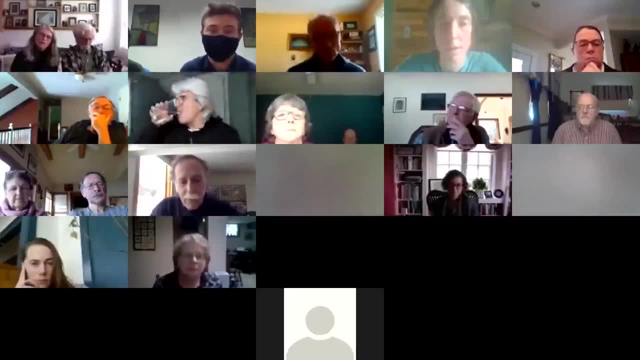 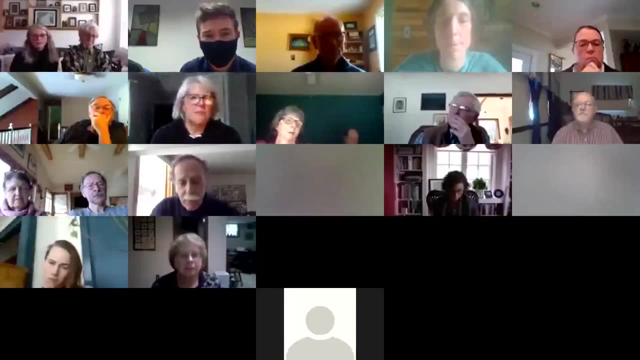 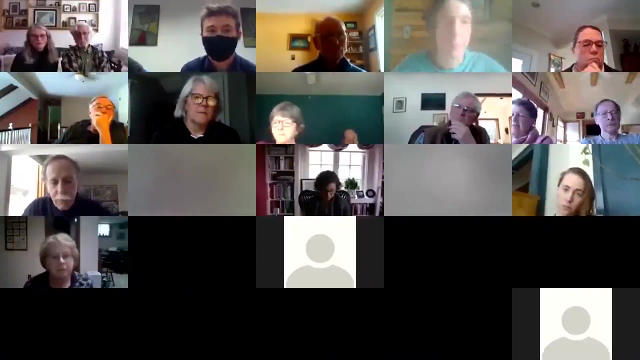 Or are they something relatively new, like in the recent past? I just I'm kind of wondering if they were going on for a couple hundred years, 500 years, two years. I don't really have a sense for that. Yeah, that's a great question. 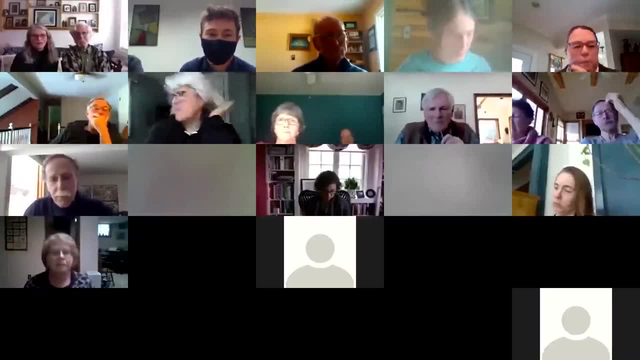 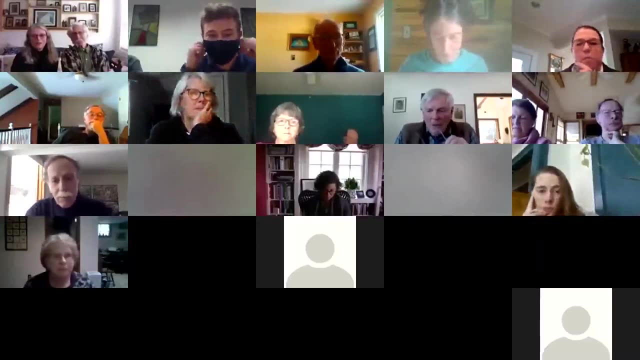 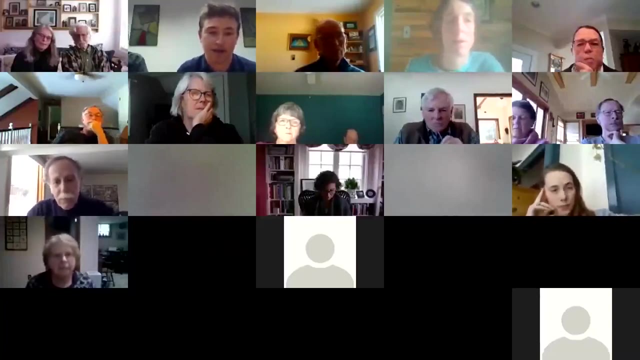 And it's a hard one to answer, certainly because many of these kind of comprehensive harmful algal bloom monitoring programs really began in the last kind of decade or so And that's when we started to get this really good record of harmful algal bloom occurrence. 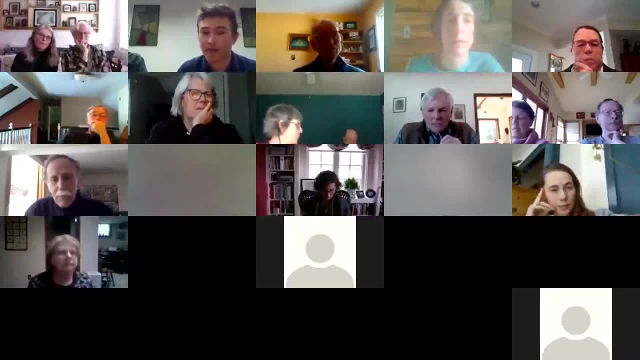 You know, I think, that harmful algal blooms have occurred for a long time. Although there we don't have very many historical records, There are, you know, comprehensive records of them. I might also open this up to any HABS, Harriers or Lakeshore homeowners who are out there. 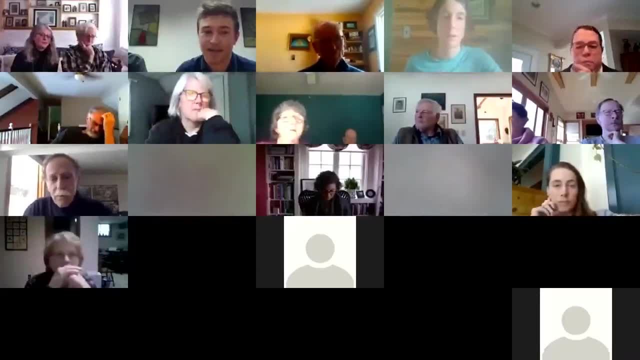 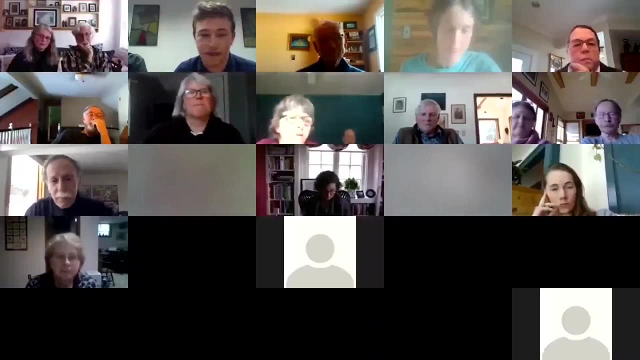 You know. if you remember these blooms happening in the past or not, or have any stories about that, you could unmute yourself and comment. I spent a lot of time in the lake when I was young and into my teenage years, And that would be the 60s and the 70s. 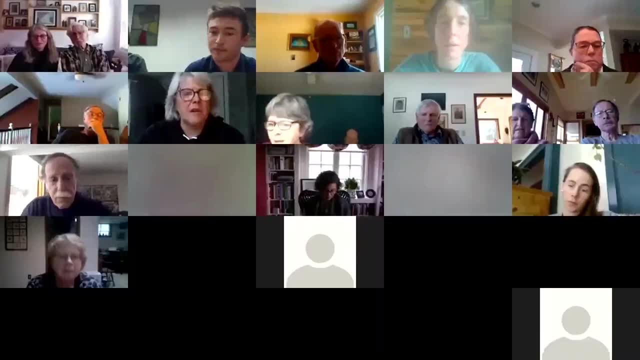 My grandparents had a farm and we had a cottage on the lake below the farm And I don't ever remember seeing anything like that, like what we're seeing now at that point, And that was across from what we call the power plant in those days. 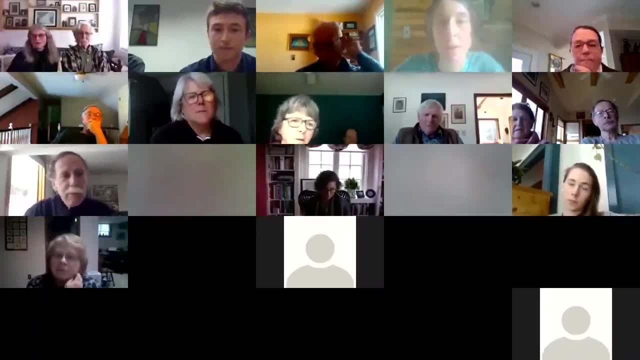 Just from a plankton survey perspective. there are a few years in the past, in the early 1900s, and then some other years, And most recently I found a report for 2013 when some plankton surveys were done in the lake. 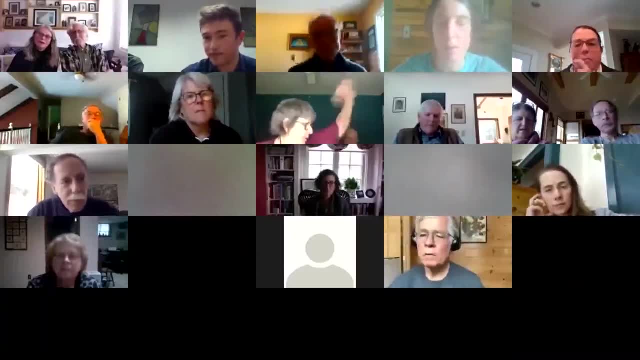 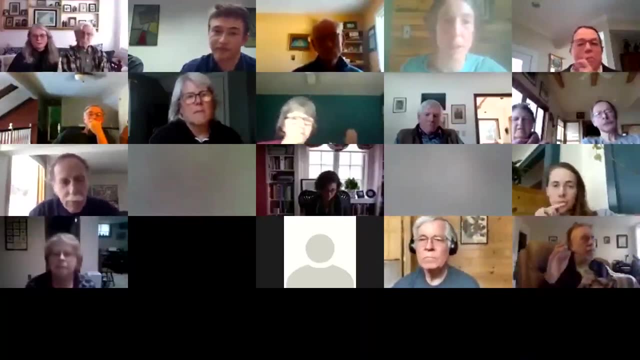 And these were done every few weeks And it just really looked very different than what we see now. when I look with the plankton surveys that we're doing And it seems to be a phenomenon all over the world that's happening. These harmful algal blooms are increasing. 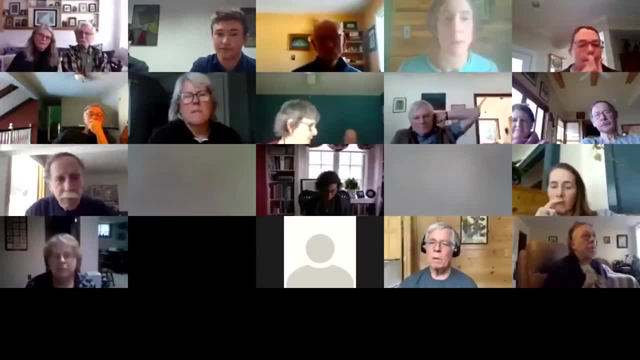 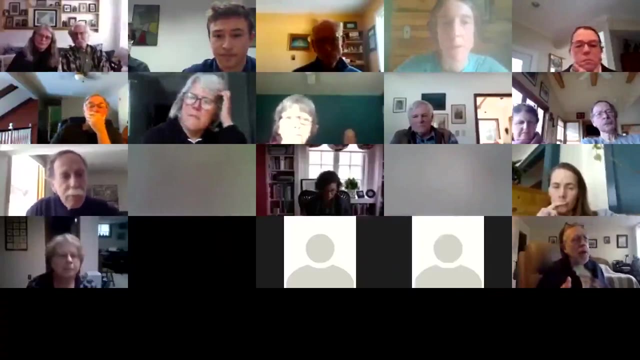 And it's not always cyanobacteria, like the ones you hear about in Florida- are dinoflagellates And sometimes Cyanobacteria are involved as well. But yeah, And this is Ed Swayze- My grandparents owned land in Lansing. A little piece of lakefront that they bought from relatives we had there in the 50s And I started going there in the 50s with them And eventually my father- My father- took that over and then I took that over and I just sold it a couple of years ago to another family member. 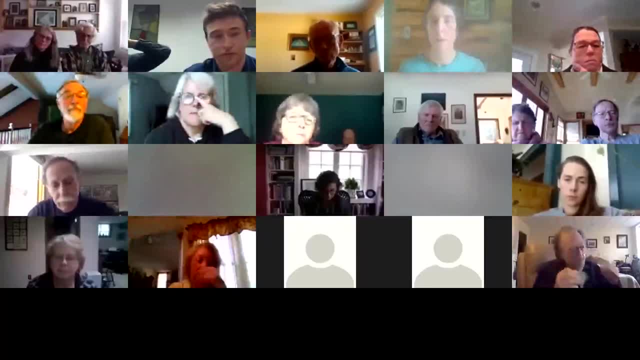 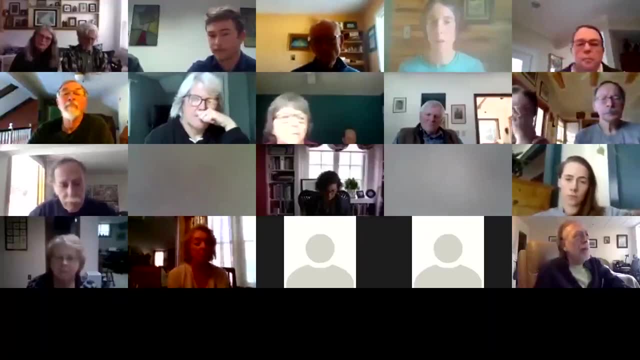 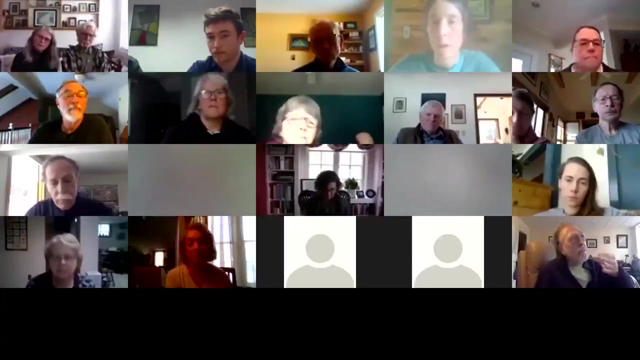 But my sense is that in those early years this wasn't obvious. You didn't see much And of course we were ignorant to even be looking for it, of course. But I do remember, As I lived there for 15, 20 years, that we started to see it toward the end of that period. 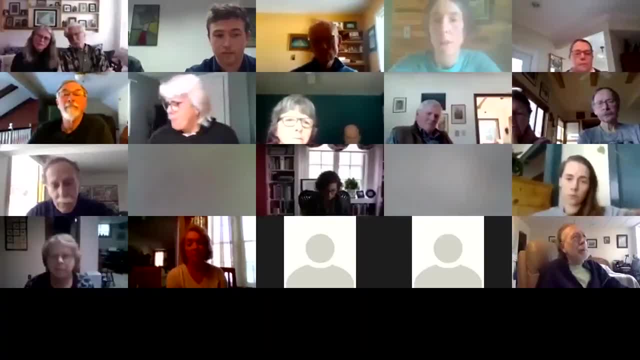 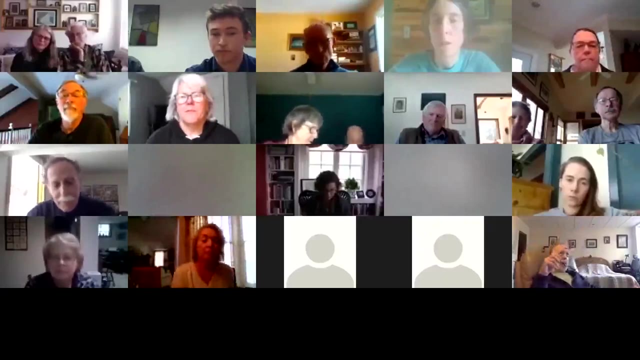 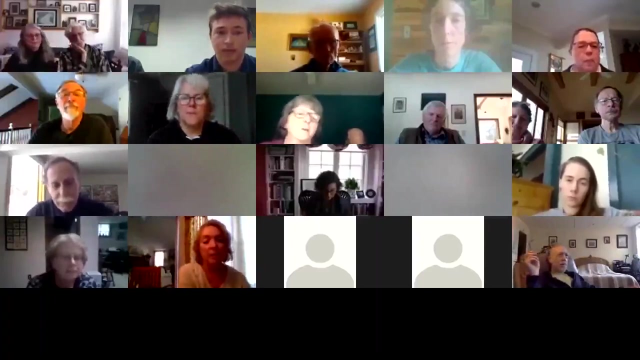 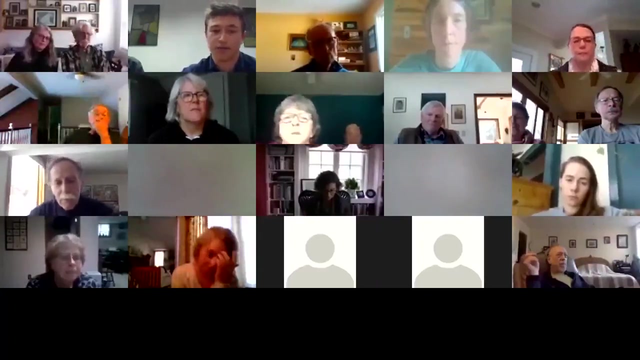 So we sold it in well anyway in the aughties, early and mid-aughties. So I have a sense that it's just been a gradual increase. Yes, Thanks, Yeah, Based on kind of what we're starting to see through our Blue Monitoring Program, I think we get a similar impression. 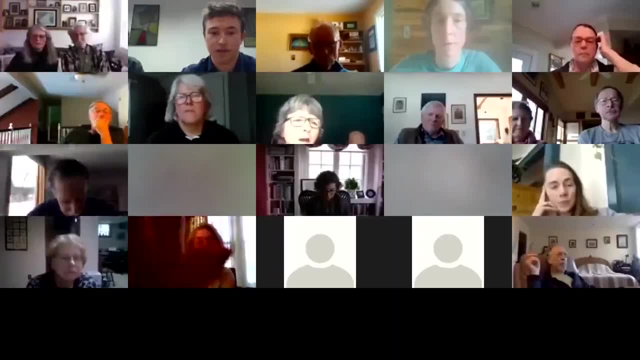 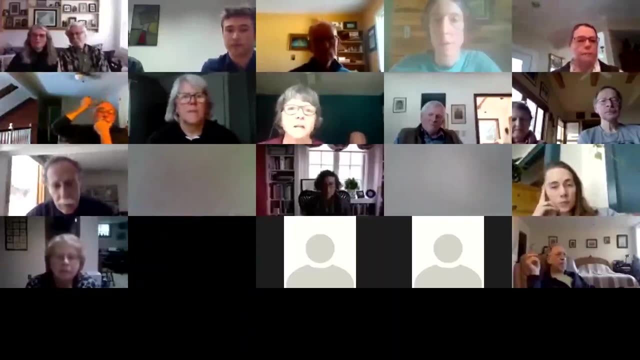 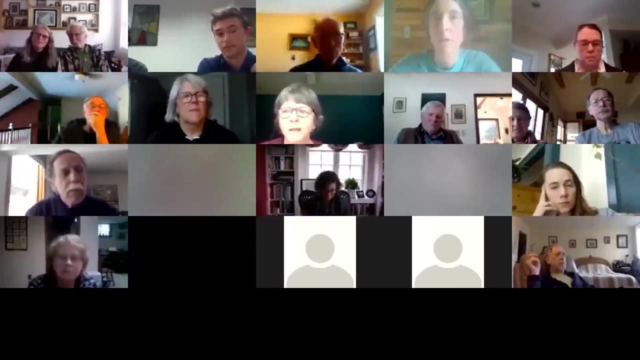 Joyce. Leslie, you had some good questions. Joyce, would you like to unmute yourself and ask them? Yes, My name is Leslie Webster and we have a cottage just south of Teganik. My question is why, in the fall, like September and October, when the water's cooler and it's 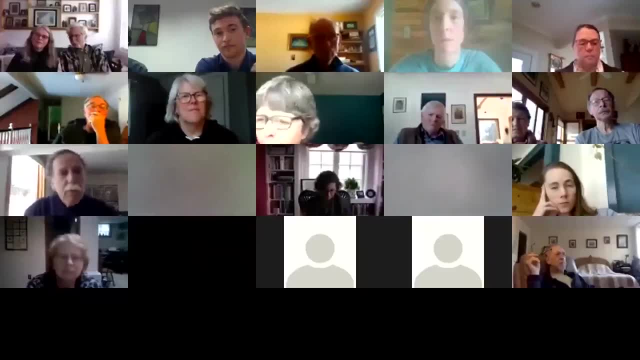 windier. why are there more microcystis then than in the middle of July or August, when it is hot and still? We've seen blooms, and it's usually been a hot still day. Once the wind comes up, we're good. 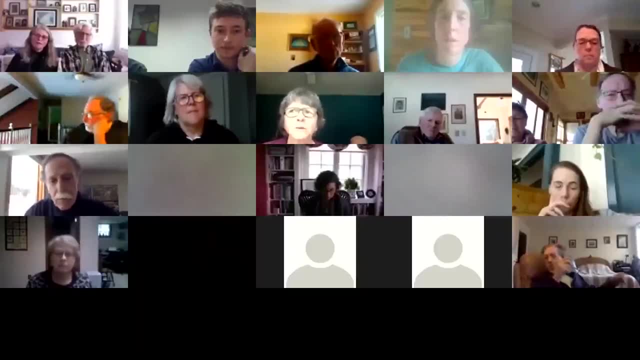 So why has the level been so high the last two years in September and October? Could it be? Could it be the From Adriana? Could it be? Could it be nutrients coming down the creeks because there's more rain and there's more? 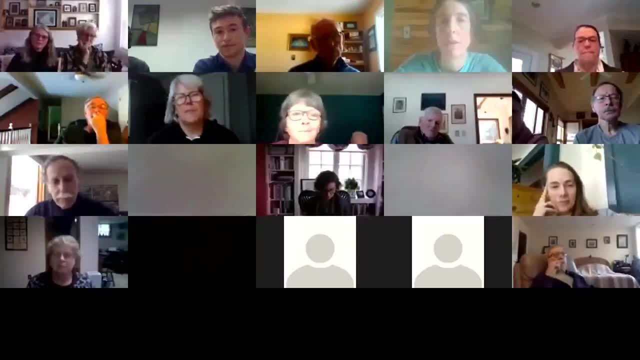 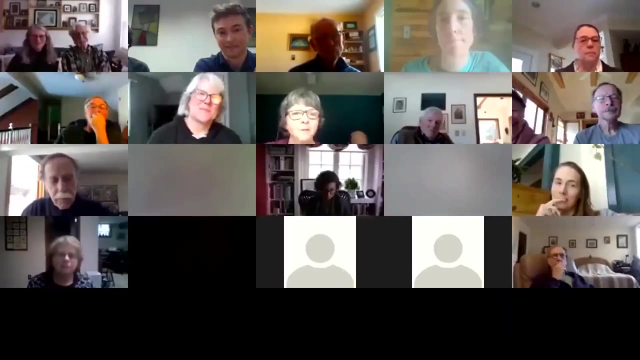 nutrients out there at those times. I was just going to mention that water temperatures are still pretty warm at that time of year, Not if you go in the lake. it's freezing. in September It's a lot cooler than August, Maybe not near the surface, but there's a definite cooling off. and after Labor Day 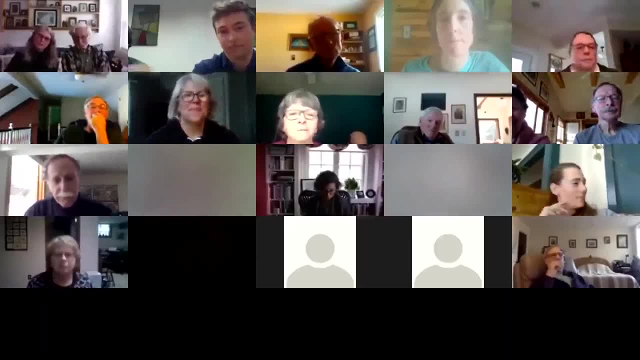 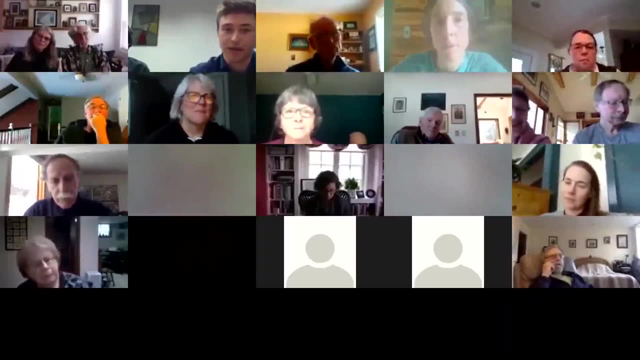 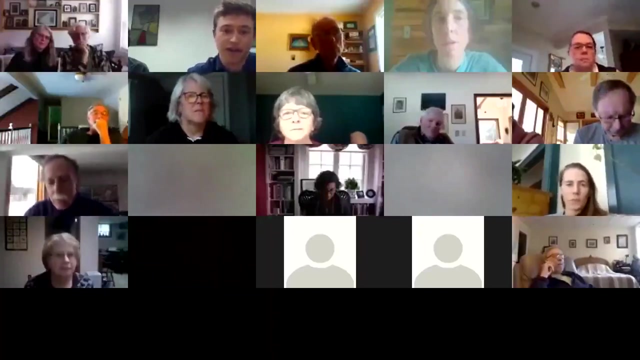 there's a definite cooling off. Yeah, one of the things that we've seen in our bloom record from the past three years is that the types of cyanobacteria that we see in these blooms. it seems somewhat seasonal in a sense, and maybe others can comment on this, whereby in 2018 and 2019, we saw blooms. 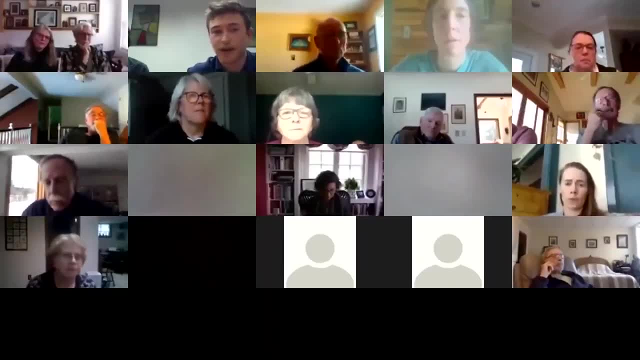 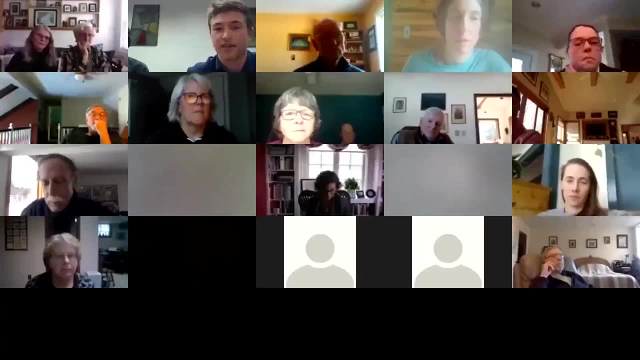 that were dominated by Dahlkos spermum primarily in the early summer months, And then the The, The microcystis blooms would follow in like late August and September. So there could be kind of a seasonal succession factor even within the cyanobacteria community. 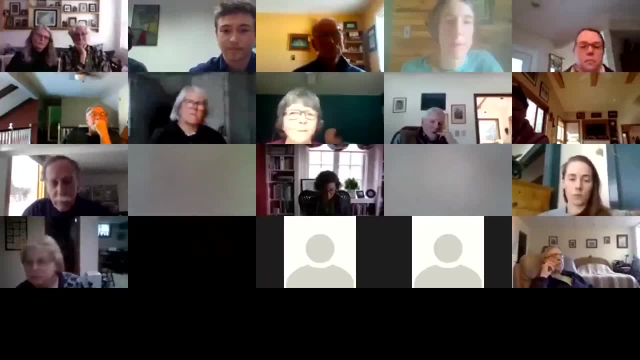 Okay, Yeah, and I want to add, I'm a fifth generation living on the lake and it's definitely a lot different than it used to be. I don't know when people started noticing these, but I had never seen them growing up. 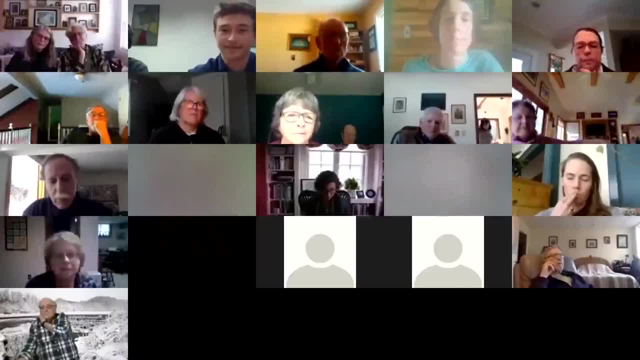 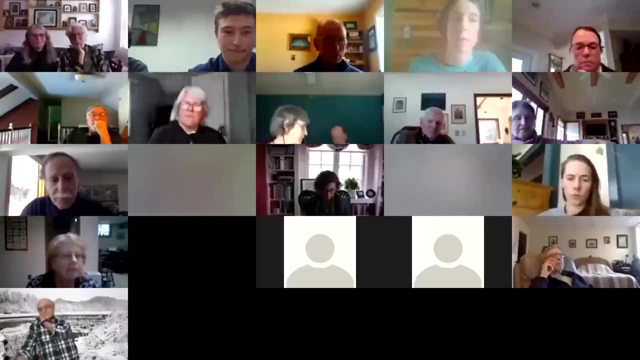 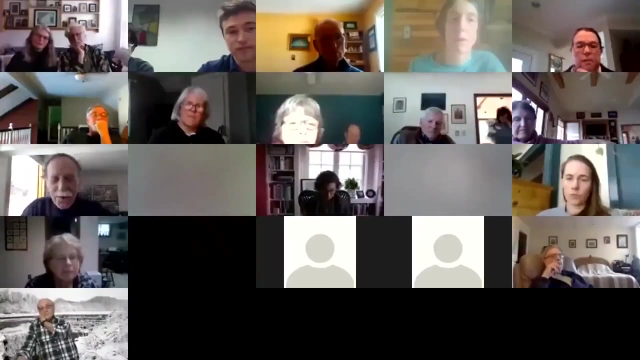 Yeah, And I think it's concerning John Dennis. you had a great question, John. would you like to unmute yourself and ask it? Sure, Thank you, Nate. I thought of a second question, So the first question was just: do the folks at CSI think that water temperature warmer? 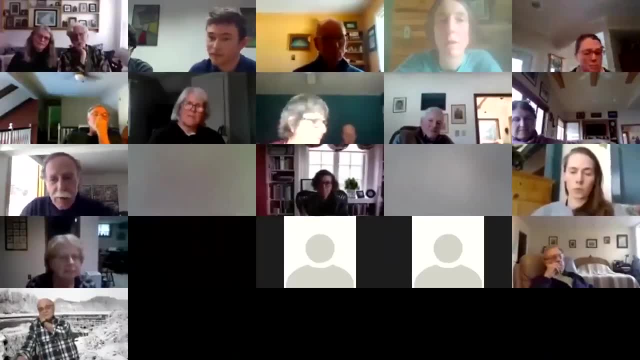 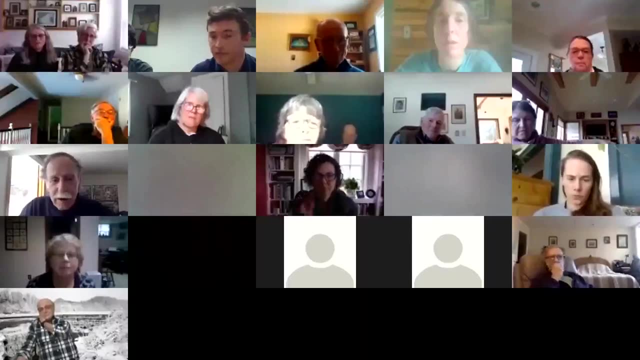 water temperatures and phosphorus are the key drivers of blooms on the lake, And my second thought was If we could invite Tom Vorder to comment why Onondaga Lake hasn't had any serious blooms, whereas Cuyahoga Lake has. I don't know if you'd be willing to comment on that. 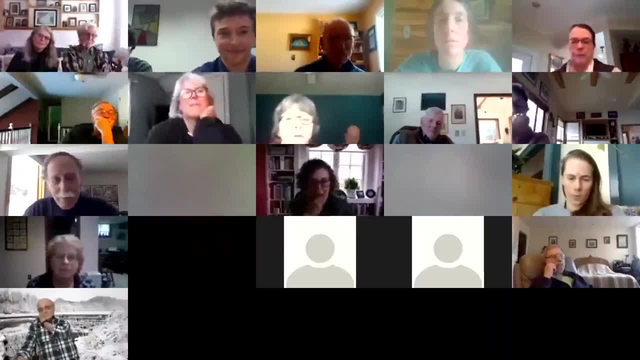 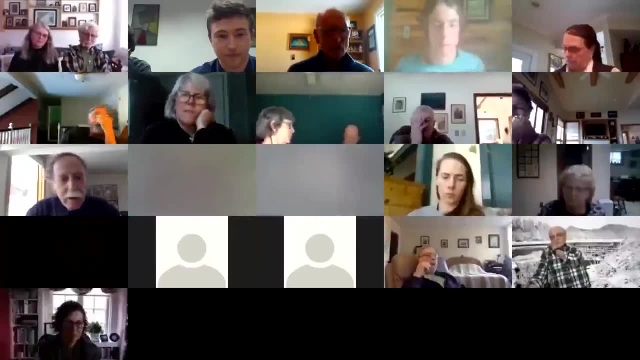 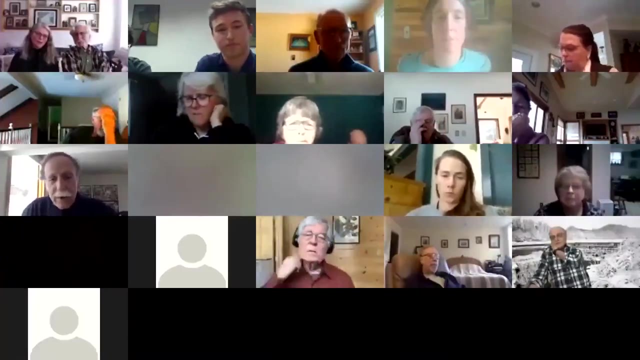 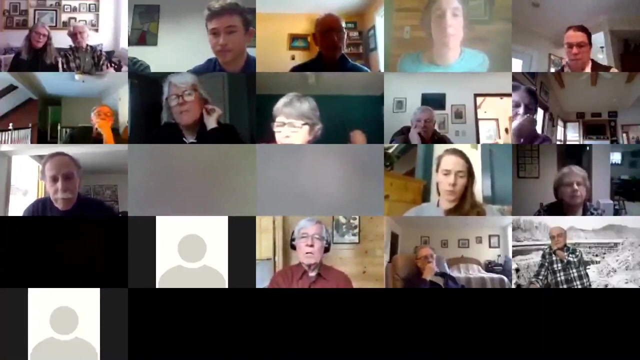 So the first question, John, could you repeat it please? Sure, just do you consider that warmer water temperatures and phosphorus- you know, higher levels of phosphorus- are the key drivers of blooms on the lake? Well, I mean, I think it's generally accepted that both of those are drivers, you know. 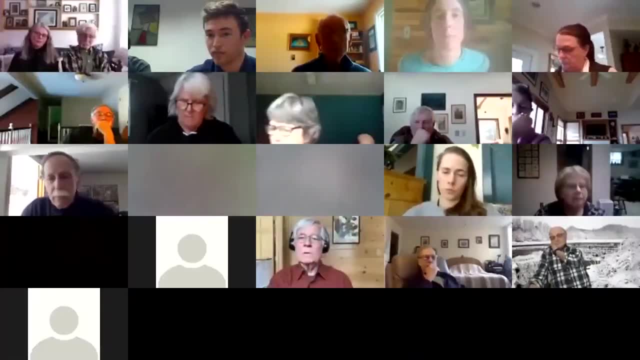 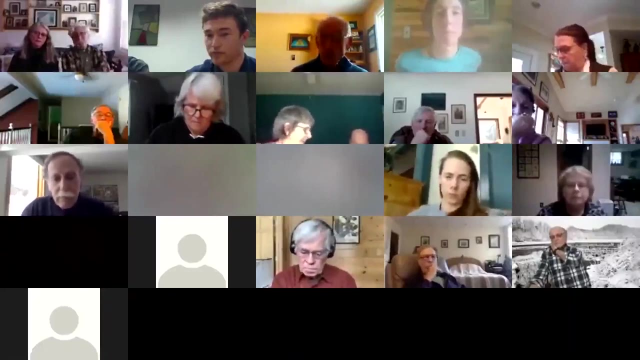 temperature and nutrients, particularly phosphorus, but whether they're key drivers on Cuyahoga Lake in particular. I mean, we can't say that we don't have any evidence to support a key role on Cuyahoga Lake, But in general, yes, absolutely. 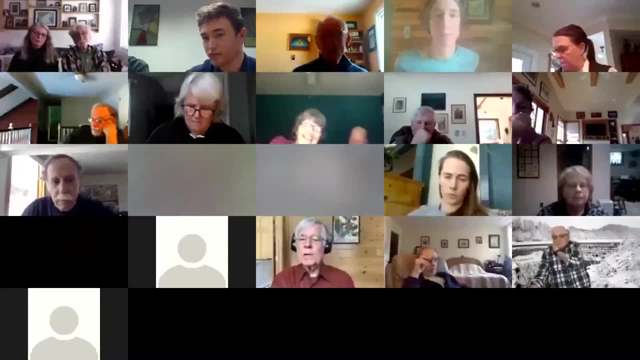 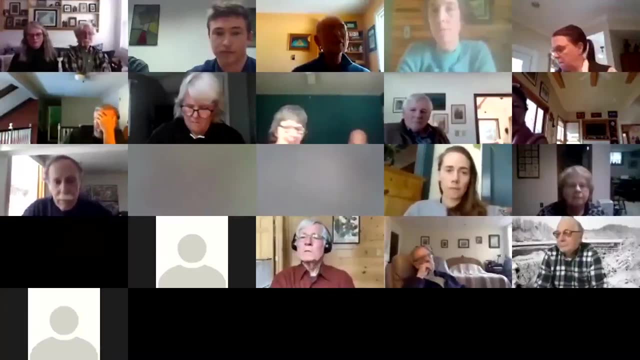 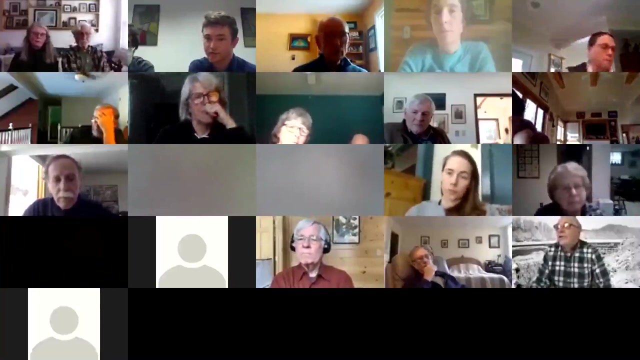 Temperature and phosphorus are very important, But having said that you know, it's important to realize that not phosphorus concentrations- elevated phosphorus concentrations do not necessarily result in harmful algal blooms, And low concentrations of phosphorus do not necessarily exclude harmful algal blooms. 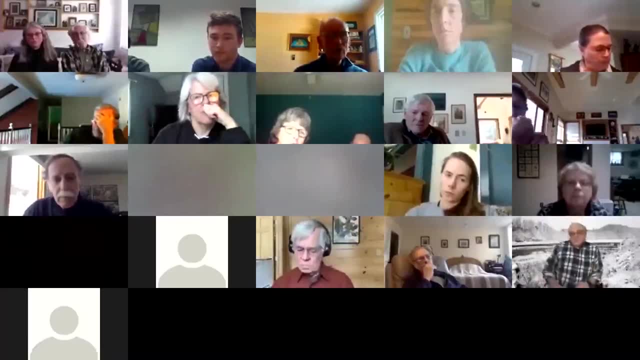 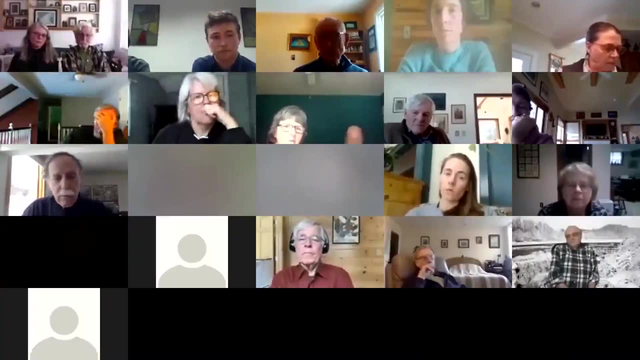 And I think the poster child for that second scenario Right was Skinny Atlas Lake right- Very low phosphorus concentrations and yet a few years ago at least they had a lot of blooms. So it's, it's, they are drivers, but it's not a one-to-one correlation. 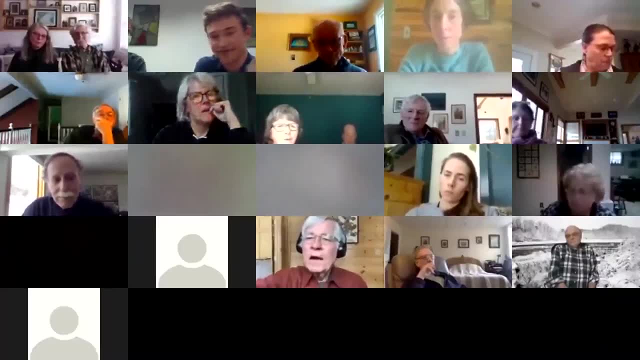 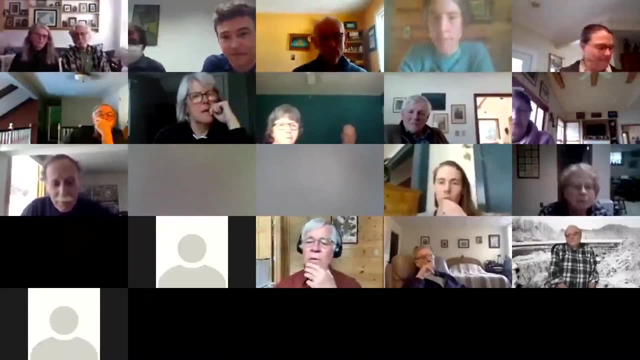 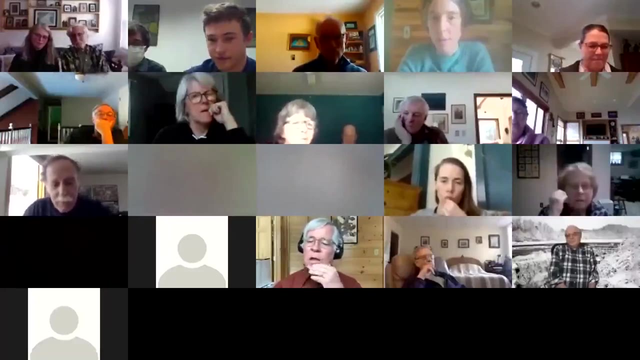 And now I'll turn it over to Tom. Hi, am I? am I unmuted? Yes, I should be. That's an interesting question about the relationship between nitrogen and phosphorus. Yeah, Yeah, Yeah. So the two kinds of nitrogen and phosphorus, in causing blooms. 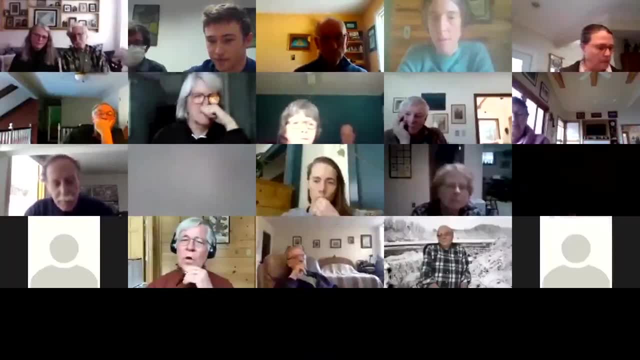 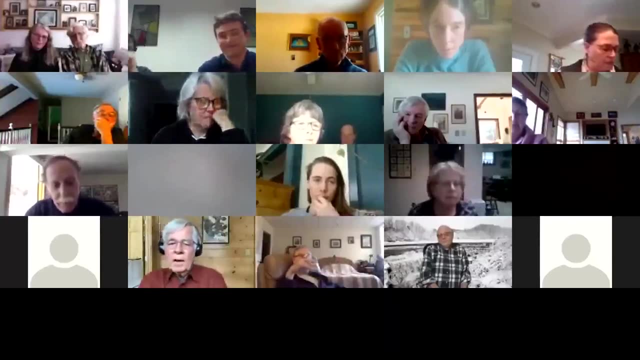 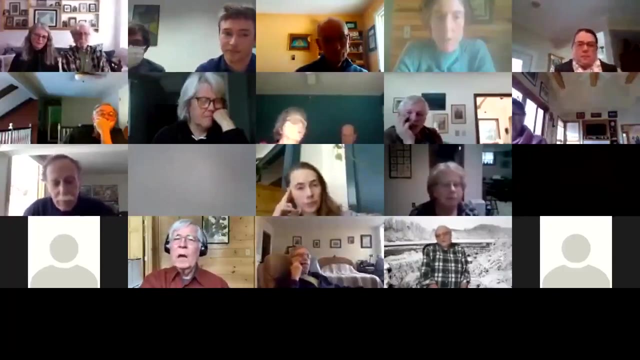 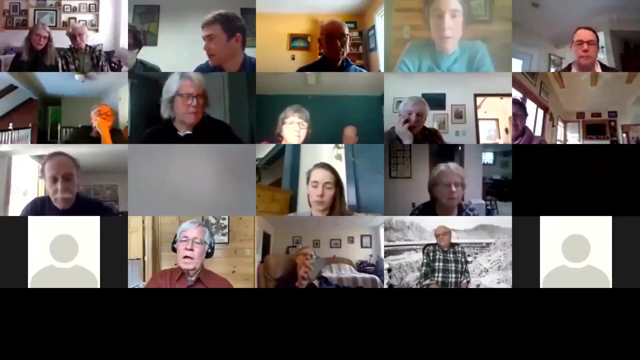 Onondaga Lake, historically, was notoriously prone to harmful algal blooms in the late summer and autumn, was at one point considered the most polluted lake in the country, I think. But in the process of solving those problems, The A metro wastewater treatment plant in Syracuse, which was the source of many of the nutrients entering the lake, introduced a process that got rid of the ammonia that was going into the lake, which is a toxin, of course, to most things, converting it into nitrogen, nitrate, nitrogen. 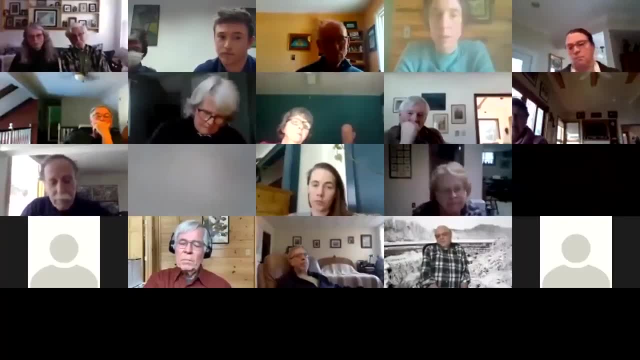 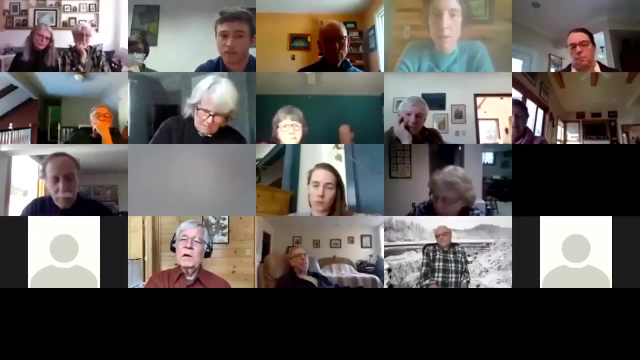 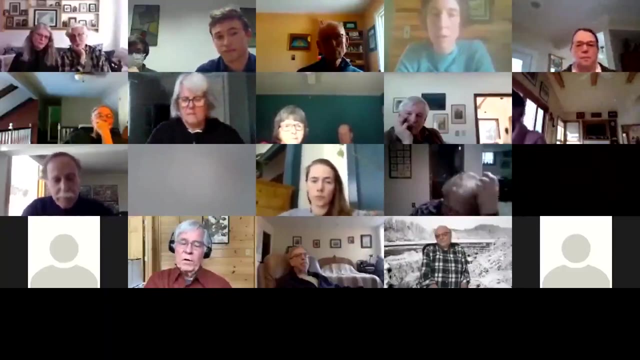 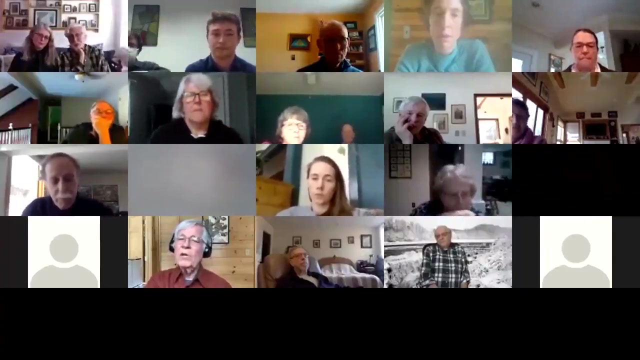 Now that cyanobacteria- some of them, as I think Adriana pointed out- have the ability to fix nitrogen from its rather unavailable state in the atmosphere and therefore dissolved in the water, And by that means they gain some advantage over the other kinds of algae, the competitive advantage over the other kind of algae in the lake. 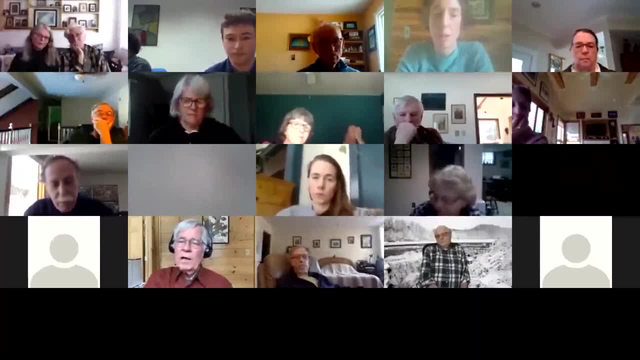 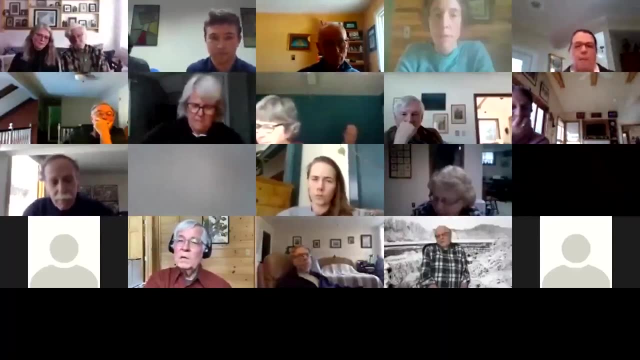 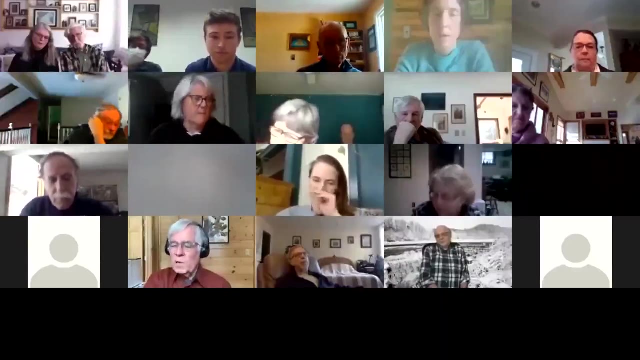 But there's been a sort of rule of thumb that as long as the nitrogen to phosphorus ratio was less than 29 to 1, I think that that advantage didn't excuse me, that that advantage to the cyanobacteria didn't occur. But once the nitrogen to phosphorus level got greater than that, in other words, as the relative amount of phosphorus increased- excuse me, relative amount of nitrogen increased- the cyanobacteria lose their competitive advantage and harmful algal blooms are less likely to appear. Kind of a complicated answer and I'm not sure it's held up, But the issue in Onondaga Lake right now is it has a very high nitrogen to phosphorus level because of this increase in nitrogen from the sewage treatment plant. It's well over 100.. 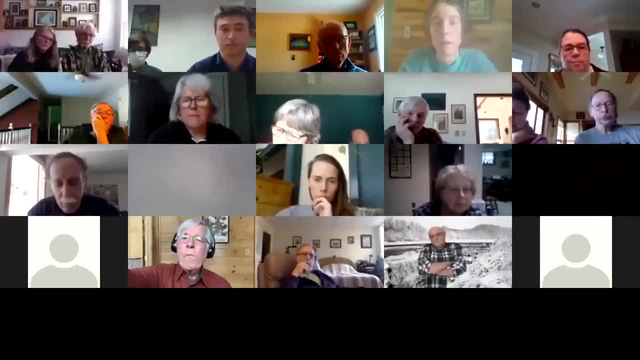 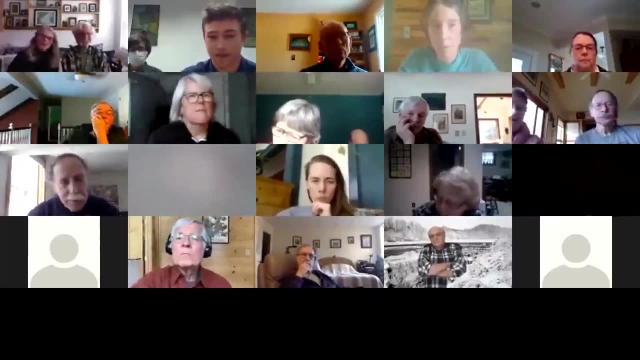 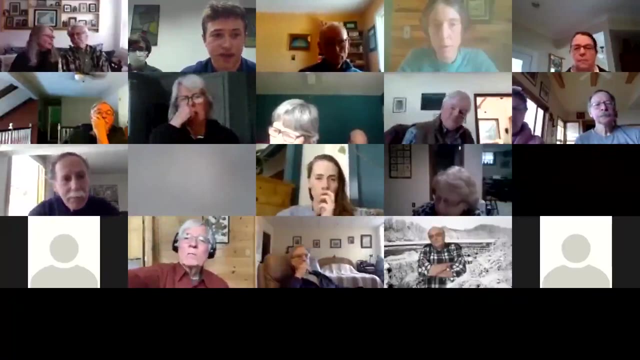 It's over 100 to 1 at this point. Thank you, Yeah, those are great answers to that question. Kathy Quitt has a question. Kathy, if you'd like to unmute yourself and ask it, that would be great. 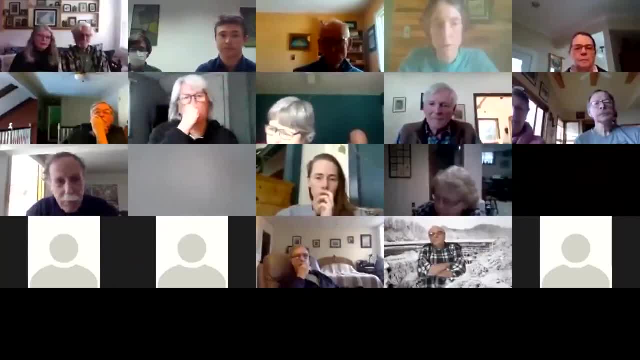 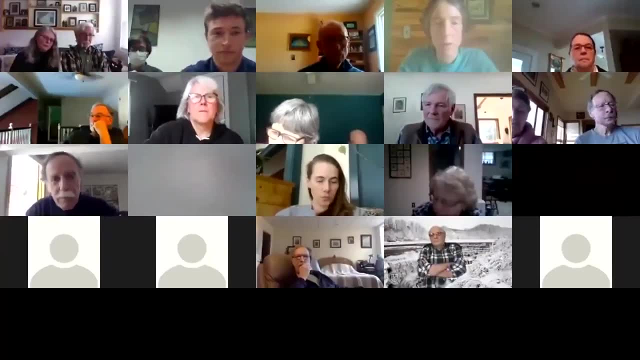 Thank you. We have grandchildren down quite often and it's obvious when the water's dark green that there's an algae bloom. But how do we know when it's safe for them to enter the water and swim again? We've just been going by color. Yeah, that's a really tough question and something that a lot of people struggle with. I'll give you an idea of kind of what the New York State Parks do, for you know how they manage swimming at public beaches, So what they do is that they wait 24 hours after a bloom has dissipated, has completely gone from the shoreline. 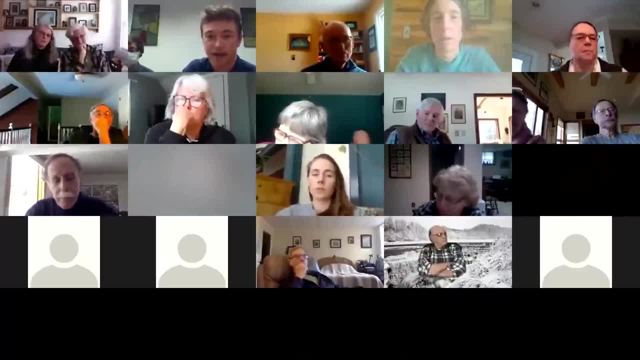 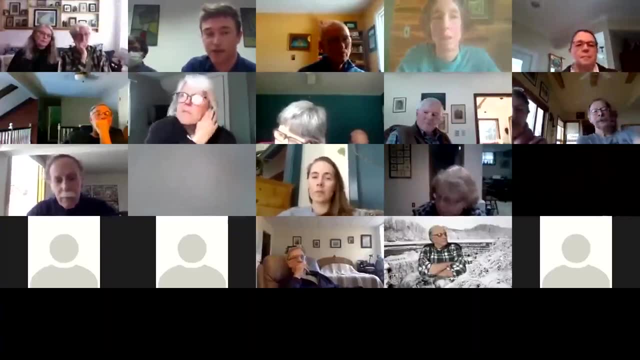 So no swimming within 24 hours of the water. They wait 24 hours after the last sighting of the bloom and then they collect a sample and test it for microcystin to make sure it's below that four microgram per liter limit. 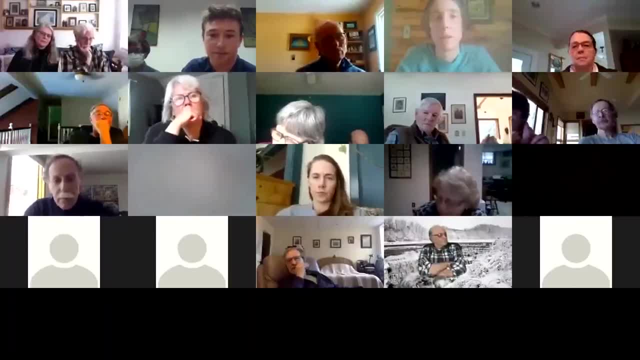 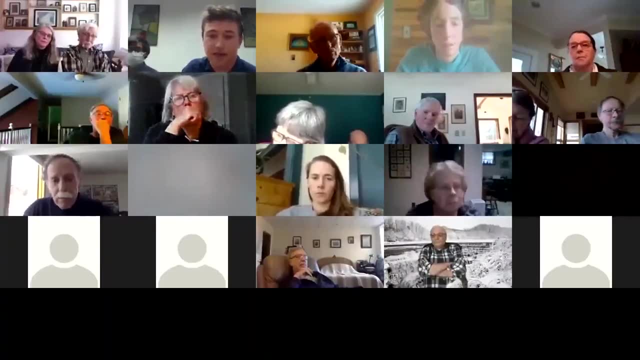 And then, if it is, then they reopen the beach for swimming. So I guess what I would say? you know it's always never. you know, go swimming when there's obvious signs of a bloom, And you know, following their lead, a good rule of thumb, maybe you know, even waiting 24 hours. 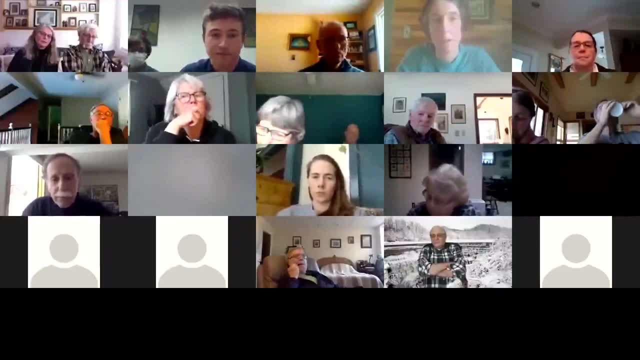 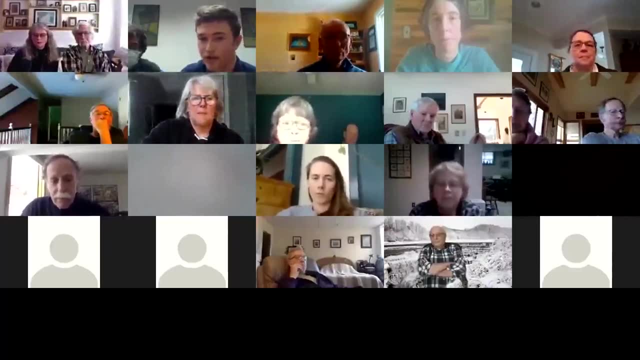 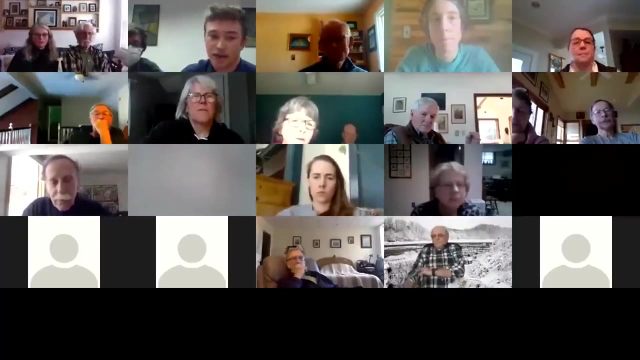 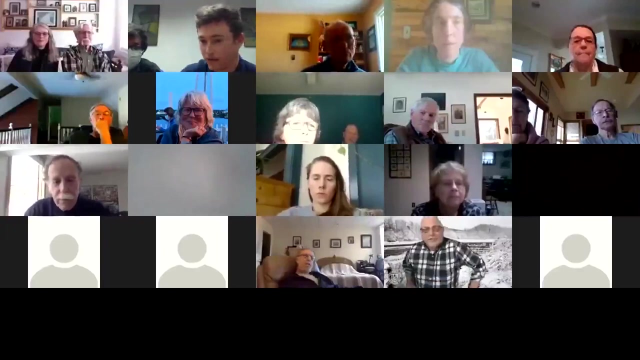 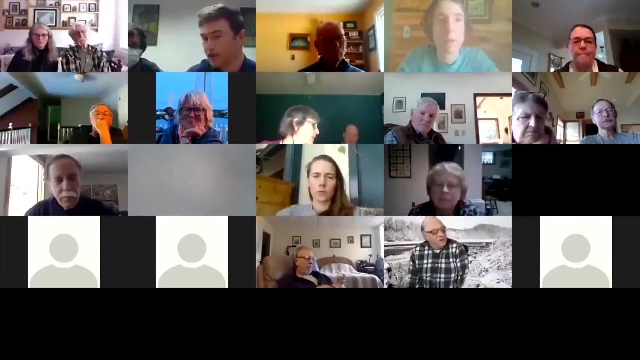 after a bloom has cleared. Thank you, It looks like John Abel has a question. John, if you'd like to unmute and ask, that would be great. Yeah, I have a kind of a naive question, But I was wondering. with climate change, we're seeing increases in CO2 concentrations in the air and probably in the water. 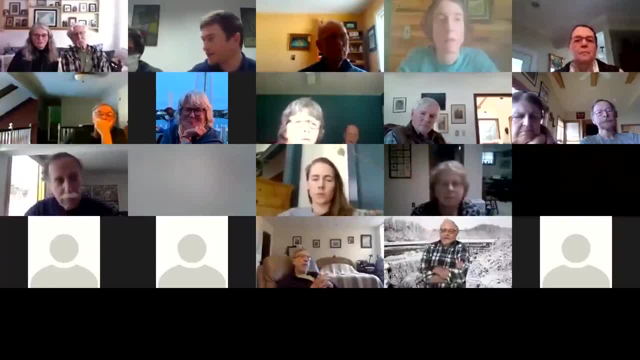 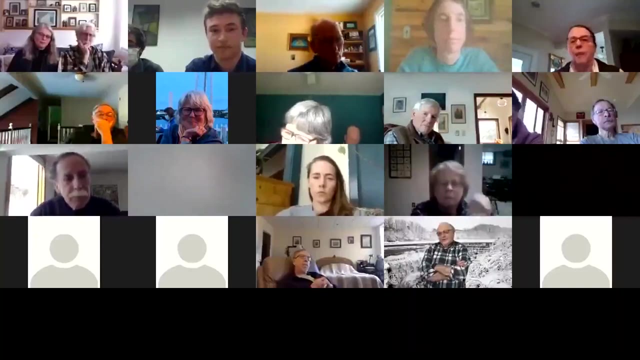 And I wondered whether the levels of CO2 might have any influence on blooming of the algae, in the sense that they consume it and convert it to oxygen. So it is. It's the input, the photosynthesis. So I don't know whether anyone has. 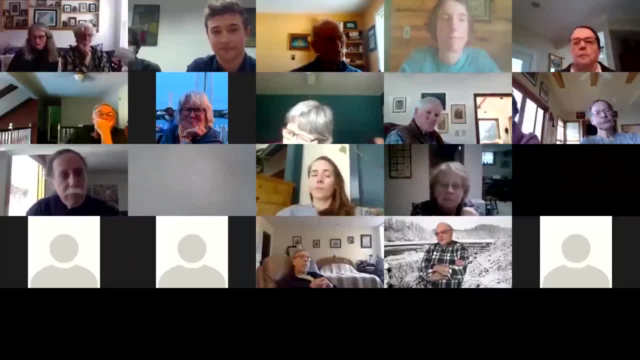 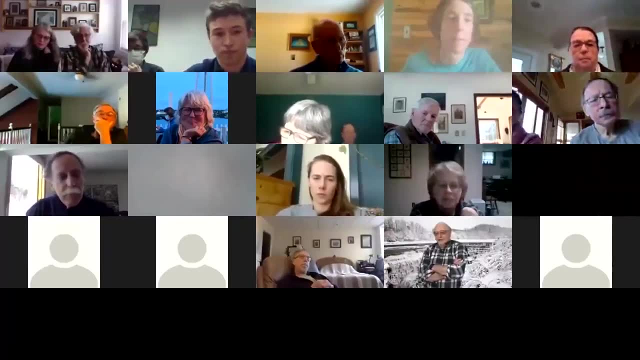 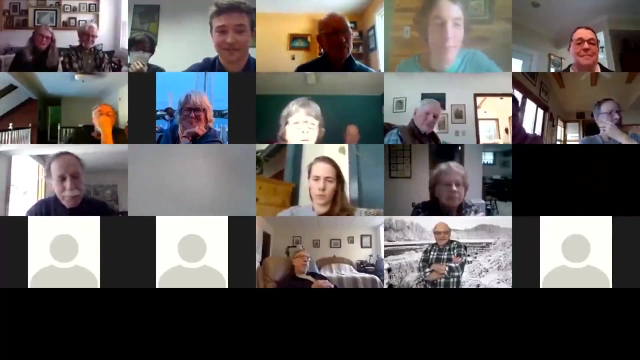 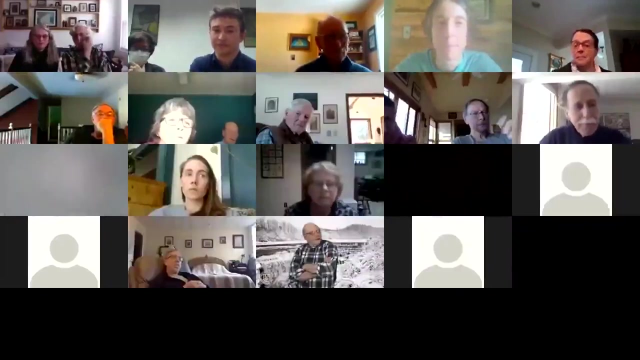 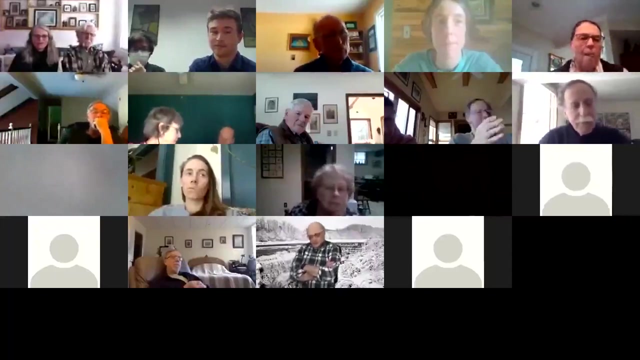 thought about that or ruled it out, or whether the levels of concentration are so unvariable that it's not a factor. Sounds like a good project. You up for it? That's an interesting question. I wondered, for example, whether in midsummer, when the trees are very busy photosynthesizing and that they're competing for the CO2, and in the fall, when they're declining, that maybe the CO2 concentrations go up because there's less competition for it. 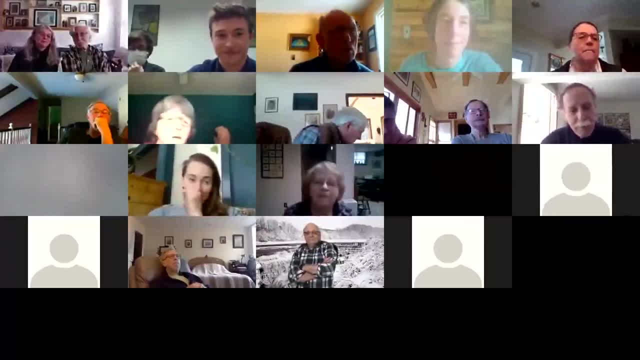 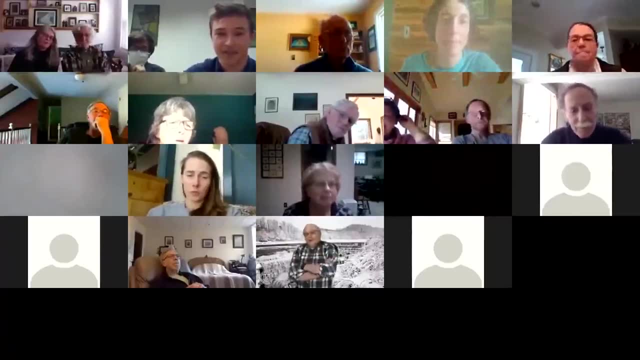 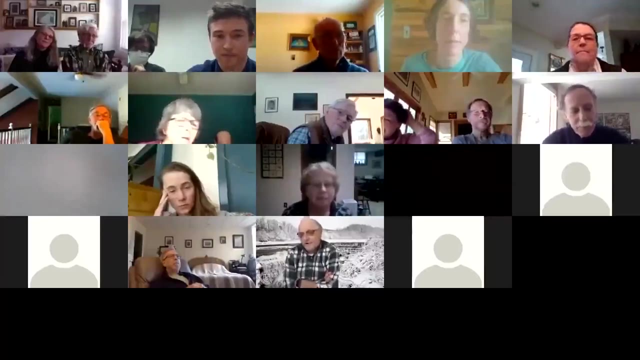 That's a difficult one to answer, Yeah, but certainly something that I think we should put some attention towards. Yeah, I think it relates to a larger question that some of us have, who are harriers, as to whether there should be other things that we're measuring when we sample, such as water temperature. 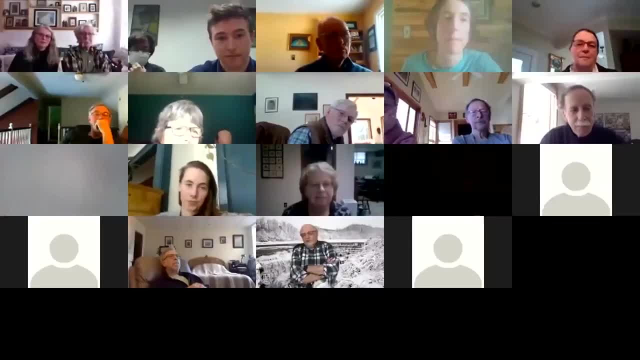 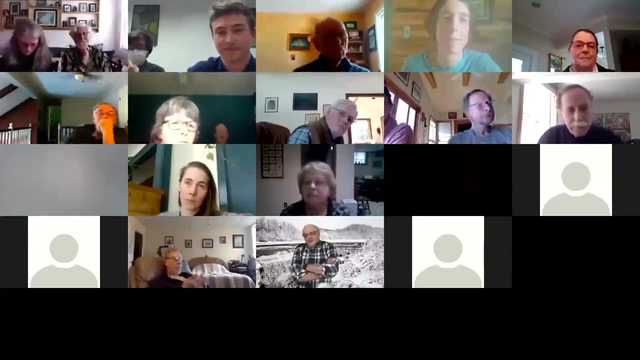 and things like that. I don't think the There's easy ways to monitor CO2 concentration, but you know, we have this wonderful experiment going on with lots of input, and yet we may be missing some important parts of the data, is my thought. 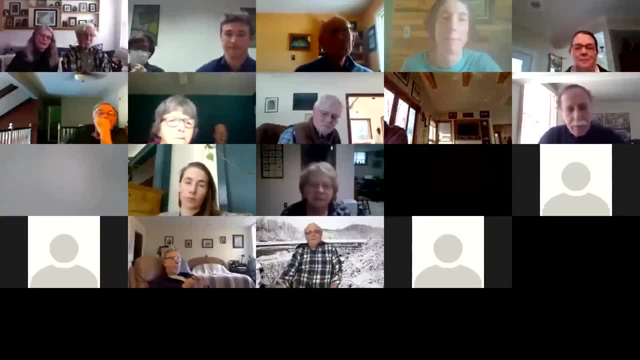 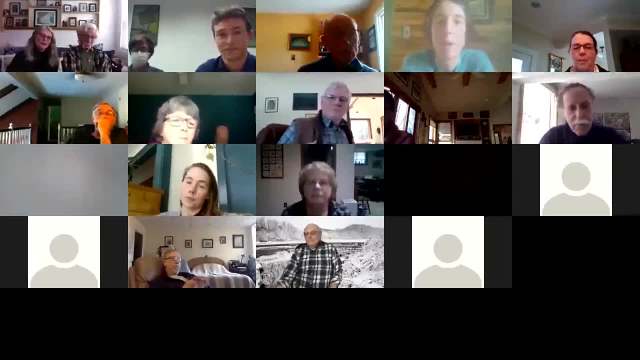 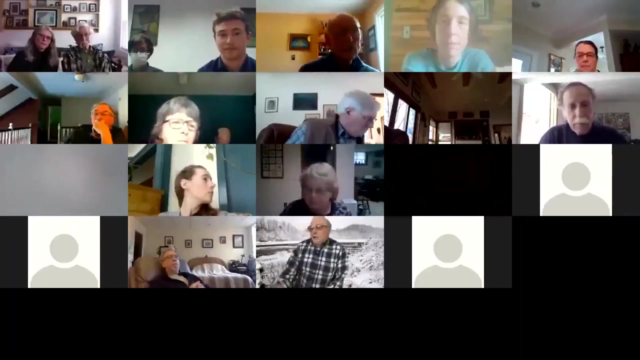 Yeah, John, we've often talked in our lab at CSI about measuring temperature, also about measuring nutrients in blooms. Nutrients are, that's, you know, really really tough to do accurately or meaningfully because the algae or the cyanobacteria themselves 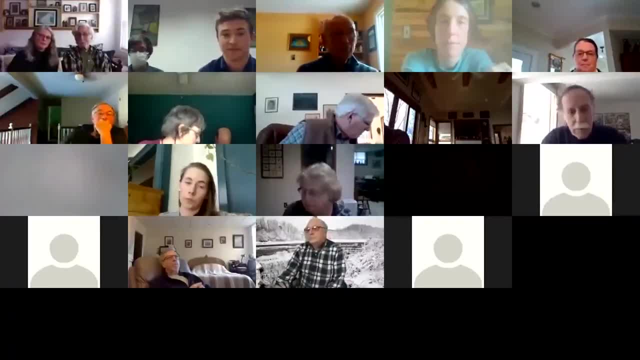 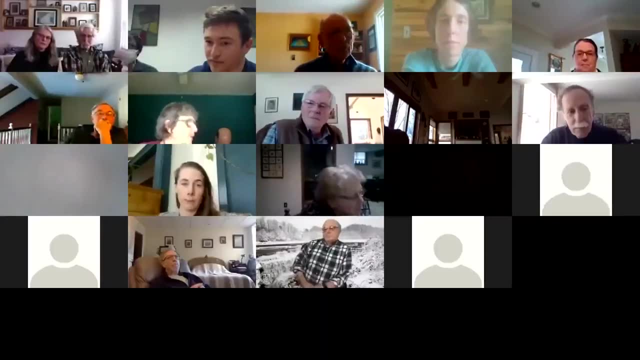 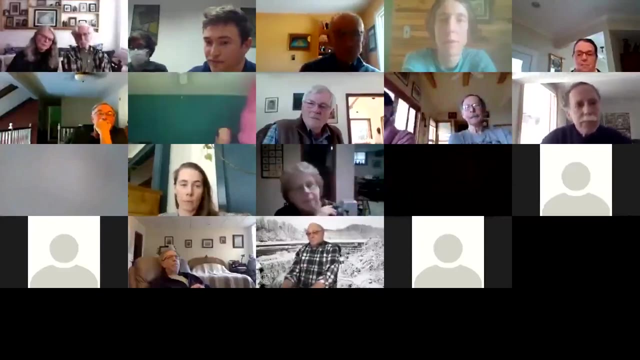 contain nutrients. So you know when you. how do you separate the nutrients in the ambient water In a bloom from the nutrients in the cyanobacteria, which have begun to die and release nutrients by the time they're collected and brought to the lab? 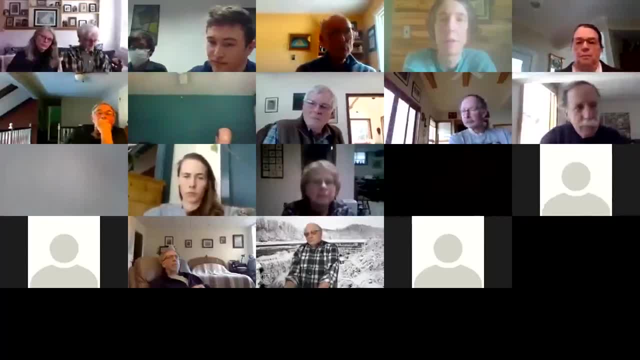 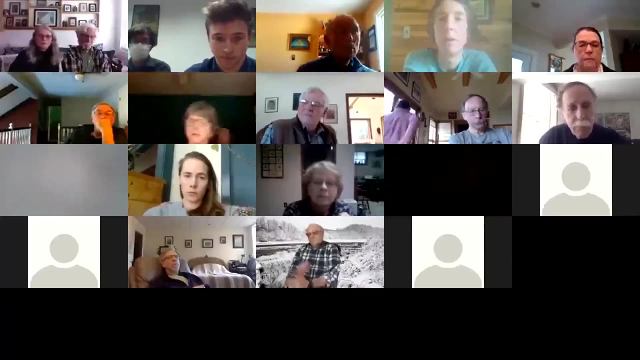 and certainly after they're processed in the lab. So so that's a so nutrient analysis of blooms. I think is is is tricky. As far as temperature goes, yes, that's a much more accessible parameter, I think the nutrients 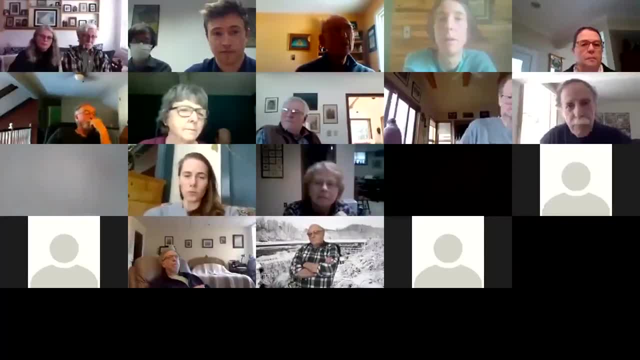 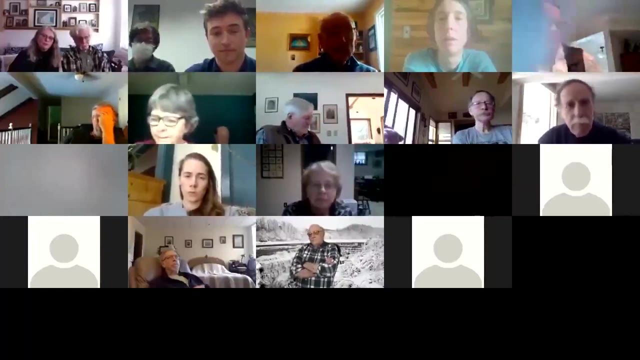 But again, to do that meaningfully, I mean you'd have to measure, we'd have to devise a protocol for temperature measurement that is reproducible among you- know all the volunteers- and have thermometers that will presumably give accurate measurements. I don't know. 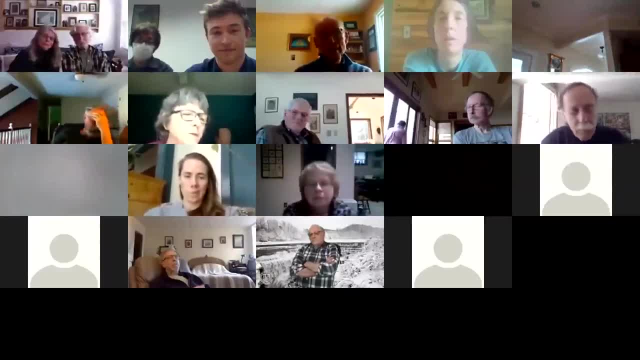 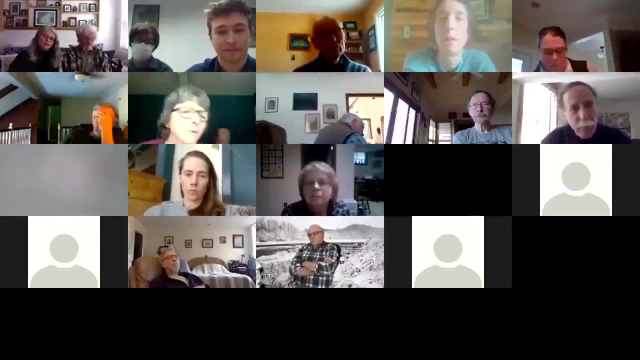 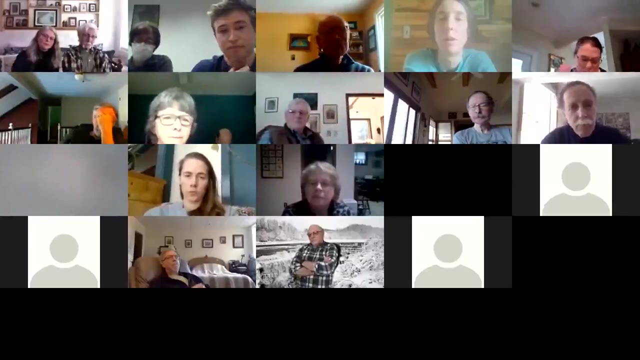 within tenths of a degree perhaps. That I'm not sure that's necessary, but it but you'd think that some of the small temperature fluctuations might be important, And one possibility that we've talked about is having a continuous temperature logger, let's say, at at one location, on one dock, or or a couple of docks. 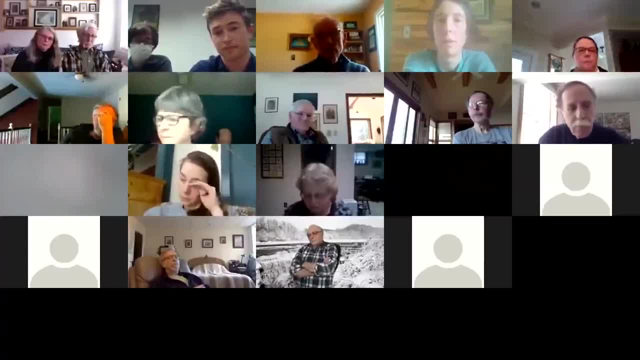 I believe they're doing that over on Seneca Lake. I don't know what the results are, Maybe somebody else knows- but they are doing something like that in their HATS program on Seneca Lake. So those are. Those are really good questions, really good thoughts. 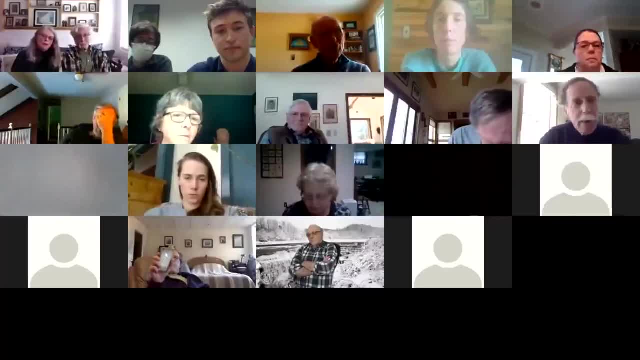 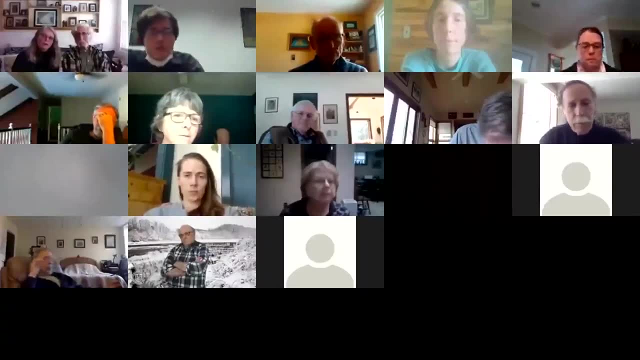 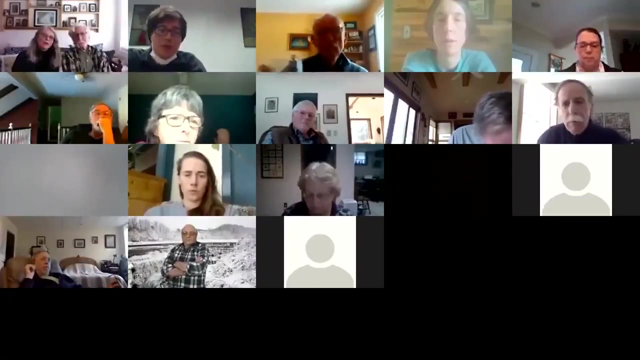 It's just but. but it's hard to do, you know hard to do. well, And just to piggyback off of Steve's comments, you know most of us are interested in the conditions leading up to a balloon, which you know as we. 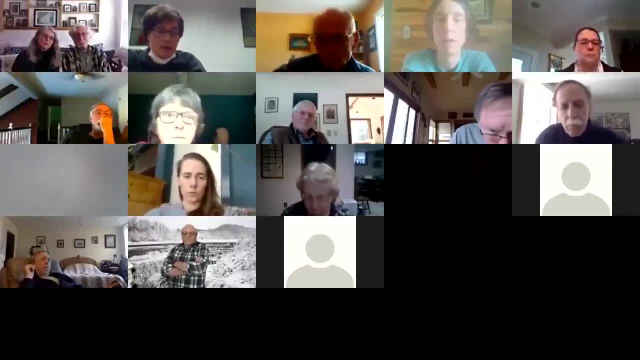 all know these things are really difficult to forecast: where they're going to, where they're going to occur. So that's, that's just another piece of the puzzle. So that's, that's just another piece of the puzzle. So that's, that's just another piece of the puzzle. 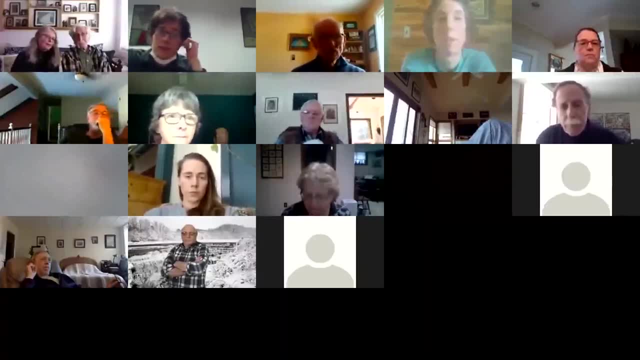 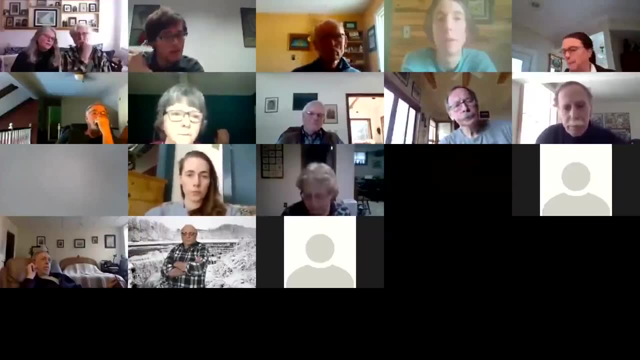 I guess you know we could look at, we could get data from. you know the like, the, the matrix that the blooms are occurring in. but I think a lot of us are interested more in like, what's the conditions that lead up to this population. 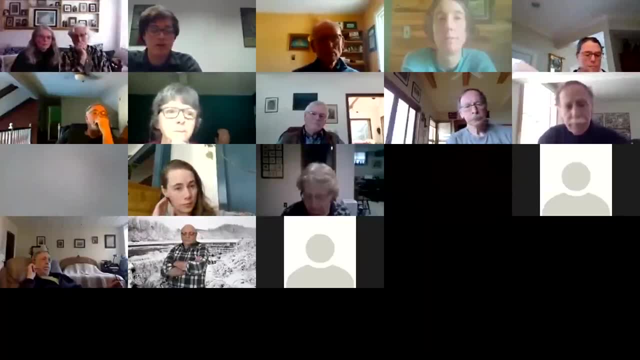 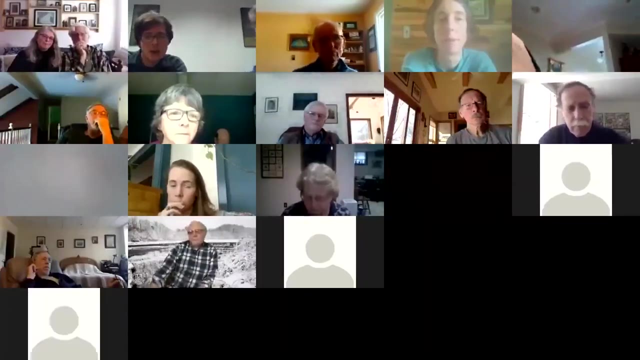 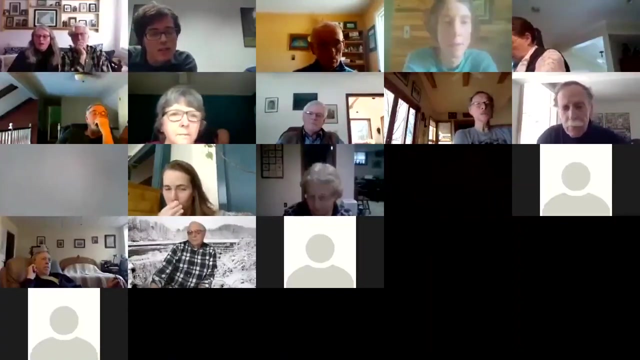 explosion that occurs and yeah, it's just really hard to logistically very hard to do. so Yeah, Um, yeah, should we move on to the next question? Sure, Um, can, can you hear me? Uh, we're going to move on to hello. uh, no, no, it's Hey, we can hear you. 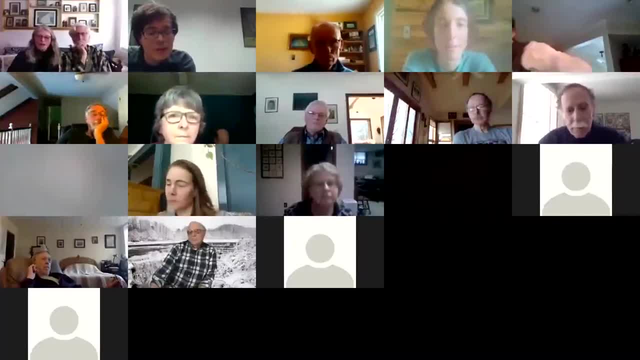 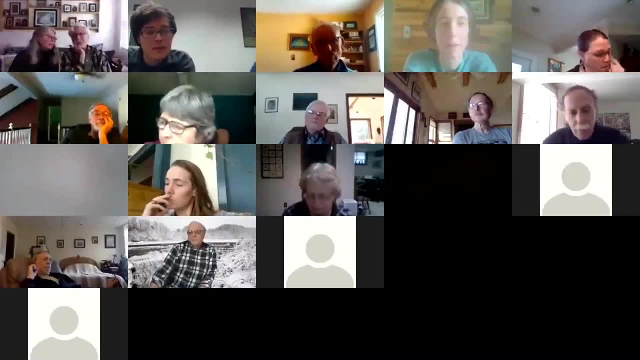 Hey, so sorry, I just uh butted in. uh, I'm, I'm Alex, a senior analyst at CSI. I just uh, can I quickly uh comment on the uh CO2 question? Sure, 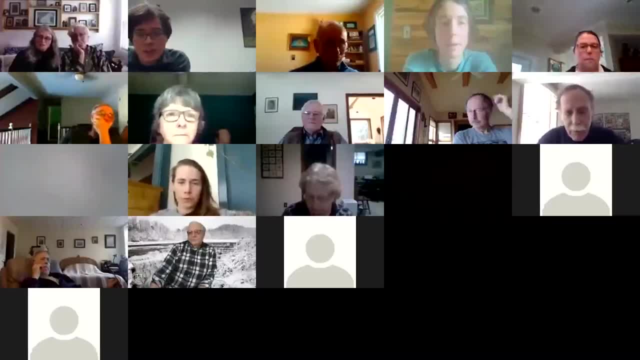 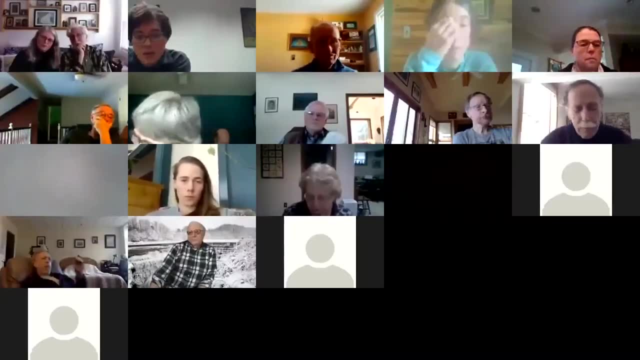 Sure Yeah, Go for it. Yeah, So uh, if we think of the kind of uh input And output of of CO2, I mean I mean in general, uh, uh, globally, uh, right, 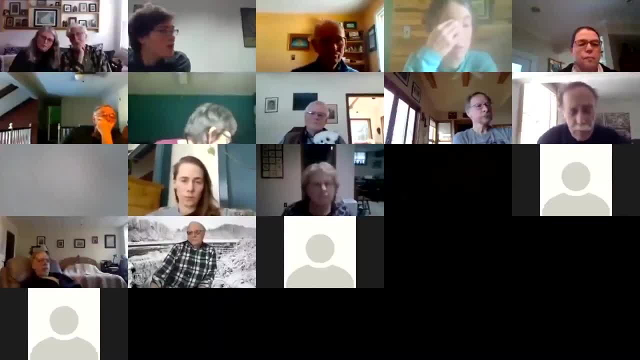 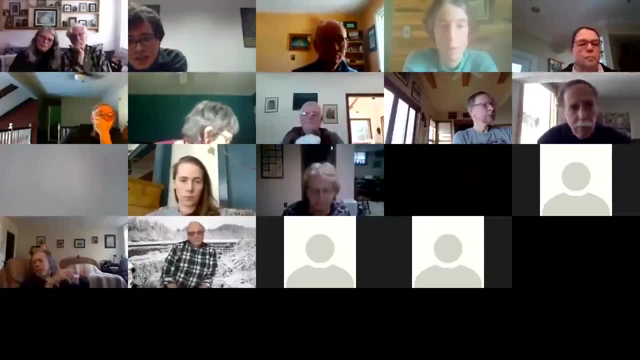 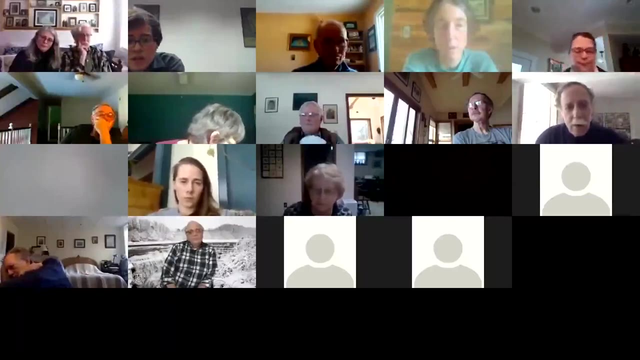 So we see an increase of CO2, uh, hence uh global warming. So um means that our input of CO2 is greater than uh. whatever the uh trees and cyanobacteria can kind of consume uh in terms of um, um, their uh uh. 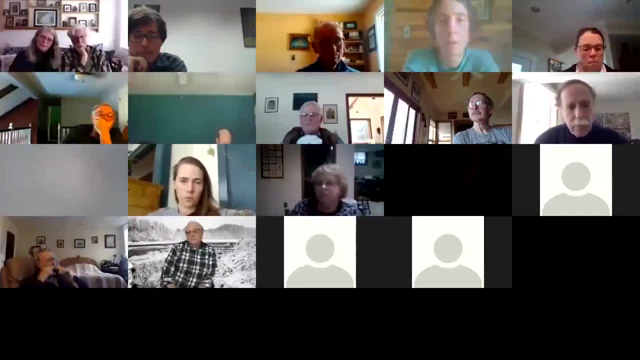 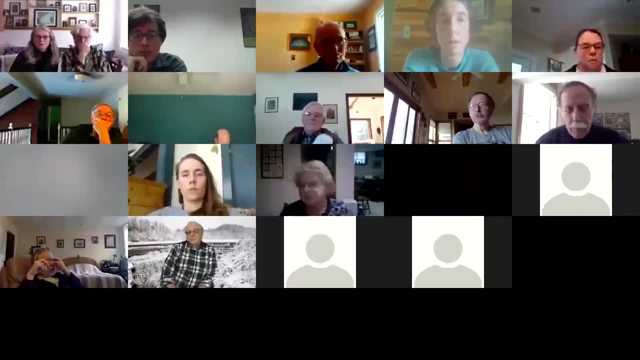 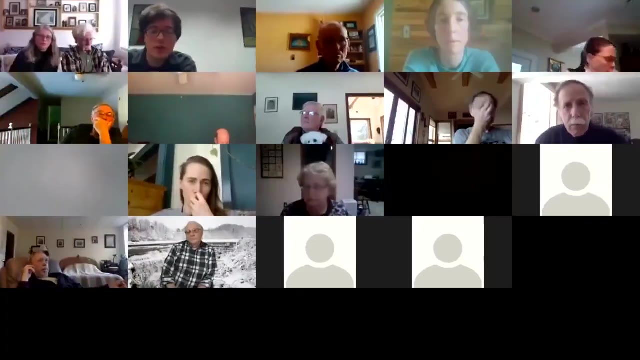 photosynthesis. So, uh, it would be probably, uh, uh, uh, unlikely that. uh, CO2 is a limiting factor In that sense. Great Thanks for your input, Alex. Um, there's two questions here. 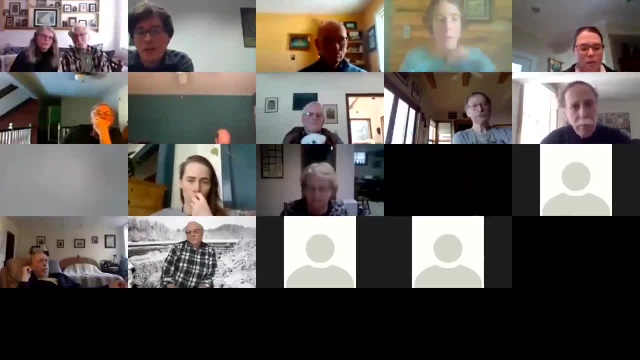 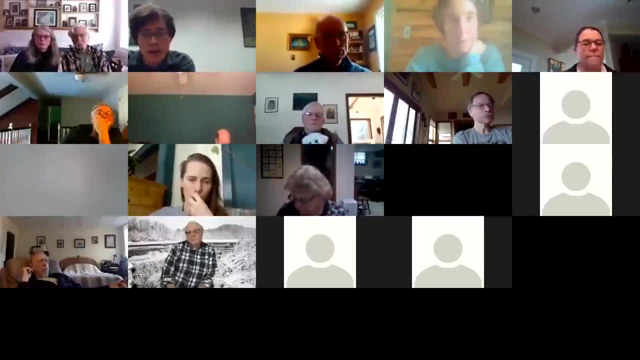 Maybe, uh, Steve, if you want to take a stab at these. um uh, someone asked: are you sampling for anything besides algae, such as other bacteria and E coli, And is there an increase in blooms near outfalls, or is there no correlation? 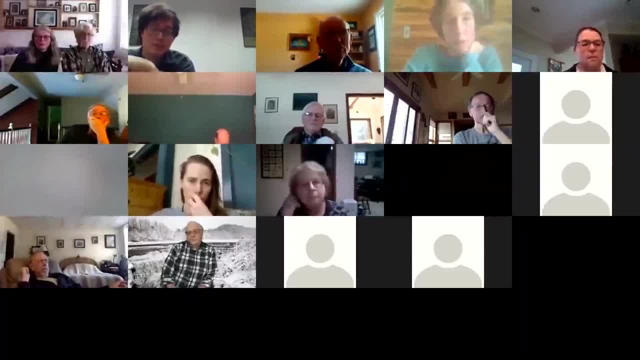 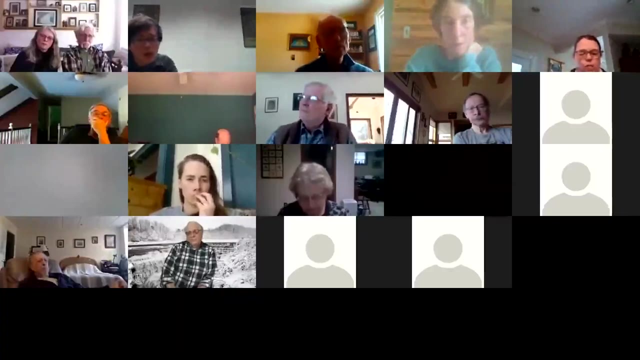 Um, so are we sampling and testing for other uh microorganisms? Uh well, uh. first Adriana, of course, is surveying micro phytoplankton, all different types of um, eukaryotic and prokaryotic uh phytoplankton. 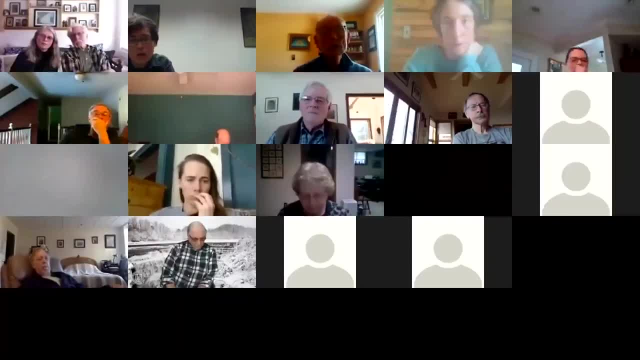 Uh, we do uh test for E coli. We uh team up with Discover Cayuga Lake and go out on uh two or three eco cruises, monitoring cruises uh each summer, And one of the parameters that we measure at at uh seven different locations on the. 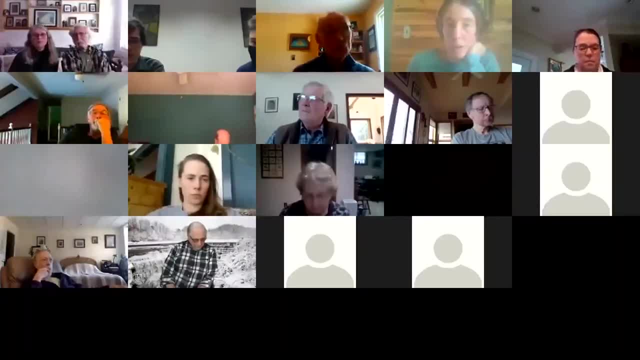 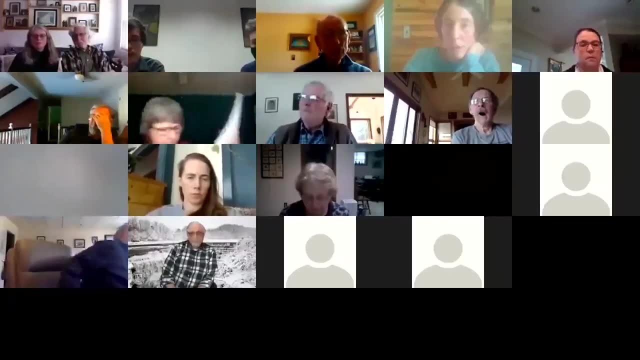 lake where we uh sample is E coli. So yes, we are measuring E coli on the lake and the levels are quite low. Uh 235 colonies per a hundred ML is the limit for uh recreational swimming uh contact. 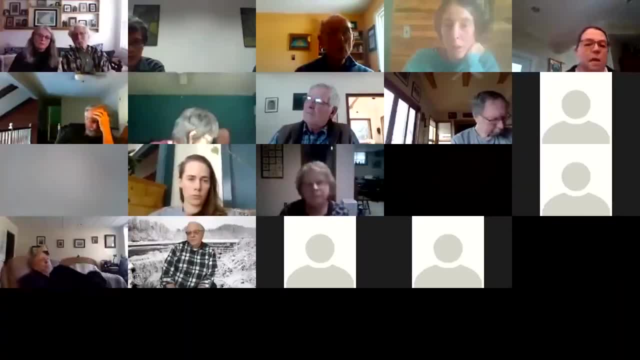 recreation. And uh, as far as I know, all of the concentrations on Cayuga Lake are well below that limit. Um so, uh, that's the answer to that question. What was the rest of the question, please? Or the other question, the second one? 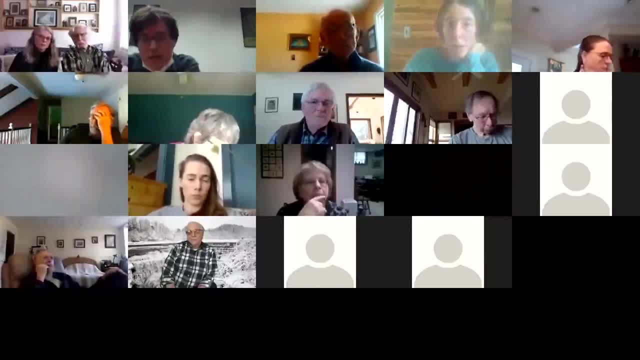 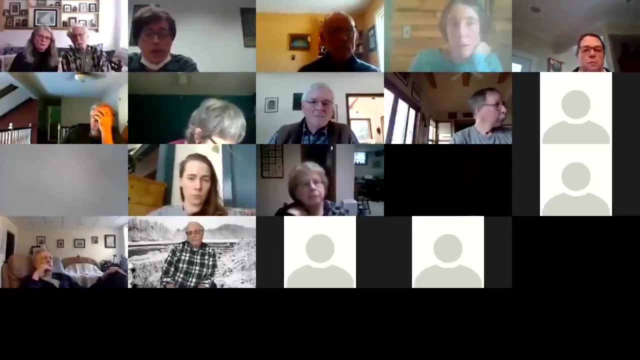 The other half of the question, um, or I guess different question- is: is there an increase in blooms near outfalls? Uh, or is there no correlation? I'm not aware of any correlation. Uh, outfalls, you'd probably mean outfalls with wastewater treatment plants. 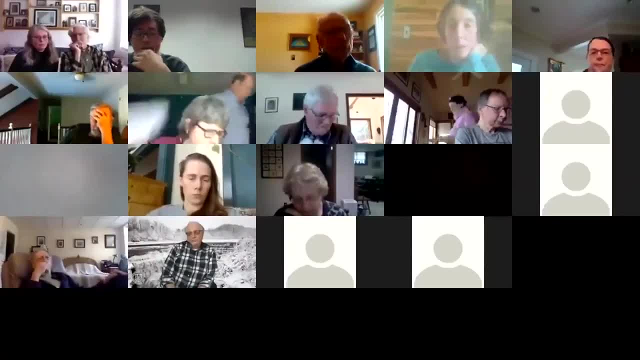 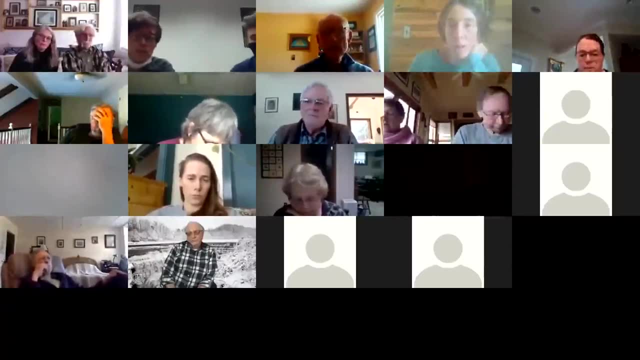 Um and uh. actually, our HABs- heritors- would probably be the best ones to answer that, because they're the ones that you know patrol uh the shoreline and they know where the wastewater treatment plants are, the outfalls uh, generally speaking. 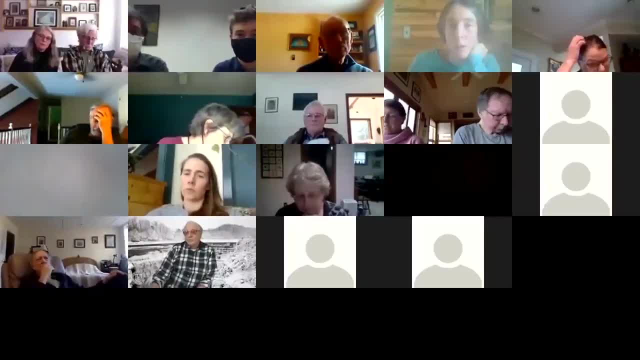 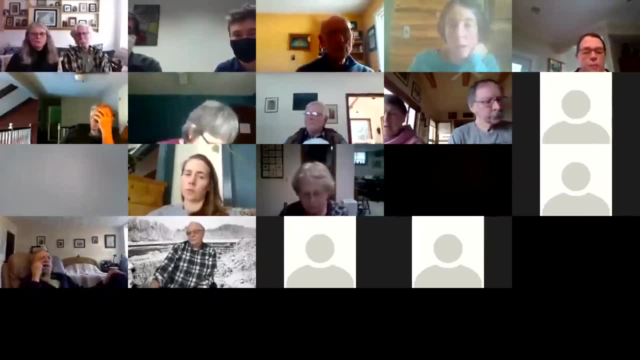 Um, just a quick comment. There are two wastewater treatment plants. One is the? uh, the outfalls at the south end of Cayuga Lake. The other one is the outfalls at the south end of Cayuga Lake, Both of them in the basically the center, the middle of the uh, of the shallow southern shelf. 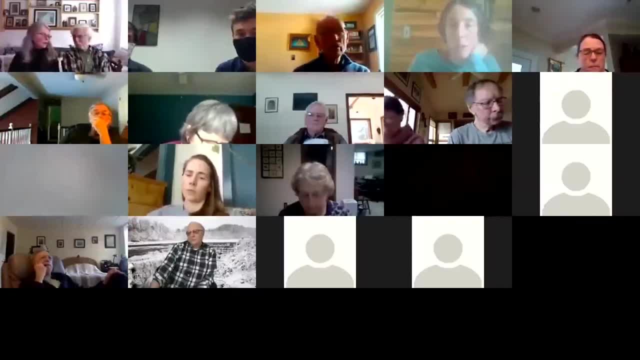 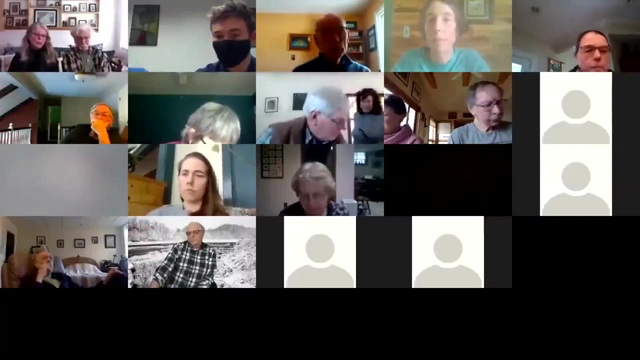 As far again, we do not test uh as a pool sample for um HABs in open water in Cayuga Lake. Uh. that said, I'm not aware of blooms uh above or near those outfalls. uh or uh above or near the uh Lake. San Diego. 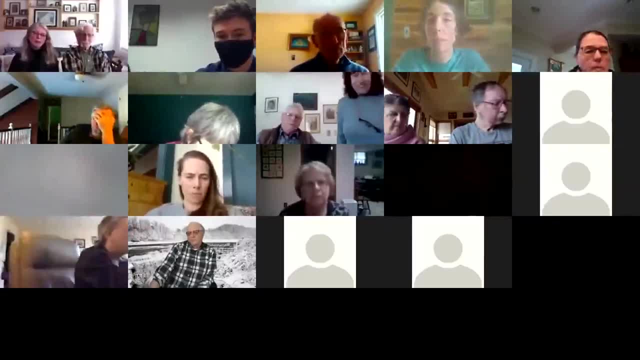 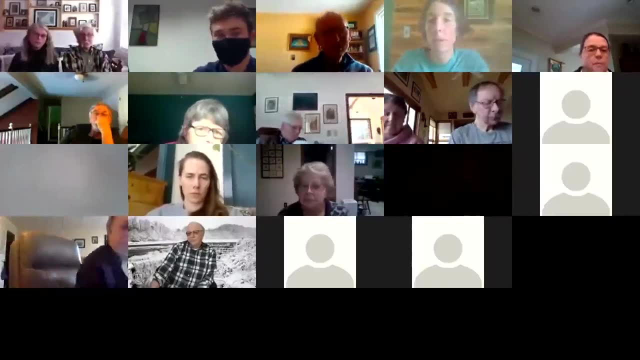 Uh and uh, I don't know if you can hear me. Uh, I don't know if you can hear me. Uh, I don't know if you can hear me. source: cooling outfall, which we also monitor. But, HABS, Harriers, what say you? You're the ones. 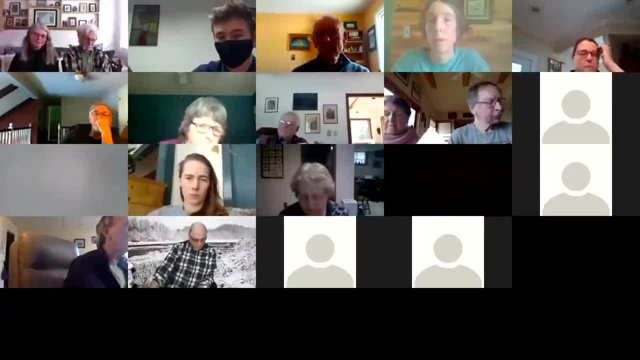 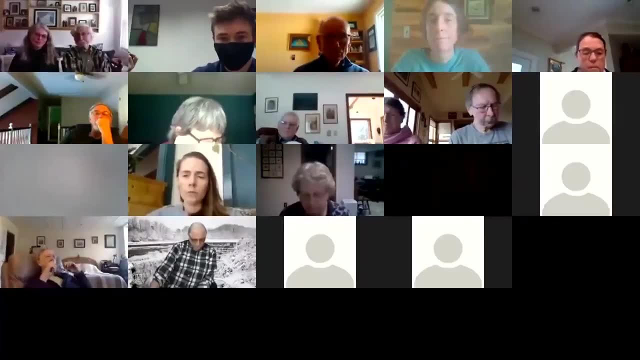 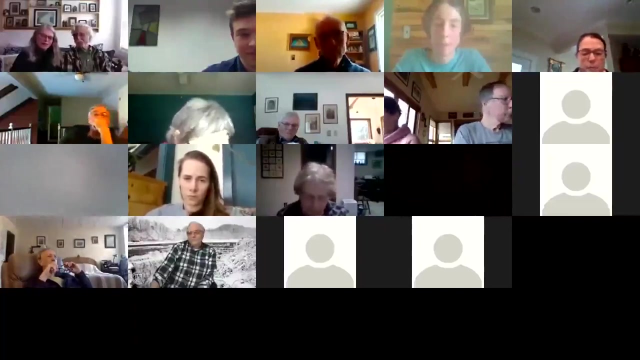 that are patrolling the lake. You have firsthand observations. Hard to say: We don't have any outfalls here. At some point I guess all of these little homes had their own septic systems, but we converted to public water and sewer over five years ago. I guess We've only been here for 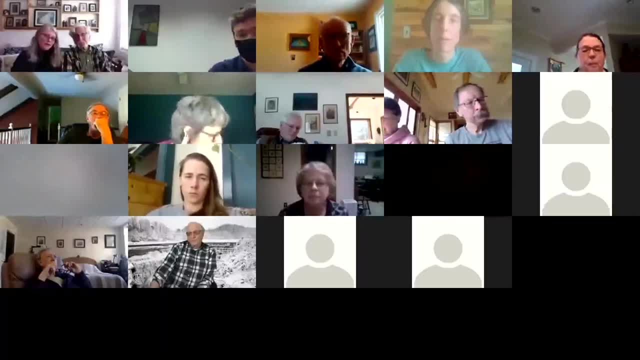 about five years, by the way, And we've seen it seems like a dramatic increase in the HABS in our experience. Of course, we're more closely monitoring it too. Anyway, I won't be able to comment about outfalls. 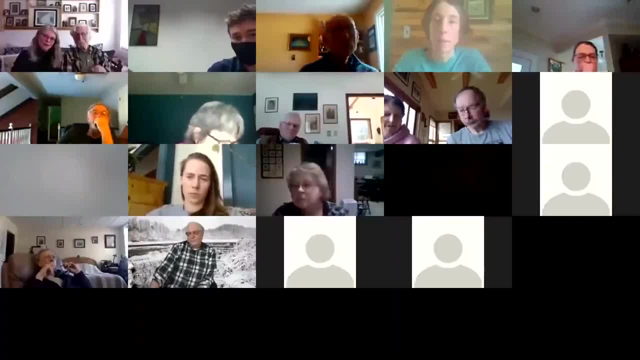 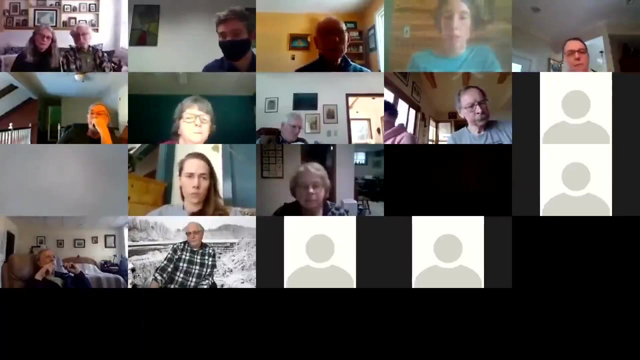 Right. And as far as wastewater from on-site septic systems, we do team up with the West Shore Neighborhood Association and they collect samples several times a year at about 16 or 18 locations along the west shore, southwest shore of Cayuga Lake, from Ithaca up to almost the Seneca River And they collect samples several times a year at about 16 or 18 locations along the southwest shore of Cayuga Lake, from Ithaca up to almost the Seneca River County line, or maybe a little beyond. The concentrations of E coli at those locations?